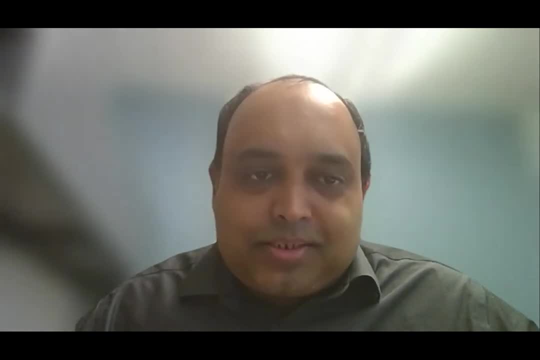 in the physical world. Professor Ramani has many distinctions, but maybe read a few of those. In the summer of 2016, he was a visiting professor at Oxford University Institute of Mathematical Sciences. In 2008, he was a visiting professor at Stanford University Computer. 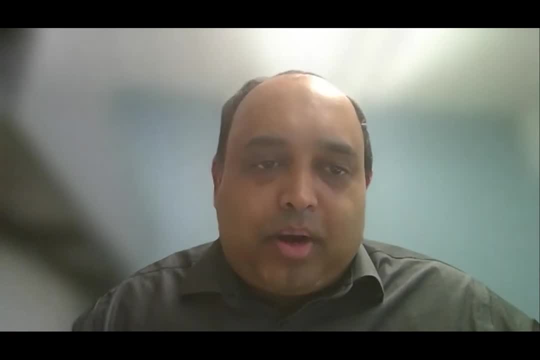 Sciences and also a research fellow at Park, formerly Xerox PARC, Professor Ramani also. He also served as the editorial board of several journals, including the Journal of Contemporary Design and the ACME Journal of Mechanical Design. Professor Ramani, as you could see, is certainly a prolific researcher, has already mentored 35 BG students- currently probably have another dogen or so ongoing- and also a prolific inventor. 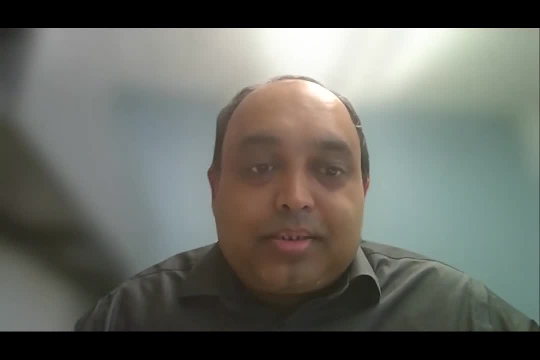 Having to his record more than 25 patents, some of them have been licensed. Professor Ramani received his PhD from Stanford University, a master's from Ohio State and an undergrad from Indian Institute of Technology, Madras, all in mechanical engineering. 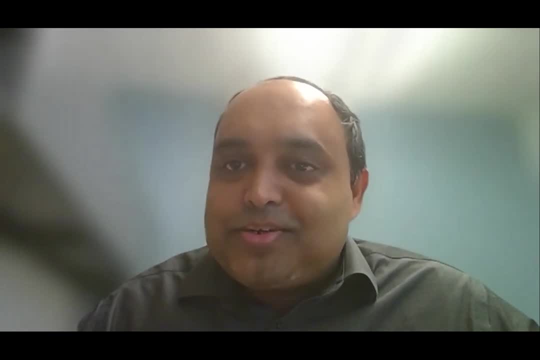 Here. I would like to give a prompt here. Professor Ramani has something very interesting to talk about, hopefully, when he introduces our two speakers, in terms of academic genealogy and how he's connected somehow with these two speakers. Again, I would like to mention that Professor Ramani doesn't say this, but I would like to mention here as a colleague. 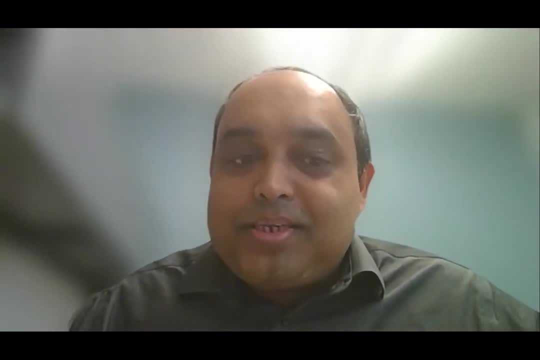 Professor Ramani also has this very rare distinction of being at Purdue of being recognized by both a research excellence award and also a commercialization award, which is rare. So again, congratulations, Professor Ramani. He doesn't say that, but I wanted to mention that. 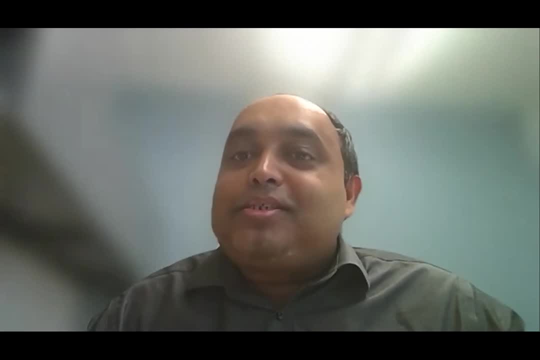 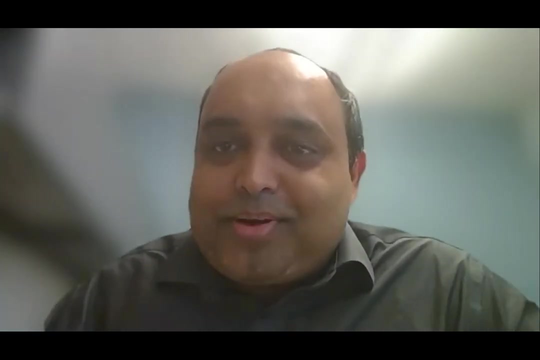 Professor Ramani has been a prolific ideator and a convergent thinker and also he has developed the award-winning toy design. With that I'll conclude here, but on a very personal note regarding Professor Ramani as a colleague, that the award about convergence in a very true and broad sense. I learned about that. 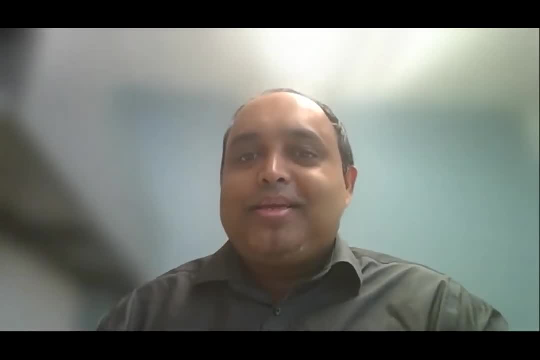 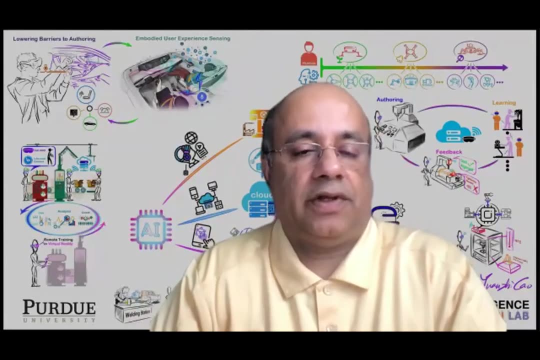 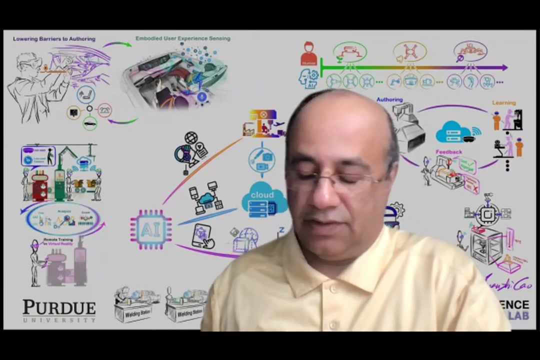 So I'll conclude with that. a convergent thinker and ideator, Professor Ramani, the session is yours. Thank you. Thanks, Partha, as well as yourself and Sid, for having started this multi-university session. It is there to stay, even after the fall of COVID. This is a great idea. 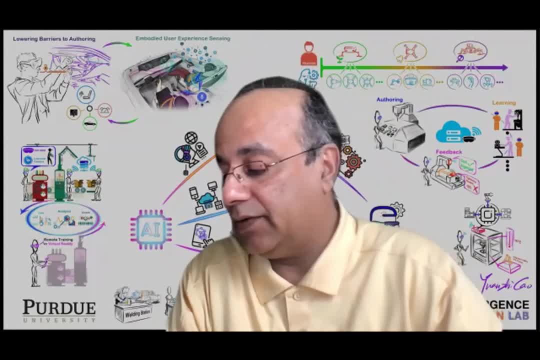 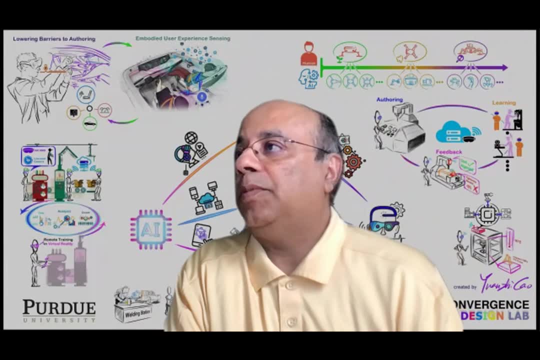 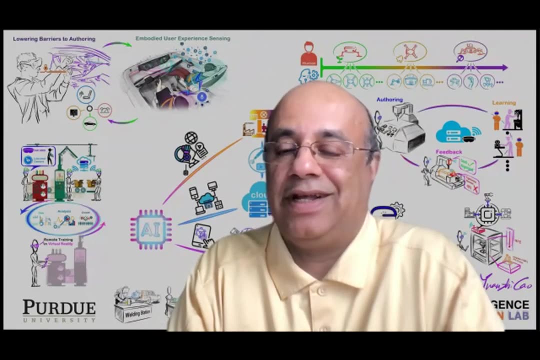 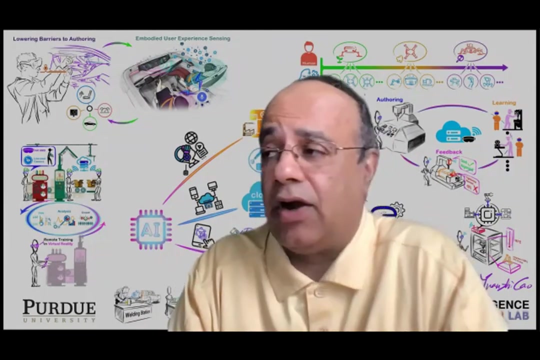 So thank you for, and all the organizers on, the effort behind this series. So I wanted to first get into introducing my colleagues, both Patrick as well as Laura, And curiously, I'm just connected to both of them in multiple ways. First of all, I started at Ohio State working on HEXAPOD, and Patrick's advisor, Oren, was working on a large DARPA project. 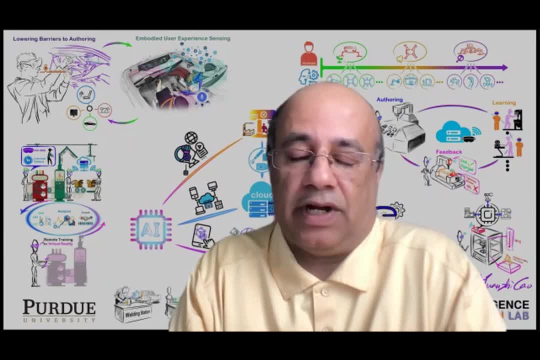 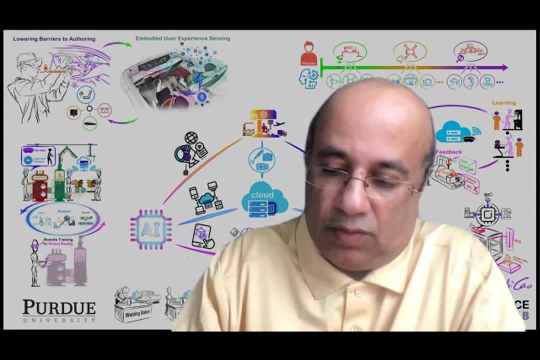 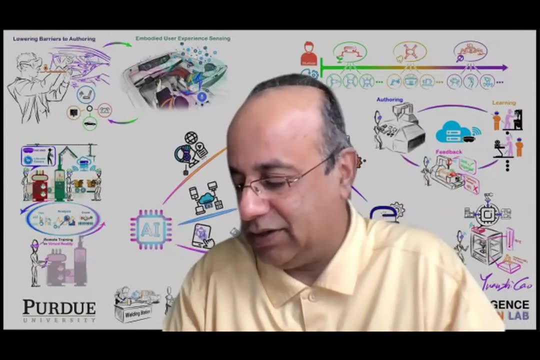 And of course, I like the Buckeyes as well And later on ended up working with Professor Mark Kutkowski at Stanford and who, it turns out, also advised Allison, who's a friend of mine- So different connections to both of them- And I started my career in robotics. 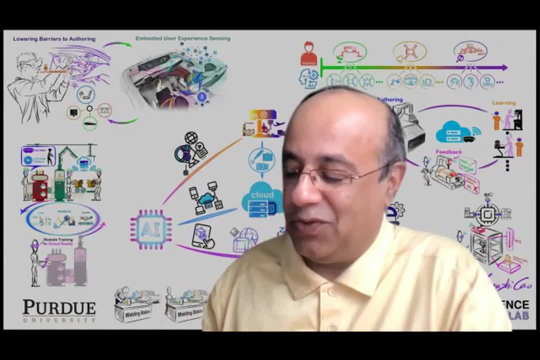 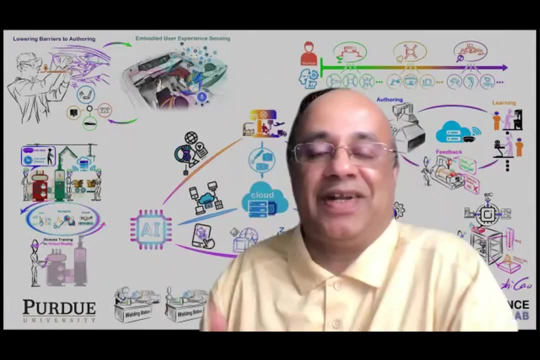 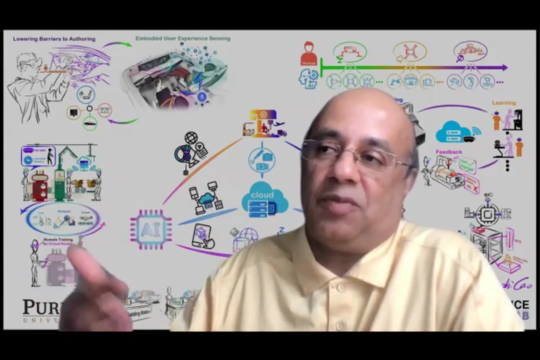 So with that, when I talked to them, I was so inspired, wanting to start becoming a student, with both of them, in fact- And trying to relearn how exoskeletons may work, How we can get rid of buttons, And I started thinking about the future of what soft robots can be. 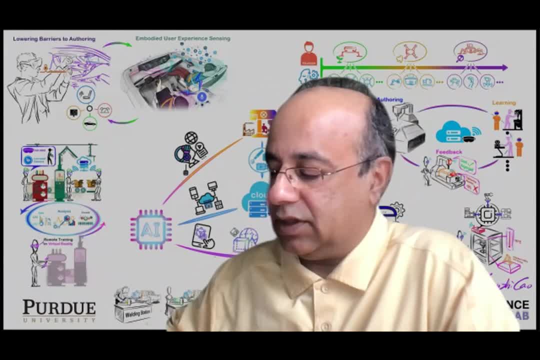 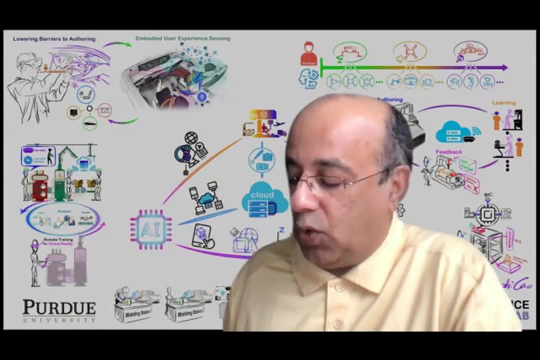 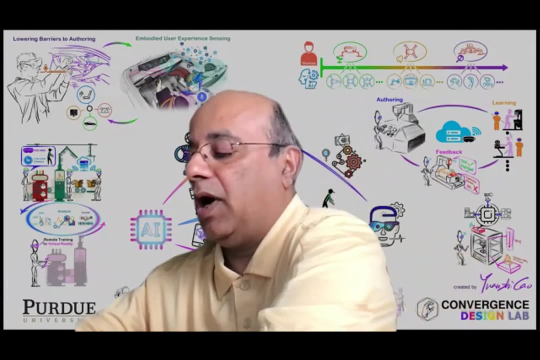 And pretty nice research done by both of them in abstraction of models, to intent detection, to what tasks are good for soft robots and how we can control exoskeleton and make robots more adaptive. But of course, robots these days are not even close to the ones that I started with, which are mostly armed robots. 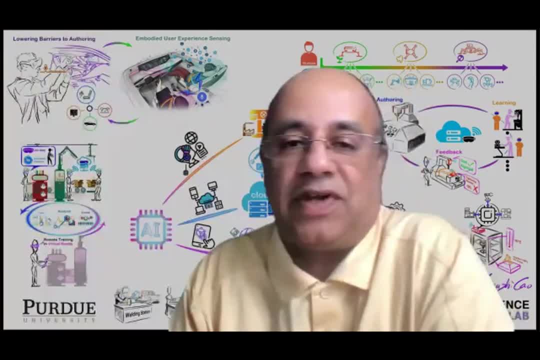 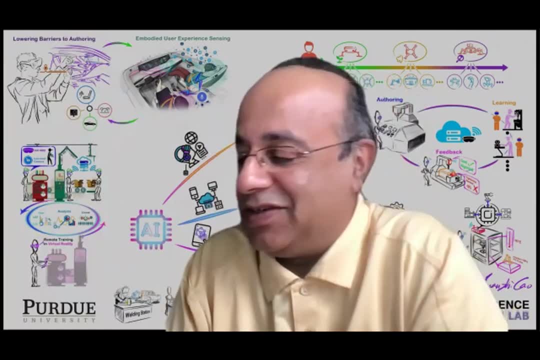 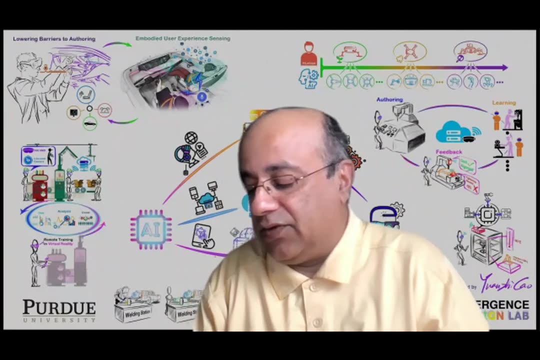 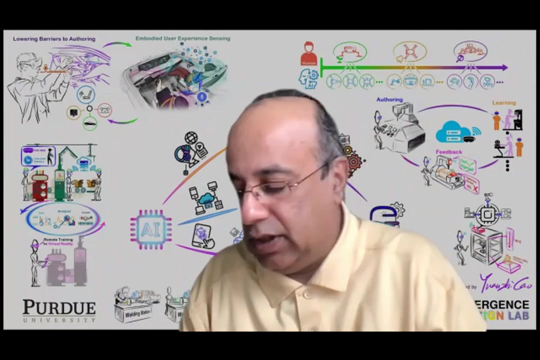 And they said in those days: robots are going to take over humans. And that story has come back again. Nothing wrong with it. It gives some of our researchers more funding. But also going in this direction, the theme that we are going to hear from both of them is co-design, control, design, action planning and so on, where robots can become more robust in tough environments. 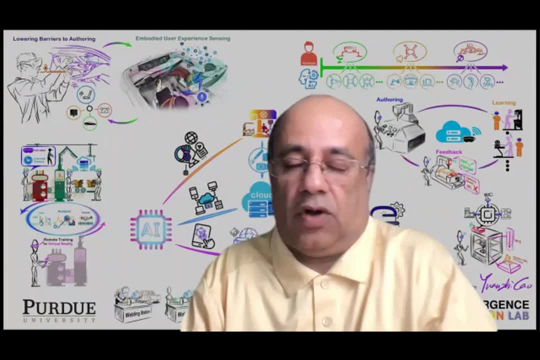 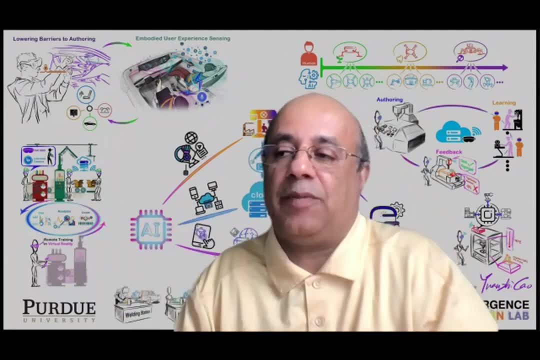 And in terms of Laura's talk, we're going to talk a little bit about that And, in terms of Laura's talk, we're going to hear a lot about, hopefully, geometric adaptations and meanings of kinematics and inverse kinematics- all that I studied in the 1980s. how that is changing completely in terms of how we can think of soft robots. 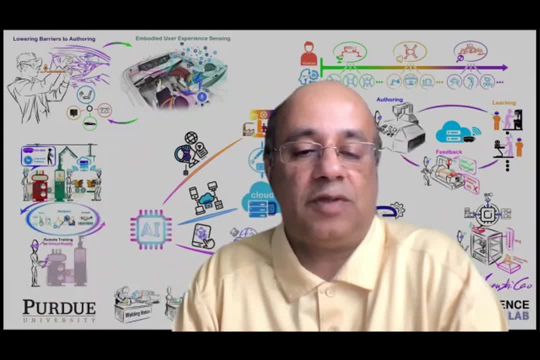 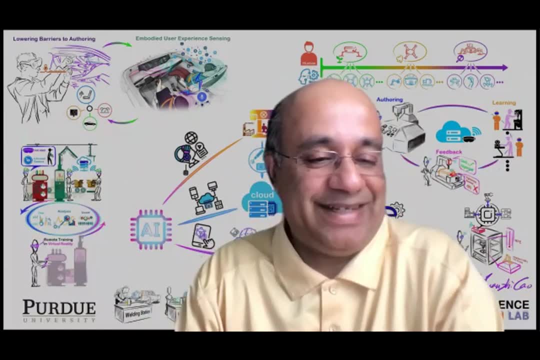 So with that, without taking any more time, we will start off with Patrick- the hard problems- And then we'll end up with soft problems that are hard. Okay, All right, Go ahead, Patrick. Thank you, Karthik. 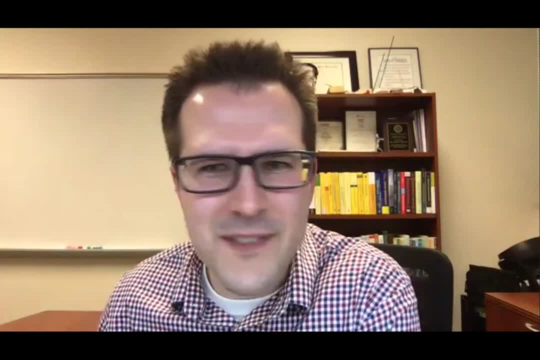 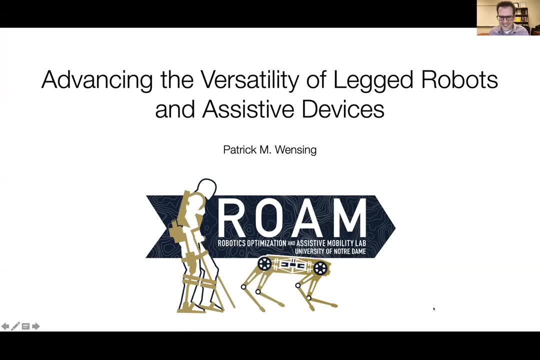 Greatly appreciate that. That was perhaps one of the most fun introductions that I've had. It's wonderful, Okay. So thank you again to the organizers for having me. It's a great honor to have this chance to tell you about some of the work in my group, the Robotics Optimization and the System Mobility Lab at the University of Notre Dame. 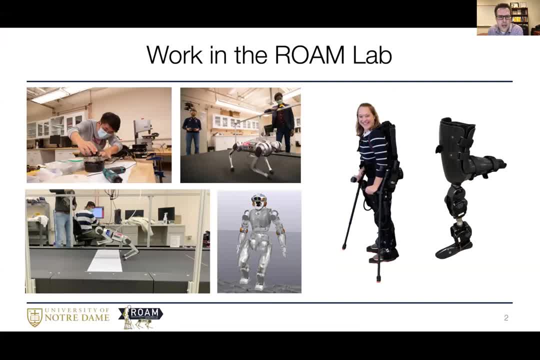 So work in my group is focused on advancing robotics. We're focused on advancing the mobility of legged robots, both in the form of quadrupeds and humanoid robots, as well as robots that we might wear on our bodies in the form of assistive exoskeletons or lower limb prostheses. 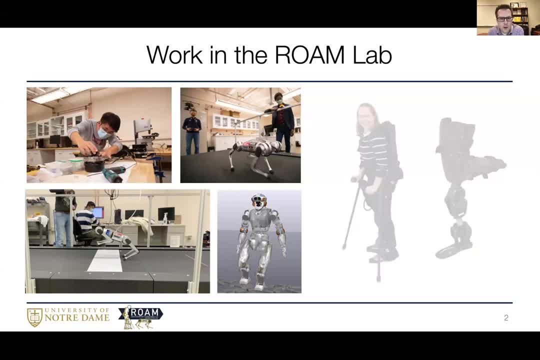 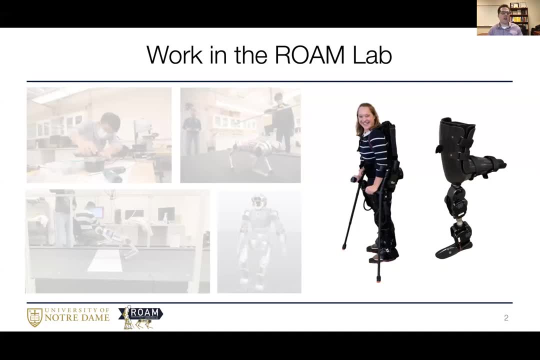 So on the left side, our goal is for these robots to be able to go anywhere on land, And on the right, our goal is to translate some of these advances so that people can go anywhere on land And then, after they've had an injury that might otherwise limit their mobility. 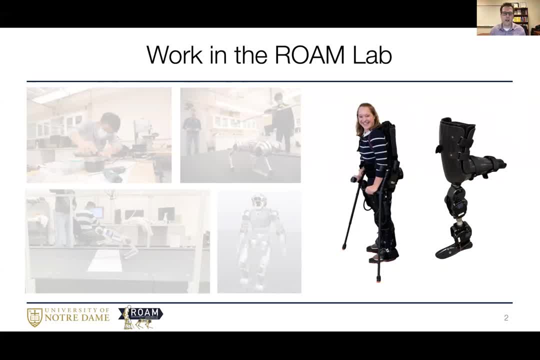 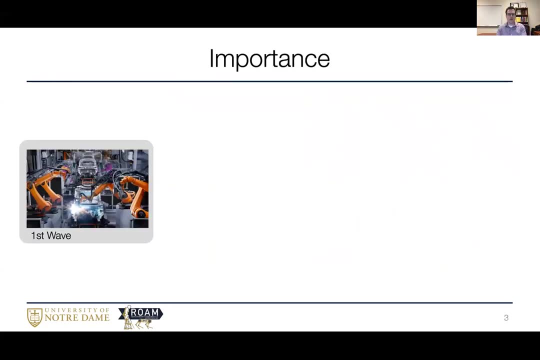 Now, aside from kind of both of these areas being united in the presence of legs, I think the challenges that are facing these systems are really representative of the ones that are kind of facing our next wave of robotics applications more broadly. So if we think about the first wave of robots- perhaps the robots that Karthik was mentioning at the beginning as the ones that he was working on at the beginning, 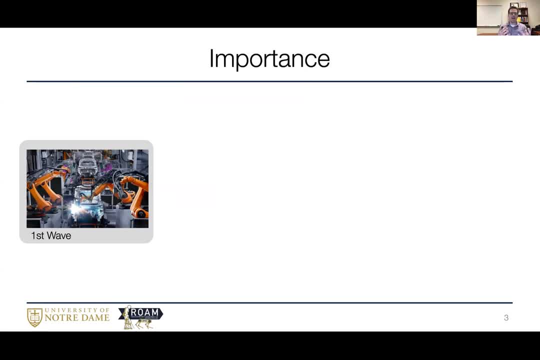 We were thinking of these robots that have made a really phenomenal impact on the industrial assembly line, where these robots are complicated to control, but we really don't want them to be around humans. They can be quite dangerous. We've seen robots, however, more recently kind of coming out into the real world. 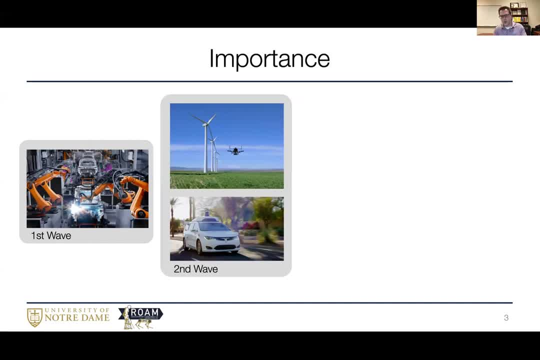 But most of the applications and what I would call the second wave of robotics have been very much, you know, look but don't touch by design. We have drones that are participating. We have drones that are participating in inspection and surveillance But, you know, hopefully not coming in contact with those objects, and very much likewise with autonomous vehicles. we don't want them to come in contact with humans. 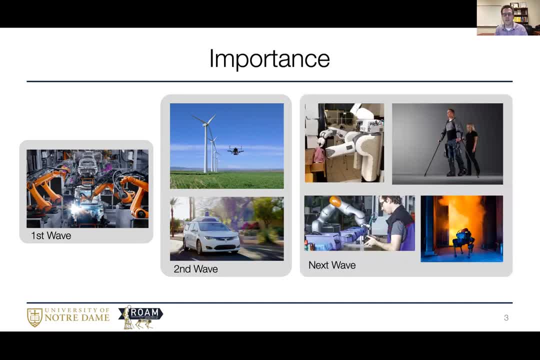 And this is very much in contrast with what I see is kind of the next wave of applications for our for robotics, where we want these systems to be kind of out in the world with and amongst us and helping to amplify and and restore our human capabilities. 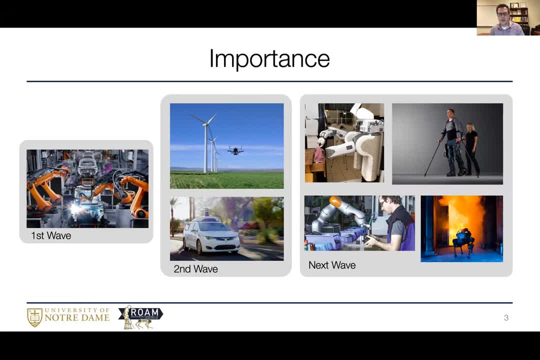 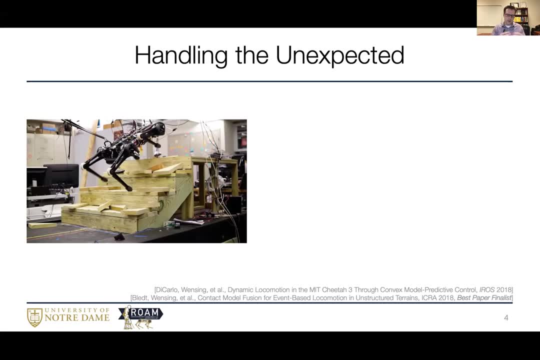 So, in terms of the challenges that I think We face there, See them as quite different, whether we're working with, you know, kind of autonomous systems or or ones that are interacting around humans. So we think first about autonomous legged robots. 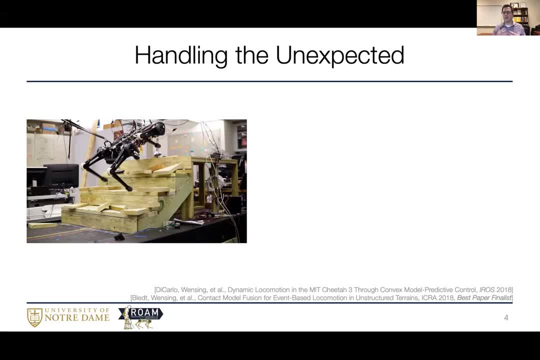 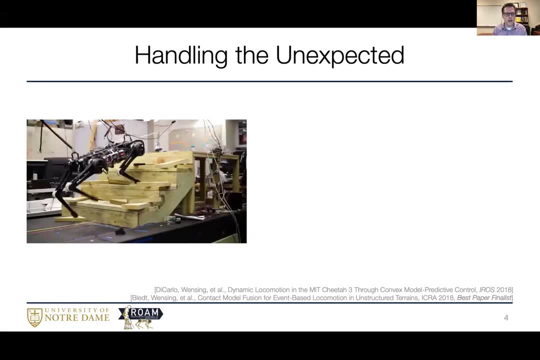 I think the main challenge is just kind of handling the unexpected and all the complexity of the environment on the real world. We've made some phenomenal progress on this recently. so here the unexpected for this robot is that it It doesn't know that the stairs are there. 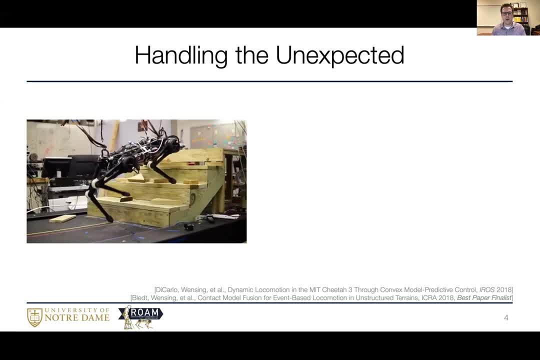 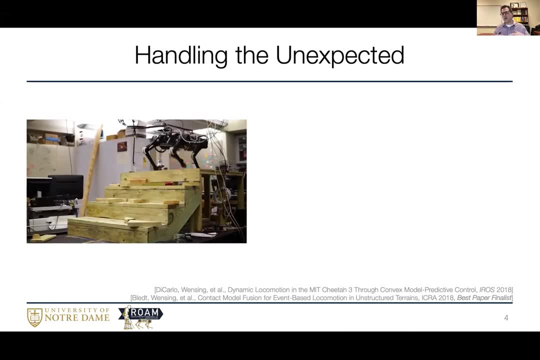 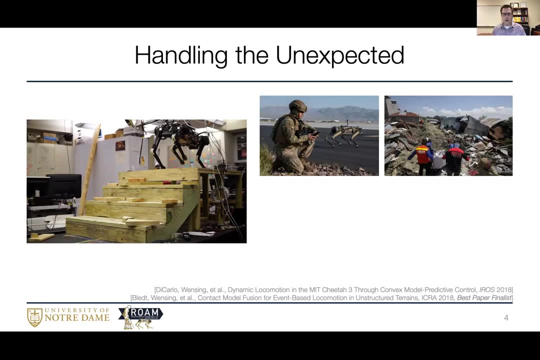 But the control policies and methods have been, You know, kind of tuned up and trained so they can work in this particular environment. But kind of my overall hypothesis is that you know, as we start to send robots out into the real world- whether they're supporting our troops or I going to a disaster zone, the scene of a fire or in our homes- kind of never going to be able to prepare them for everything. 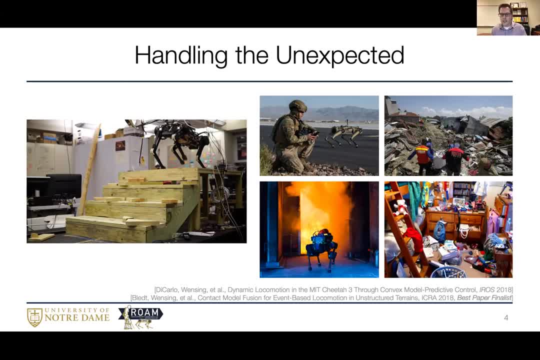 that they're going to see in these worlds, Right. Instead, our robots are going to kind of need to be able to reason through the consequences of their actions, Right, So that they can devise creative solutions that are tailored to the situations that they find themselves in. 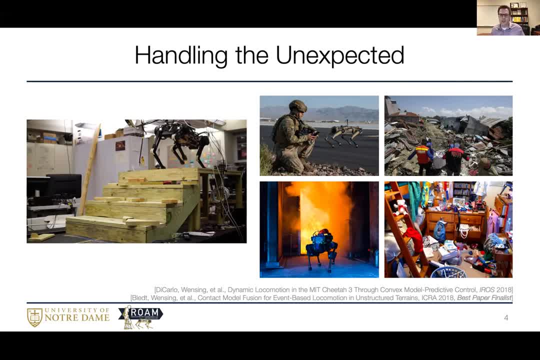 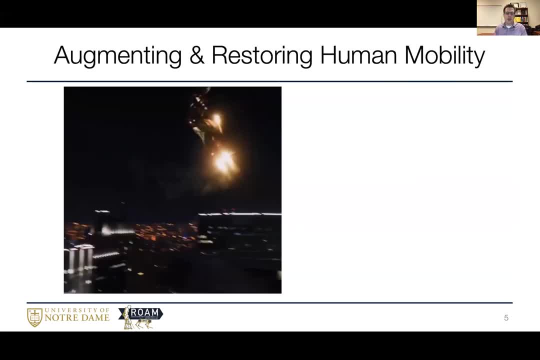 So I think that's the main, the main challenge and need for getting these robots out into the wild. It's very different when we think about human robot interaction applications And I think we have a little bit of an inflated sense of the state of the art here. 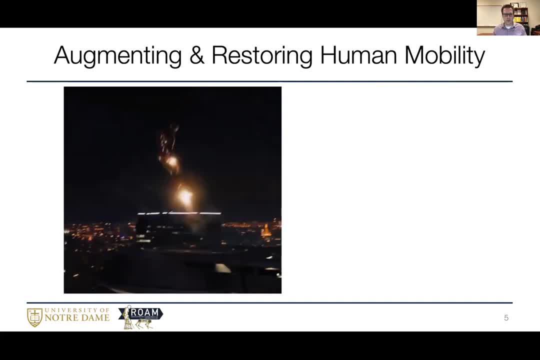 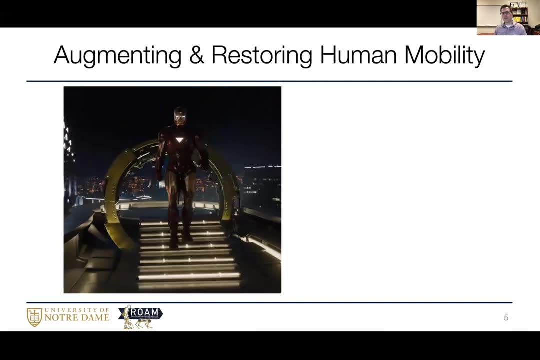 I based on you know kind of some of the things that we see on the big screen. So here's our friend Iron Man, And somehow his suit just knows That he wants to stop flying and just knows that he wants to transition from walking on level ground to walking down these stairs. to help them to accomplish that. 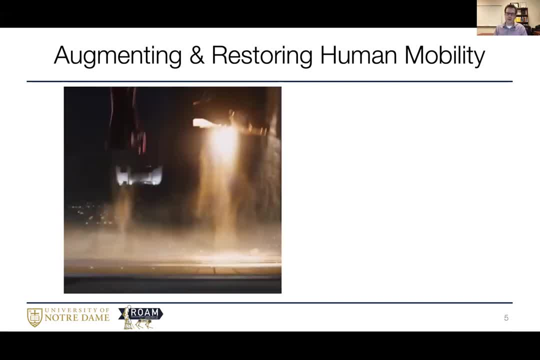 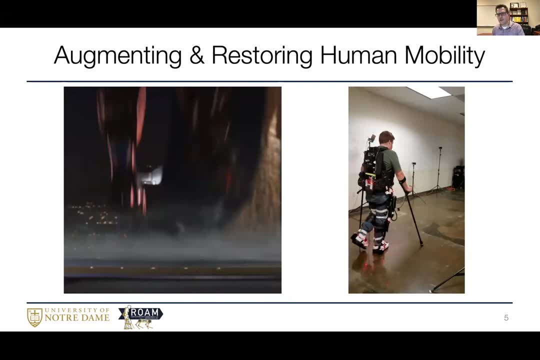 And that's just kind of very much in contrast to the state of the art. So here's a one of the phenomenal systems that we've worked with, that XO GT exoskeleton from exobionics, And here the motions just aren't quite as aren't quite as fluid. 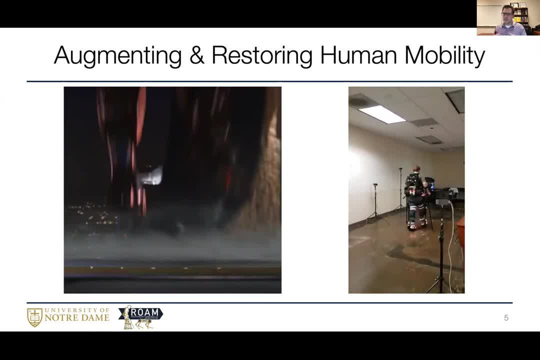 And that's because this device, you know, isn't Really able to to get into the mind of the human and pick up on their goals and desires as they, as they walk through the world. One of the challenges here is that, you know, everyone's gate is different. 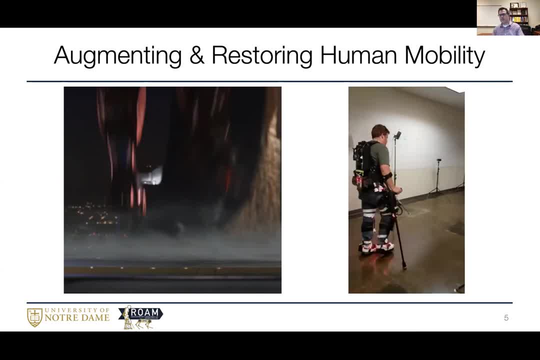 If you see your friend on the opposite side of the quad, you can tell that it's them just by looking at the way that they walk, And so a challenge here is really kind of the variability from human to human, In contrast with the variability in the environment, I think, for the more autonomous technologies. 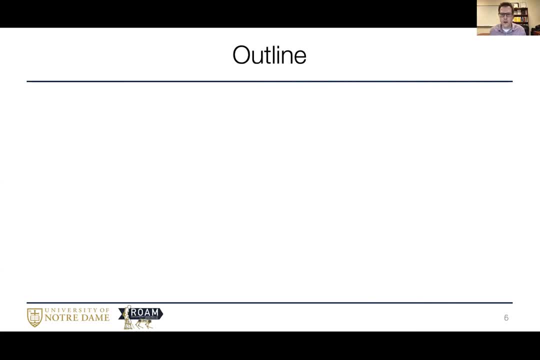 So today I'm going to talk a little bit about. I'm going to talk through Two different threads of work where we've begun to address these challenges. On the like a locomotion side, we're going to take a look at a new way that our robots can structure their prediction terms, the way that they think that the consequences of their actions as they move through the world. 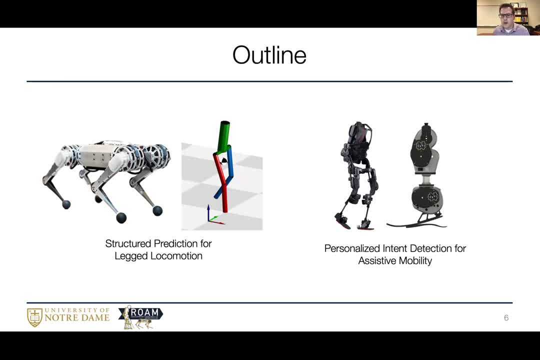 Then we'll take a look at some work that we've been doing on intent to set detection for assistive mobility. I'll focus most on an exoskeleton case and looking at how we can personalize these strategies For the people that are using these devices. 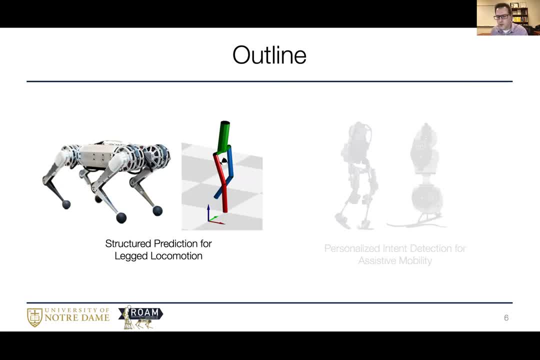 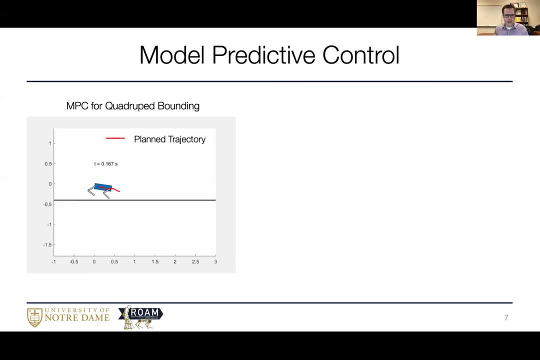 Okay, so let me start on this first part. So we're using a control strategy that's known as a model predictive control, or NPC for short. So before I start talking about this, I just want to kind of give a brief intro into the this way of approaching control. 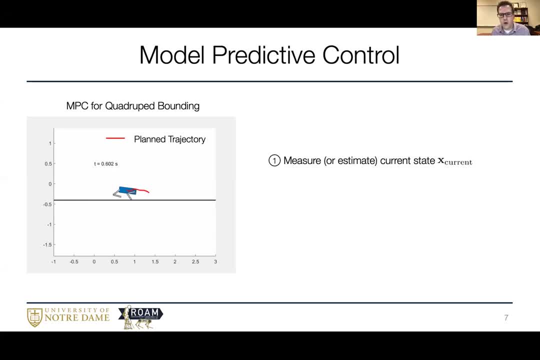 So model prediction control goes as follows: You measure or estimate the current state of the robot And then you come up with a plan Thinking about how to get from where you're at to where you want to go. We formulate this as a an optimal control problem posed over a hybrid system model for our robot, for which we've recently developed on some custom numerical methods for accomplishing this. 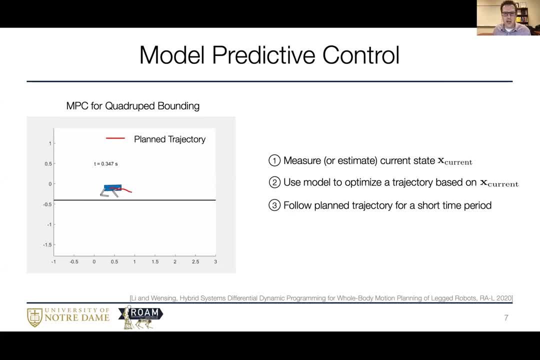 We then take and follow that plan for a short period of time into the into the future and then repeat this process. So if I look at my my robot here on the left, This red trajectory represents the plan. the robot follows that for a brief period of time into the future and then comes up with a new plan over and over again. 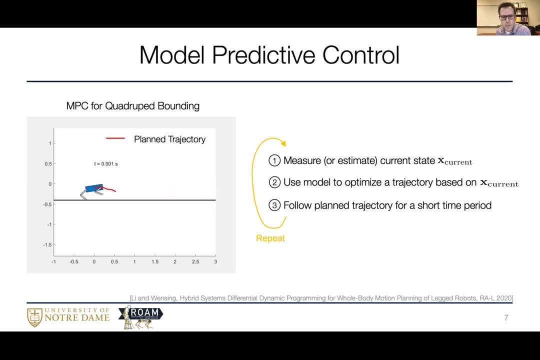 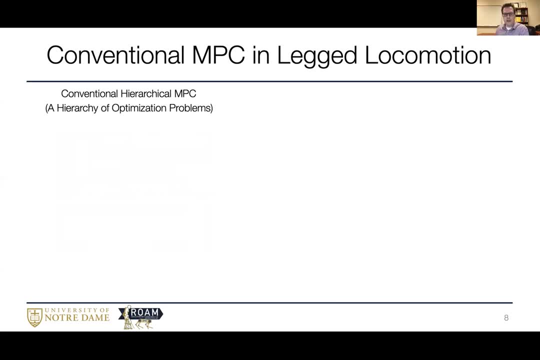 So what's the state of the art in terms of model predictive control? Well, conventionally, in the field I am, NPC is pursued in a hierarchical fashion where we solve kind of a hierarchy of optimization problems. So I am for. a robot needs to come up with a plan for a long horizon in the future, out a couple of steps. 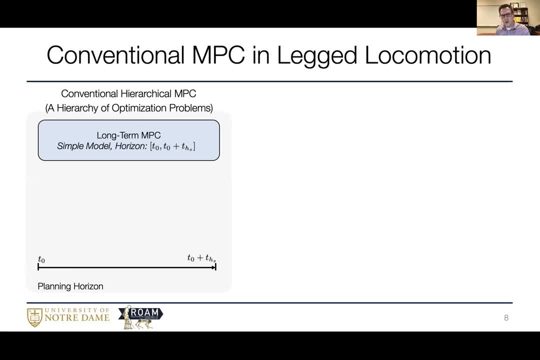 And that's computationally somewhat of a difficult problems. we often use simplified models of locomotion. So, as an example, in that video at the beginning, with the robot climbing the stairs, We used a lumped, single rigid body model. We thought about coming up with plans for how to apply forces underneath the feet to move this body through the world. 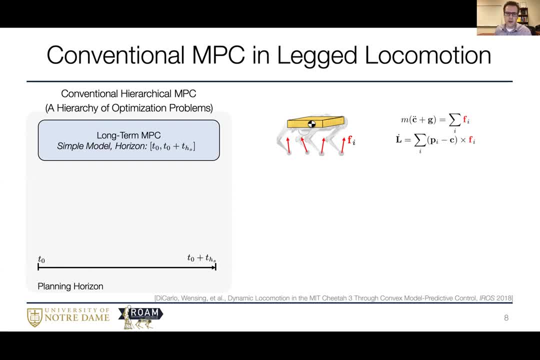 That allows you to focus kind of on the most important aspects of locomotion but still leaves a kind of a lot of additional detail that you need to stitch in. This requires another optimization process or a controller in order to fill in those details. So, for instance, when climbing up those stairs There were some swing like trajectories that were heuristically designed, along with an additional optimization based. 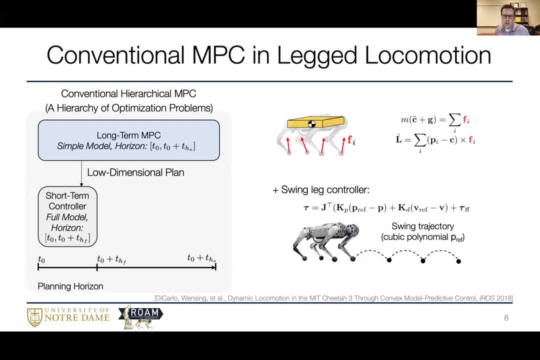 controller help track them. This works well in some isolated scenarios, But as you go out into more complicated environments, Some of these strategies break down And, in particular, you might need to think about re evaluating what type of model you're using. 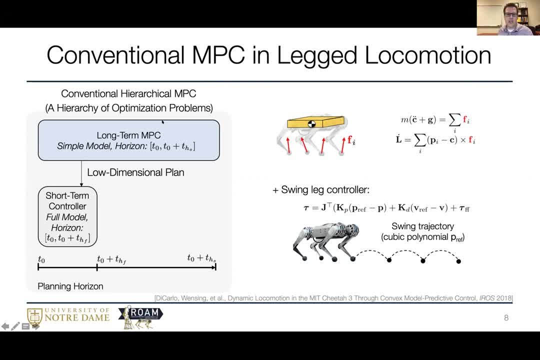 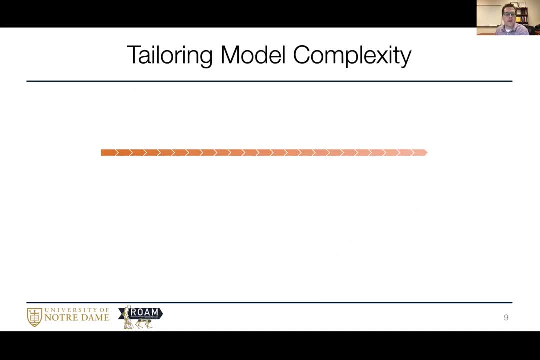 Frequently we think about there being kind of a an inherent trade off when making that choice of the model to use in our prediction. So kind of on one side of the spectrum for a choice that you could make. You could use a very simplified model, for instance, just thinking about the have the center of the model. 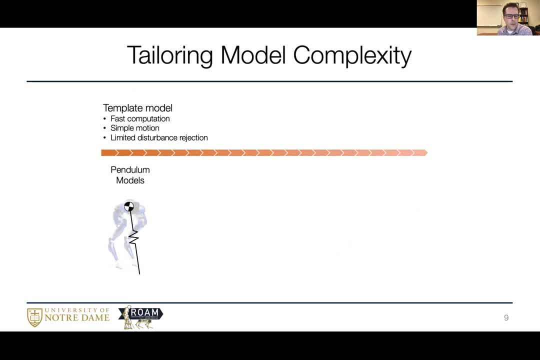 You could use a very simplified model. for instance, just thinking about the have the center of the model. mass moves through the world. The benefit of this is that by using a simple model you can do quite fast computation over it. But based on these simplifications, 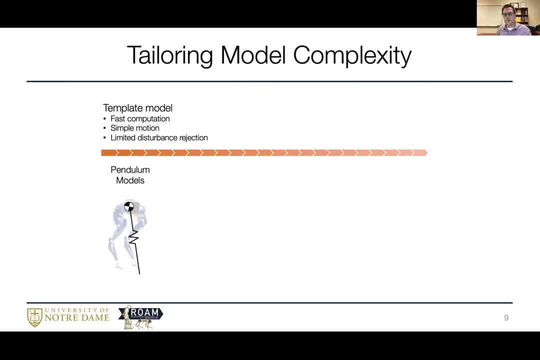 or restrictions. you often have limited disturbance rejection in terms of the pushes that you might be able to recover from or the terrains that you might be able to walk over as they shift under your feet. You can, of course, add in a little bit more detail. 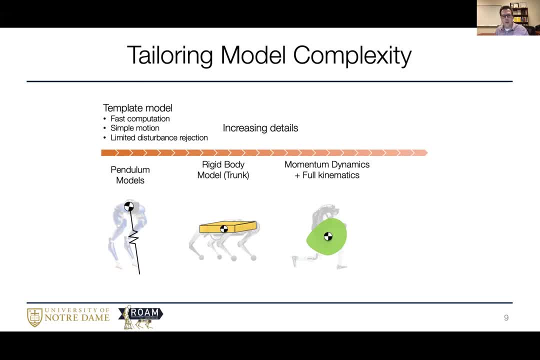 For instance, maybe considering the orientation of the body and thinking about how that's going to evolve into the future, or one that's become a little bit popular. is this model where you think about the overall linear and angular momentum, or the centroidal angular momentum of the system? 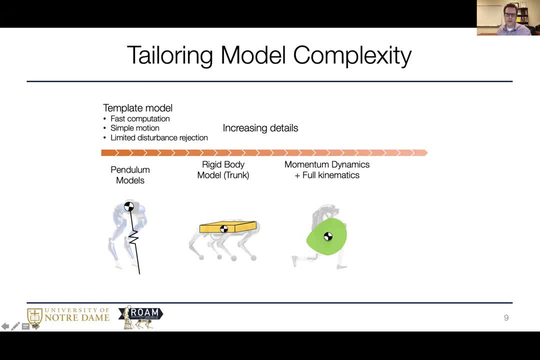 and thinking about the full kinematics, And this is kind of the model of choice that we've seen from the Boston Dynamics team recently with their humanoids On the complete end of the spectrum. you can consider modeling all of the detailed whole-body, rigid. 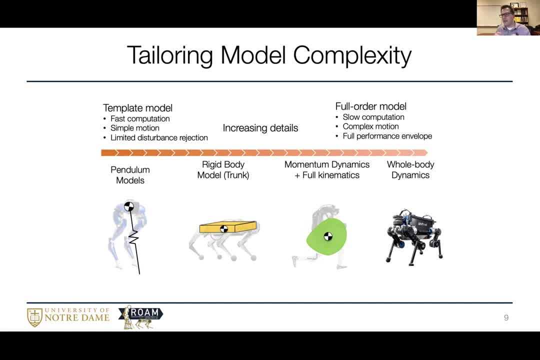 body dynamics of your robot, And the benefit here is that kind of by modeling everything, you can really unlock the full performance envelope of the system, But the downside being that since you're working with a more complicated model, the computations are a little bit more beefy to deal with. 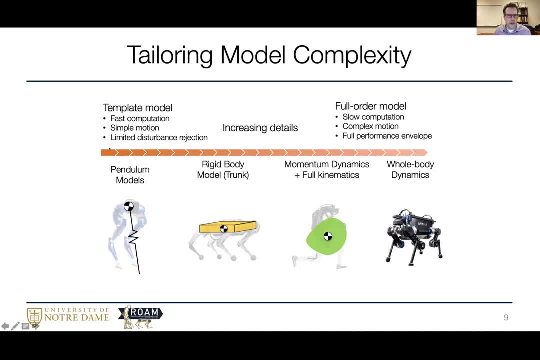 So in the past we viewed there kind of being this unavoidable trade-off: I'm either going to work with the simplified model that I can compute with quickly that has limited performance, or kind of, on the other end, I'm going to have to suffer you. 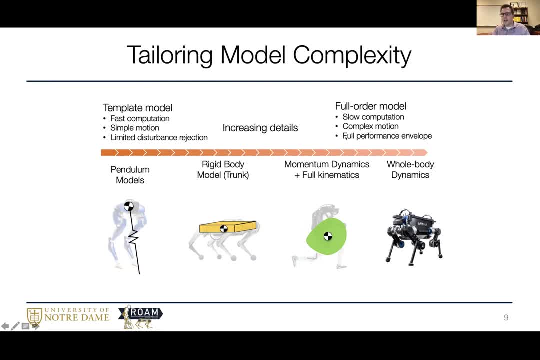 know slow, Slow computational performance, but really I can unlock and optimize any motion of my robot. Recently we've been rethinking that and asking the question: well, how can we kind of get the best of both worlds by rethinking about how we accomplish our prediction? 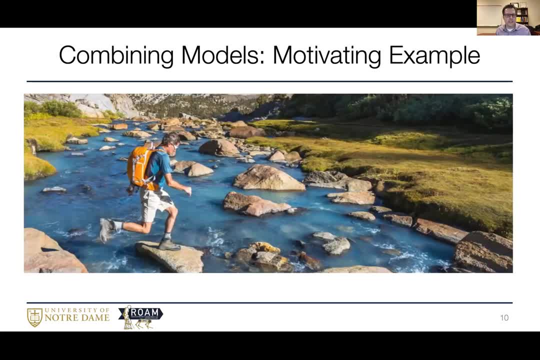 So to motivate that, I'd like you to put yourself in the shoes of this hiker. Let's think about if you need to get from where you're at to the other side of the stream. what details are you thinking through and planning out and thinking? 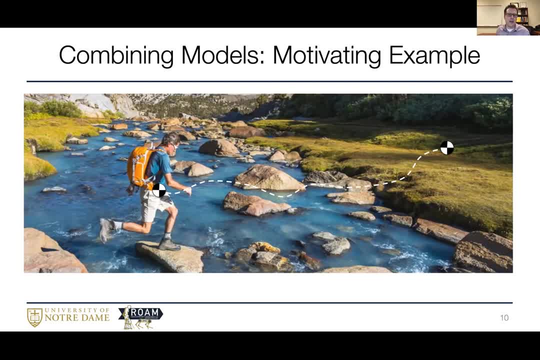 about your approach. Maybe you have some idea of the configuration that you're going to take for the next immediate step and maybe for the next one you picked out what rock you're going to put your foot on, But the further out that you're thinking about your plan, 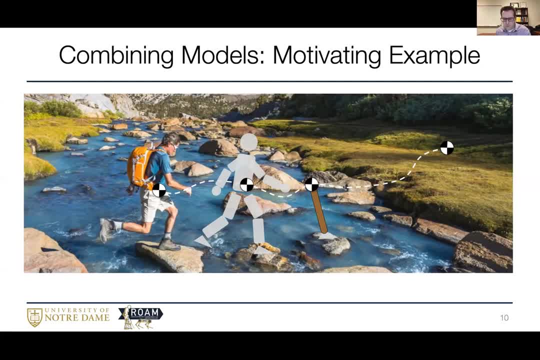 the more fuzzy it is, the more abstraction there is, So kind of at a high level. I think we need to be structuring our prediction more like the hiker here, in order to kind of squeeze the most performance out of our system without bogging it down computational. 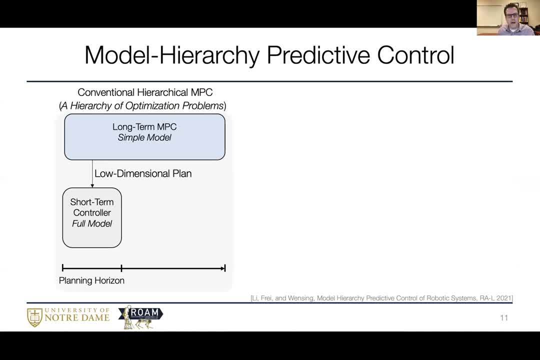 So conventional MPC is a hierarchy of optimization problems: Come up with a plan using some simplified model and then come up with another plan over the short horizon tries to match that, considering the whole body dynamics. Instead, if we structure our prediction more like the hiker, we're going to pose one problem. 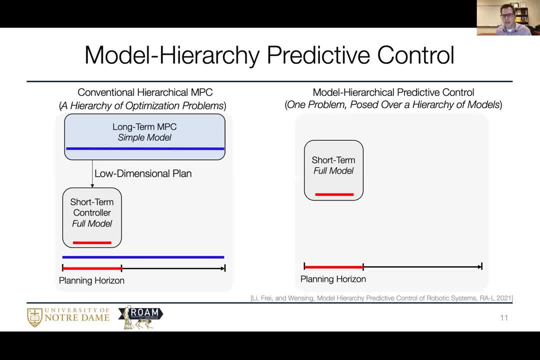 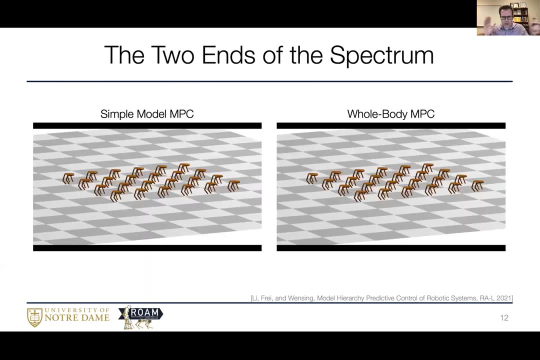 over a hierarchy of models, where we think about our whole body detail in the near term and use our abstract models to reason through the consequences of our actions further out Into the future. Let me show you some of the results of this. So first let's take a look at the two. 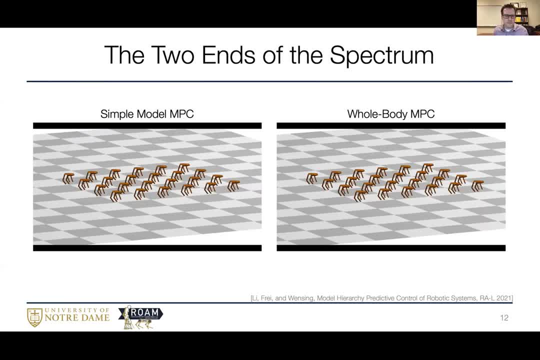 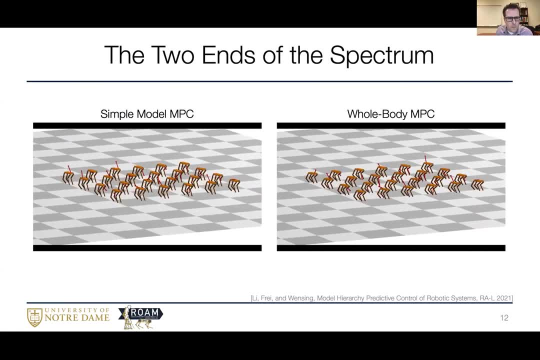 different ends of the spectrum, the simple model MPC and the whole body MPC, And I'm going to run some simulations where I'm going to put some disturbance forces on these robots as they try to run forward. So I got a bunch of different disturbances. 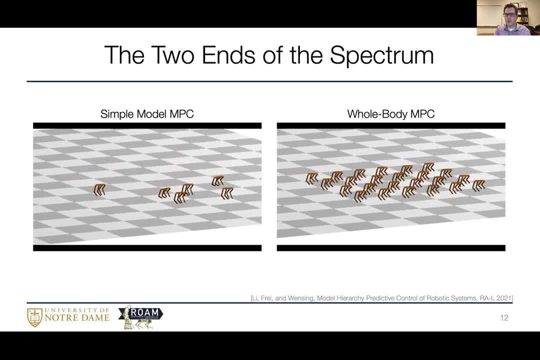 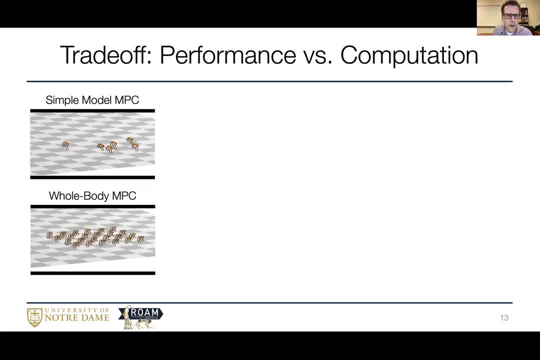 And when the robots violate joint limits or pitch too much they get removed from the simulations. We see the simple model MPC has more failures than this whole body MPC. We kind of took this anecdotal experiment and scaled it up on our supercomputer and looked at here on this x-axis. 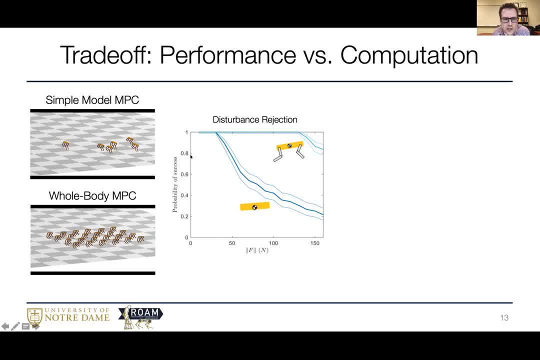 this is the force that's applied to the robot And on the y-axis is the probability of success. So here in the dark blue, this is showing the probability of success for the simplified model MPC. It starts to fail around 30 newtons of push. 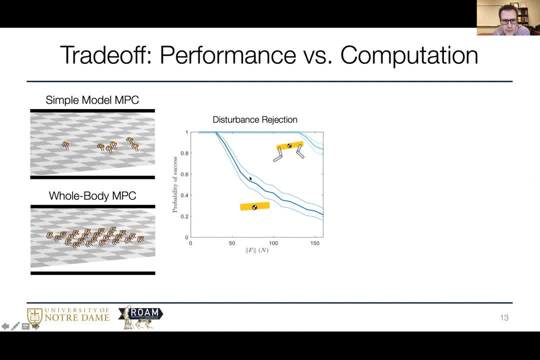 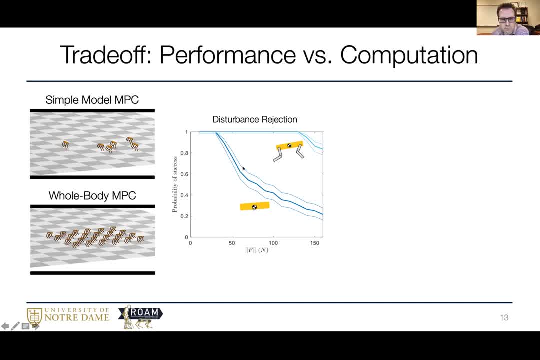 And then here, this tube that I'm showing you represents the 95% confidence interval that I have Based on the number of tests that we ran. If you instead use the whole body model, it's more robust. It handles these disturbances more gracefully. 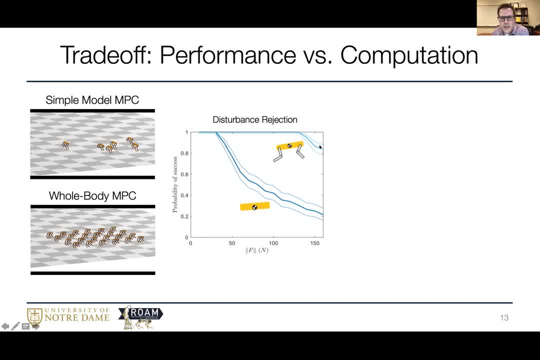 up to about 130 newtons and then it begins to degrade. Of course, kind of the price that you pay here is that the whole body MPC is about 10 times more computationally costly than the simple model MPC. Let's take a look at this model hierarchy idea via comparison. 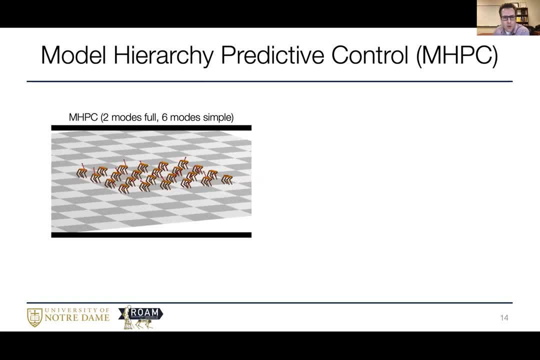 So here we're doing the planning where the robot, essentially for the next two gate modes, one stance and one flight- thinks about its full body detail and then uses that fuzzier, more abstract model to think about how things are going to go for the long term. 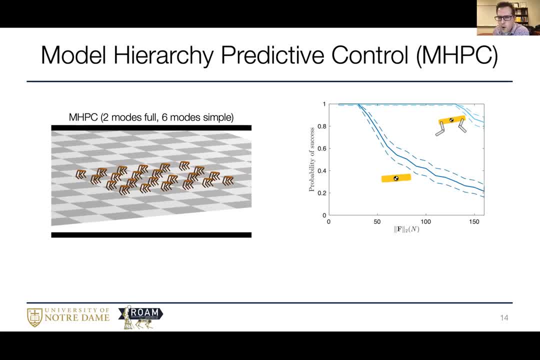 Here's the probability that we had before And now overlay in the performance of this model hierarchy. see that it doesn't do quite as well as the whole body MPC, but it's really close And particularly for these largest disturbances we're kind of within the range of error. 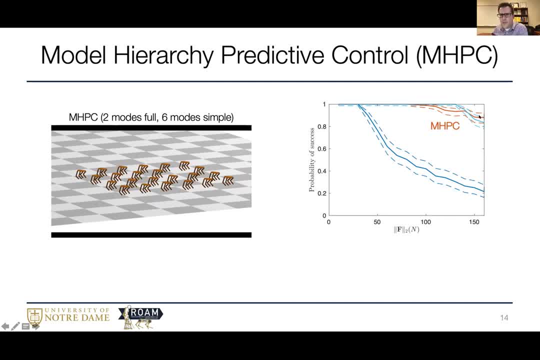 for statistical significance. So we perform about on par with the whole body MPC, but we do so while cutting the computational requirements by a factor of six. when we do this in C++, In MATLAB we get about a factor of two. in C++ we get a factor of six. benefit. 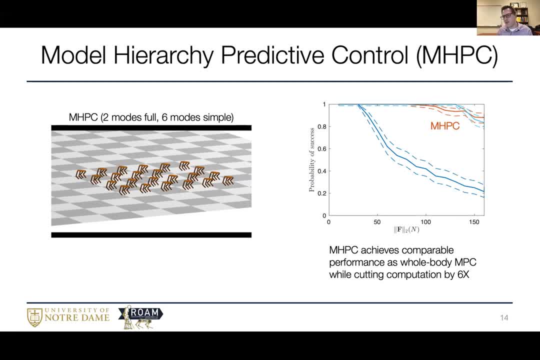 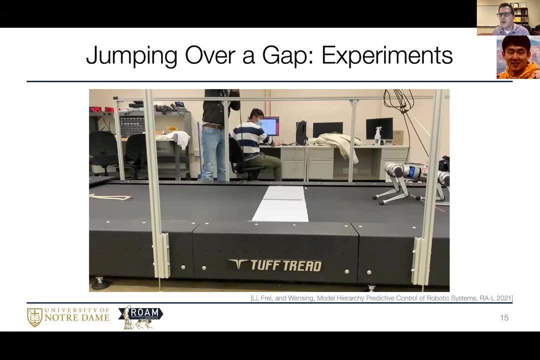 which I think is really exciting. By structuring the way that we think, through the consequences of our actions, we can keep the same level of performance as before while cutting this computation by six. We've also been looking at applying this in hardware, So this is an experiment from my student, Her Lee. 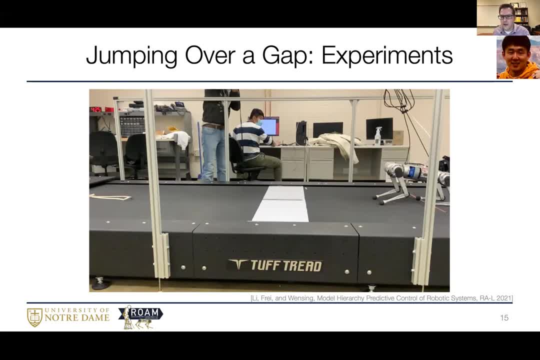 who worked on this project with our mini cheater robot that we have down in the lab. So here the robot's cheating a little bit. It knows in advance where this white area is that it's not supposed to step on, but it's able to use this model hierarchy in this case. 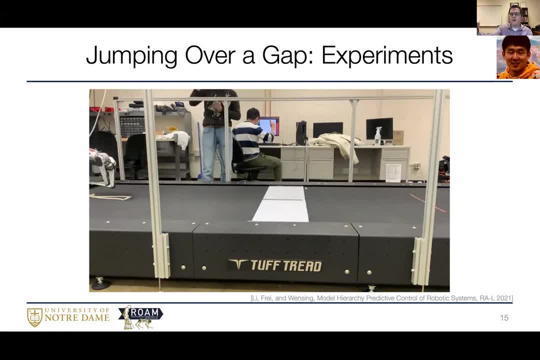 You know, when you have fewer computational requirements, you can think further out. So the robot's able to think about the need that it need to accelerate to jump over this gap earlier than if it didn't apply this model hierarchy strategy. Okay, so we're really excited about these results. 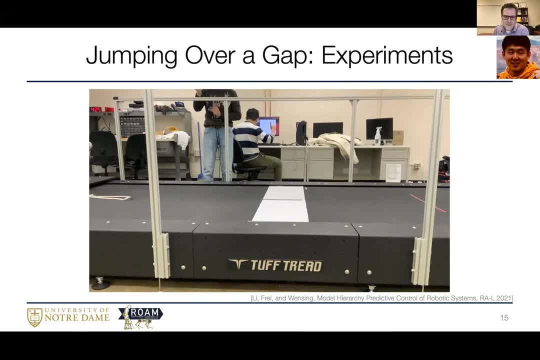 We're continuing to push on them in my group. But the one thing I would say is that here, in terms of handling differences in the environment, everything's done through control. But if you look at, you know, the biological realm, you see that you know some control actually happens. 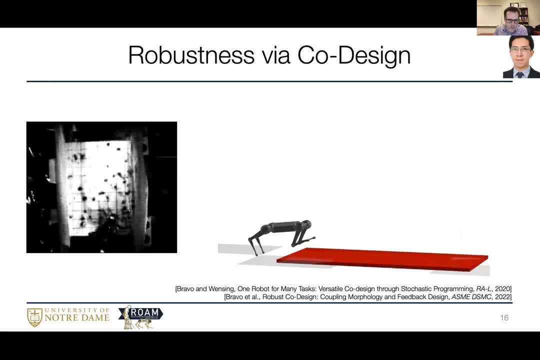 through the kind of passive dynamics of the body. So as an example, here's an experiment from Bob Full's group where they had a cockroach run across this little gel pad and they attached a little cannon to its back, And so they applied this disturbance to the cockroach. 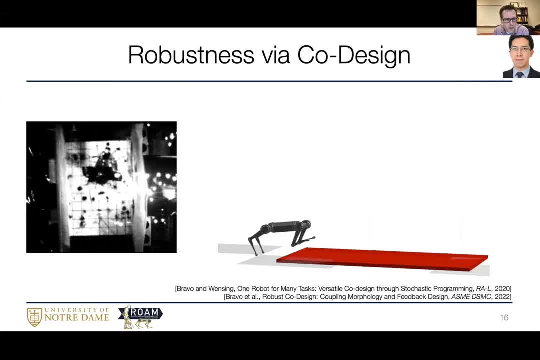 and then looked at the stabilizing response And what they found actually was that a great deal of the stabilizing response could actually be attributed to kind of the natural compliance of the robot's legs and not to any kind of closed loop centralized control. So what we've been looking at recently, 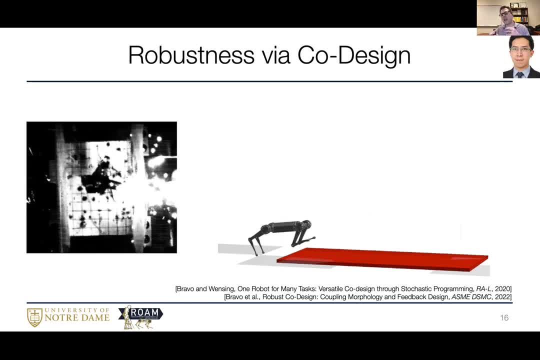 with my student, Gabriel Bravo, is how we can look at design and control together, So that we, rather than just designing a robot and then handing it off to a control designer, we treat these problems together in order to ensure synergy between them. 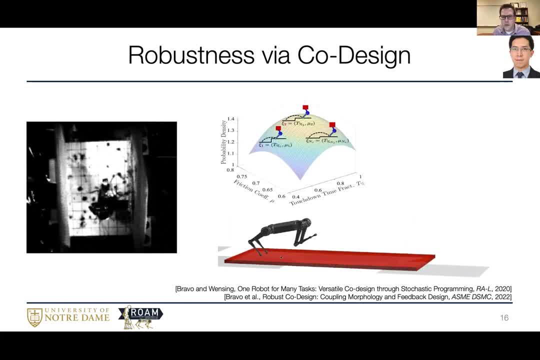 And so what we've been looking at is how can we design a robot so that it's able to handle all sorts of different type of, you know, terrain conditions and such that some of the response to those terrain conditions are happening through kind of passive compliance? 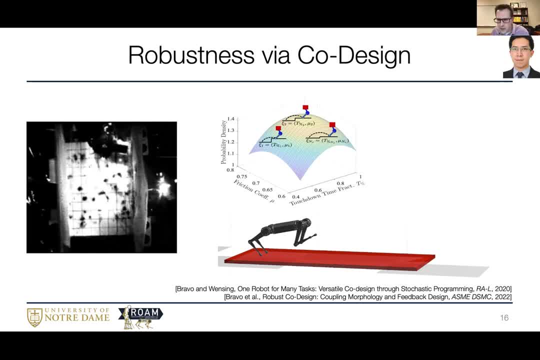 that are in the mechanism. We've been doing this mostly in simulation, but we have some initial hardware that we've built in that We're just starting to test that I'll look forward to reporting on further down the road. I wanted to include this kind of as a little tie. 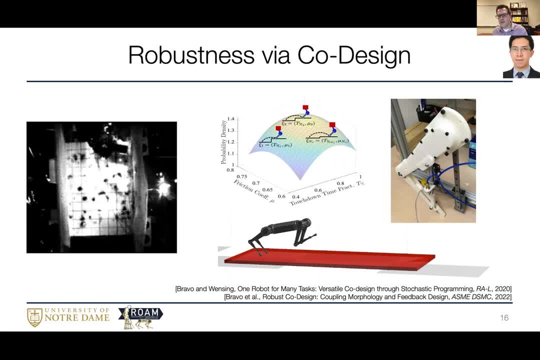 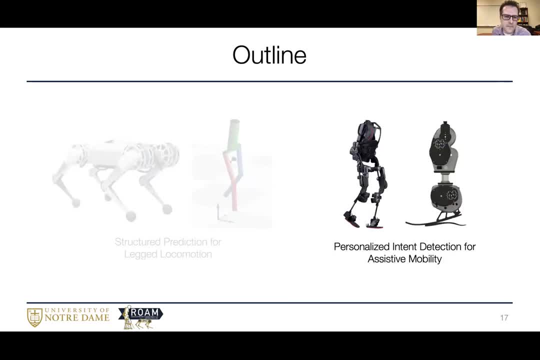 into what Laura is working on in terms of kind of the importance of compliance and finding ways to engineer compliance into our robots. Okay, So we've addressed this way for our robots to think through the consequences of their actions to handle more challenging environments, And I'd like to shift gears and talk about how we 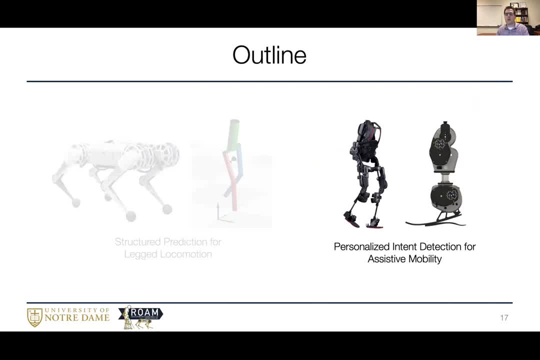 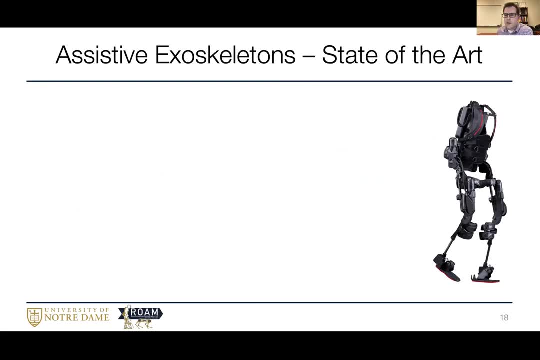 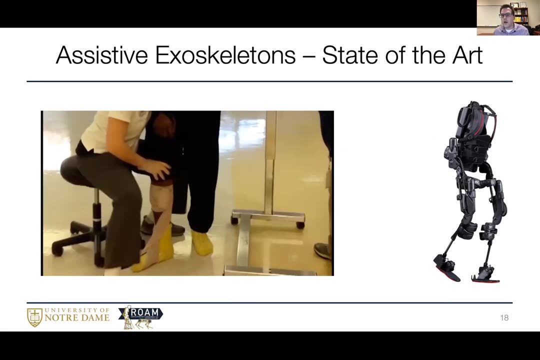 can handle the variability from human beings that might be inhabiting our assistive devices. So in terms of the state of the art for rigid exoskeletons, this is kind of what it might've looked like in rehabilitation before exoskeletons were available. 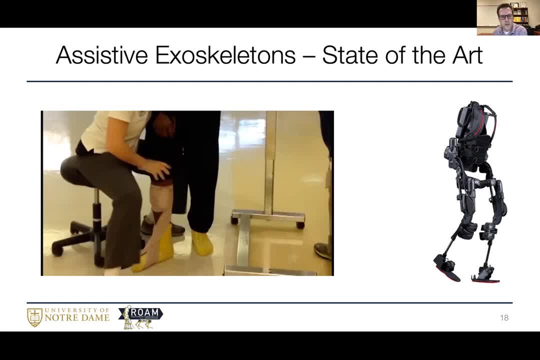 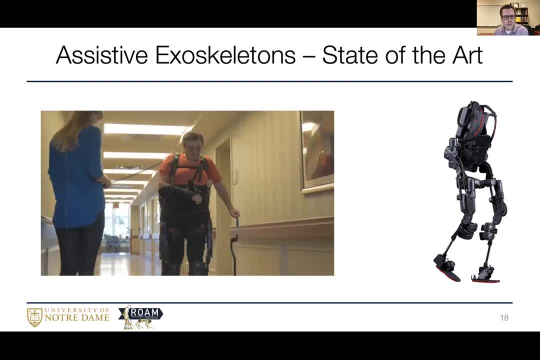 with physical therapists manually manipulating limbs to move them through gait. Now, with the use of exoskeletons, we can reduce the burden on therapists. We need fewer of them. It's fewer of them, It's less taxing and can produce more repeatable gait patterns. 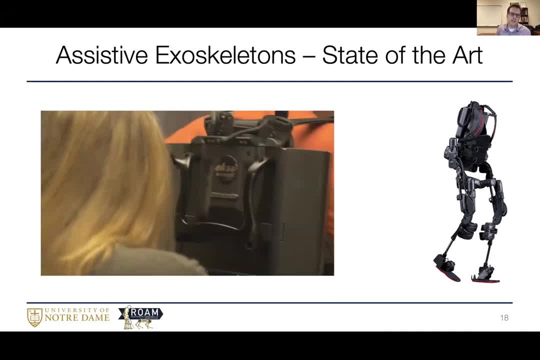 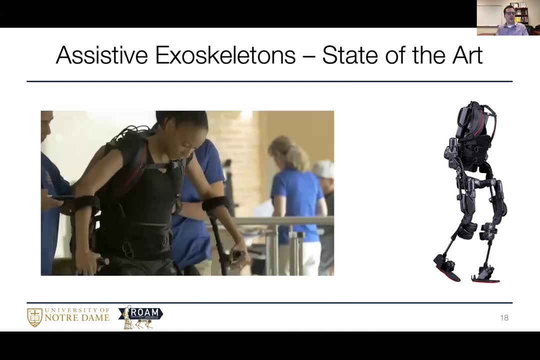 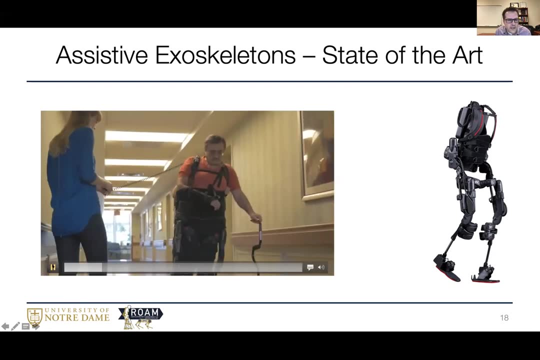 during rehab. The kind of end goal here is that we'd like these devices to be able to go home with people and out into the community so that they can interact with the community from a standing posture as opposed to from a wheelchair. One of the challenges with these devices is kind of here: 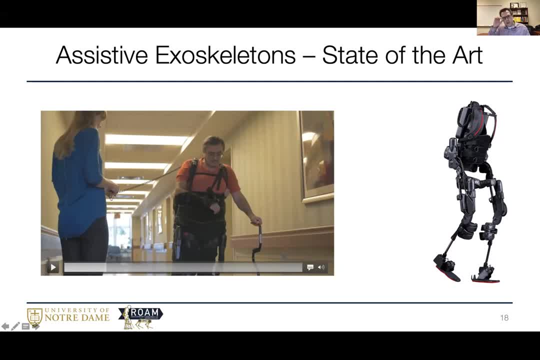 you can see, this therapist is holding a pendant, And so anytime a change needs to be made to the gait, she's kind of keying that into the device. Instead, what we'd like to be able to do is to pick up on small changes in your motion that might telegraph changes. 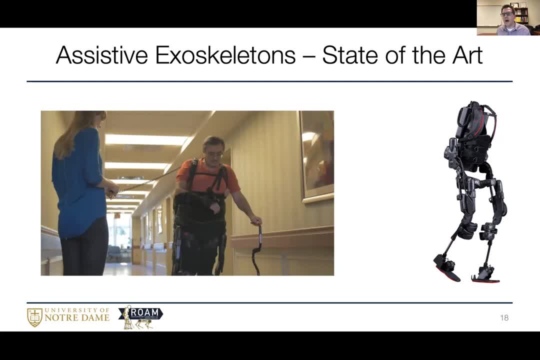 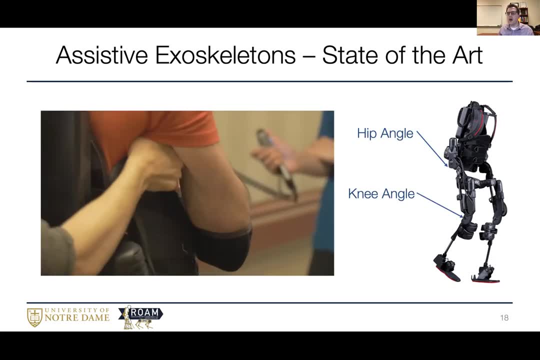 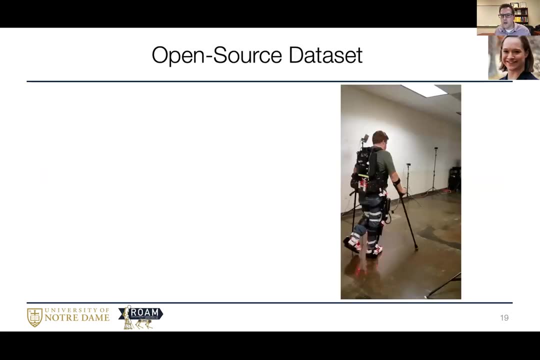 that you wanna make to your walking speed. And we're doing that by looking at sensors that are already onboard the exoskeleton, in terms of angles of hip and knee motors, as well as currents of those motors and contact sensors under the ground. So we have an open source data set. 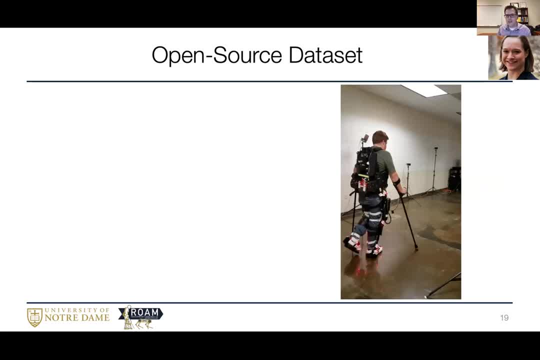 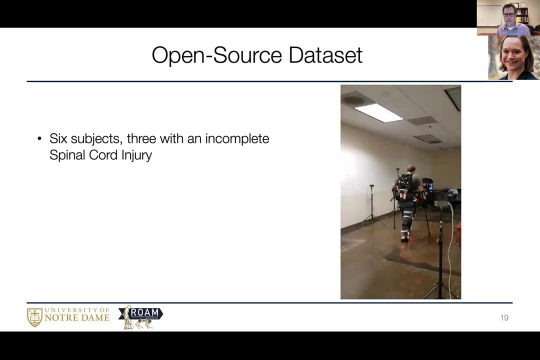 that we've been using to conduct our studies And, if you're interested, I hope you might use it too. So this was a study that was conducted by my student, Taylor Gambon, with our industrial collaborators at ExoBionics. So Taylor ran a study with six subjects. 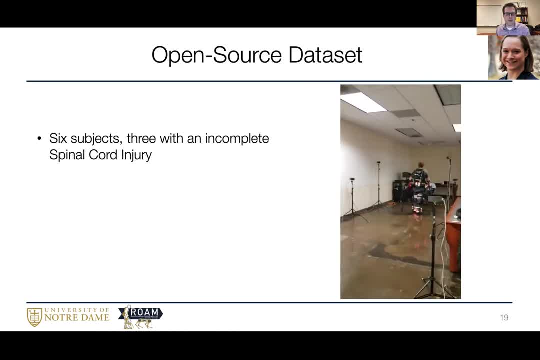 three uninjured individuals and three with an incomplete spinal cord injury, And she had them walk through this mocap arena And commanded them to either speed up, slow down or make no change in their gait. We monitored all those sensors onboard the suit. 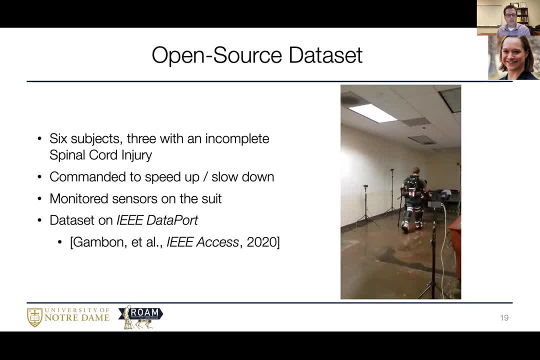 and have made that information available as part of an open source data set that's associated with Taylor's recent IEEE access paper. So I encourage you to take a look if you're interested in this area, And if you have any questions, please feel free to reach out. 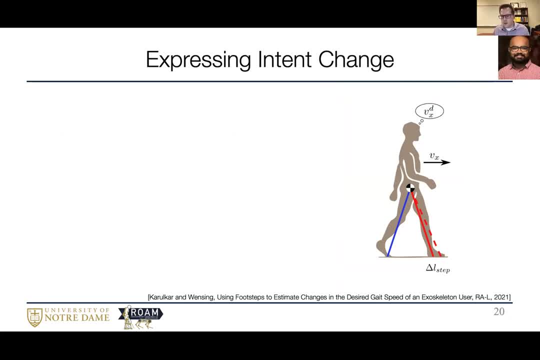 So, again, our goal is that we'd like to be able to use these, these sensor readings that we've collected in order to estimate that the user has made a change in their desired walking speed. So, if I think back to kind of like the first part of the talk, 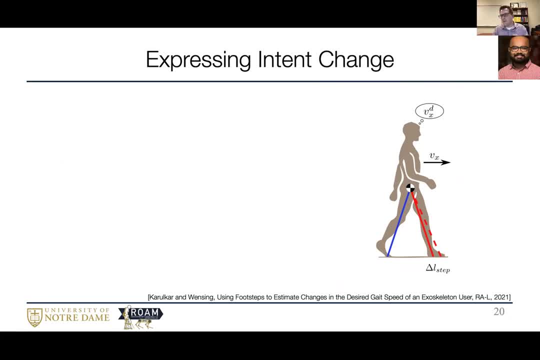 these simplified models that we were using to plan locomotion. they were often focused on figuring out you know what force is being applied under the foot at a specific location And you know kind of the reason being that when you select a footstep, you're stuck with it. 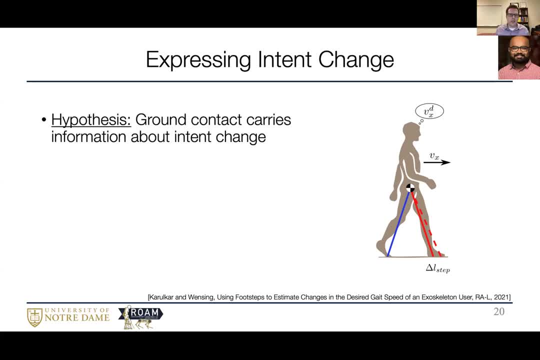 both now and into the future. Our hypothesis was that choices of ground contact would carry a great deal of information regarding the intent of the individual And, in particular, we were motivated by some recent work that showed that changes in step length are well correlated with changes in gate speed from step to step. 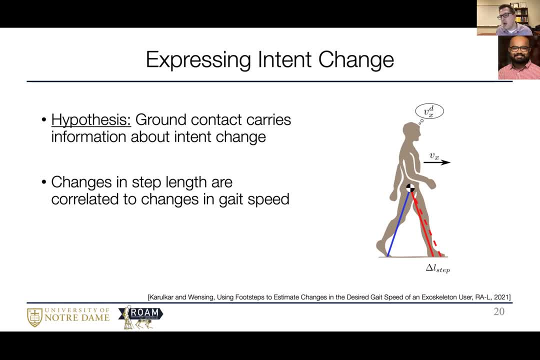 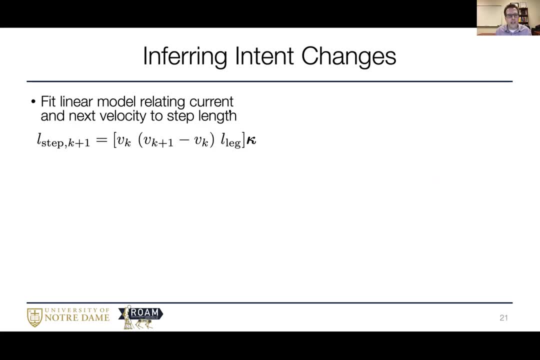 So we've been using this insight to pursue intent detection through the following method: We collect a bunch of data and from that data we glean the walking speed. So here, VK is the forward walking speed on the kth step. We glean that data, as well as other features of the gate. 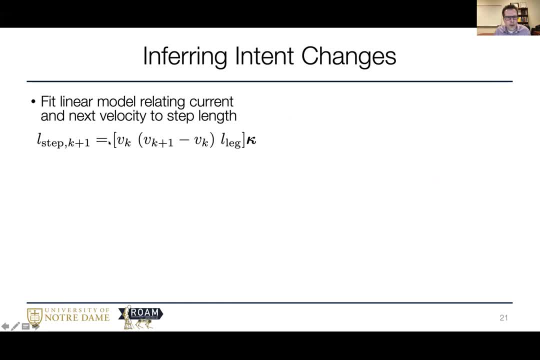 for instance, looking at the step length, And based on those previous studies, we fit a linear model that relates the current walking velocity and the change in walking velocity and the leg length to the step length that we observe. Here we're basically viewing the velocity. 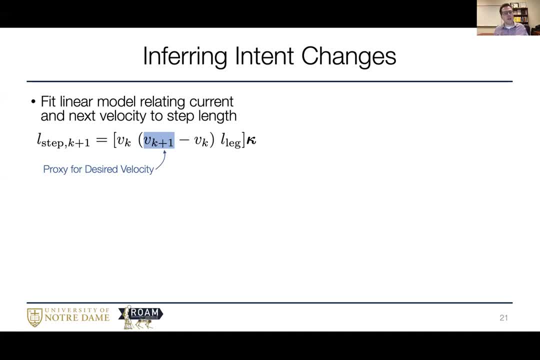 in the current step at the next step. And then there's a proxy for your desired walking speed. at the current step We then consider a state vector that contains both the center of mass position velocity and- that's kind of latent, unknown desired walking speed. 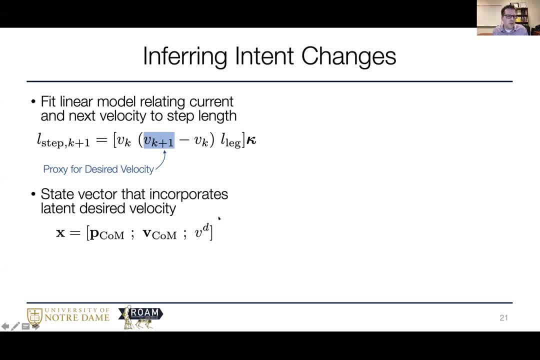 We don't know it, But we now have a measurement model for it which enables us to apply Bayesian strategies. we're using common filtering tools in order to infer walking speed. Let me show you some of the results. So here, on the x-axis, I'm showing you the step. 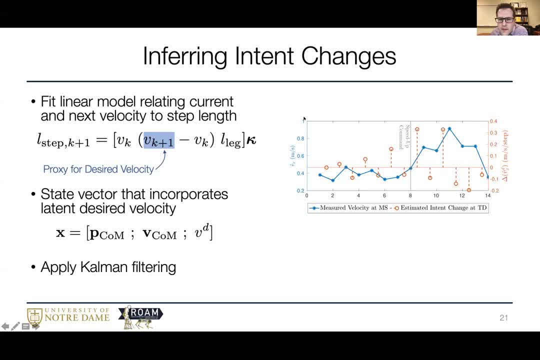 number and on the left, in blue, this represents the measured walking speed. So here, on this eighth step of the data, the user was commanded to speed up, and so, between this mid stance of one support for their leg, they sped up from about you know 0.45 up to you know 0.75 meters per second. 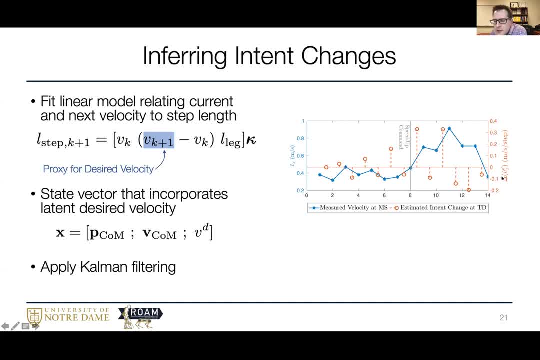 On the right, here in orange, is the change in the estimate of the desired velocity from step to step. In other words, this is, you know what, how much we think the user wants to speed up on this step. So here our estimator is saying: we think they want to speed up, you know, 0.3 meters per 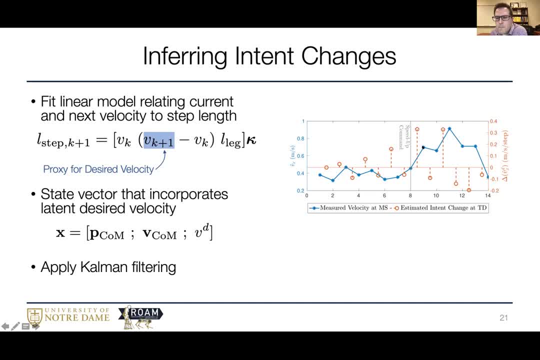 second, which agrees, you know kind of quite well with how much they want to speed up. So here the, you know, essentially, the estimator is working when the slope of the blue line matches the sign of this, of this stem plot. And through this strategy we were able to get performance up to about, you know, 78% success rate at preemptively identifying. 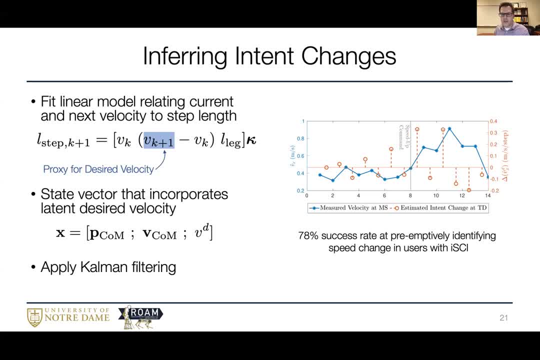 speed change in users with incomplete spinal cord injury, That's to say, you know when their foot would touch down. we would identify- oh, you probably want to speed up, and then, by the time that step was over, they had sped up 78 percent of the time. the challenge with this, however, was 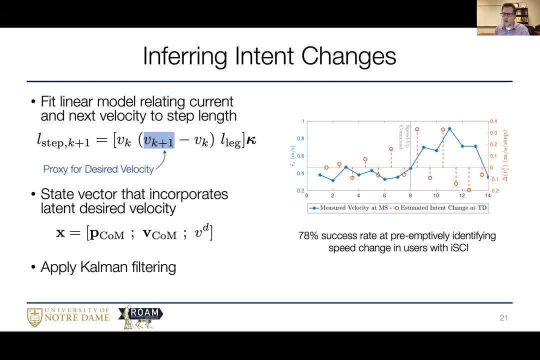 that for each individual, we required a good bit of training data. we needed, you know, 70 steps of training data to get these results. and if you think about, you know, in a rehab setting, you want to spend all the time possible doing rehab, not a lot of time gathering data to calibrate the. 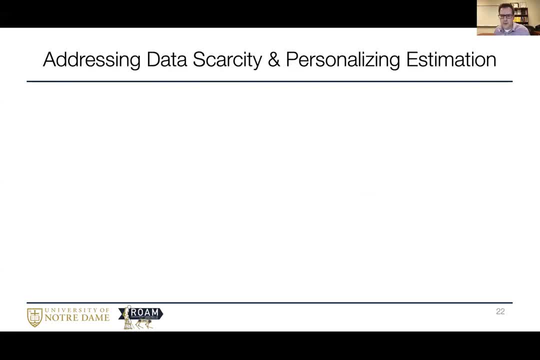 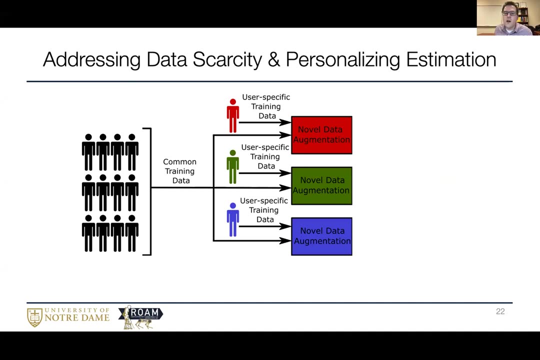 exoskeleton to the individual. so we've recently been asking the question: well, how can we address this data scarcity problem? and, in particular, if we have a bunch of data from healthy individuals, how might we be able to combine that data set and, just you know, sprinkle in a little bit of data? 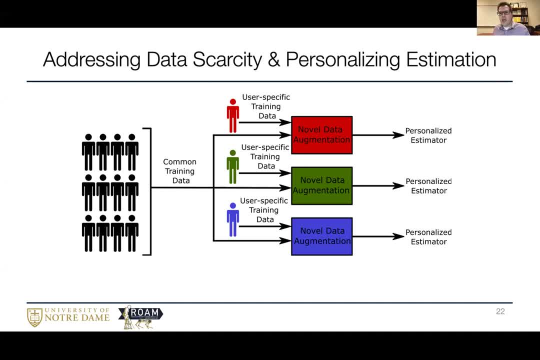 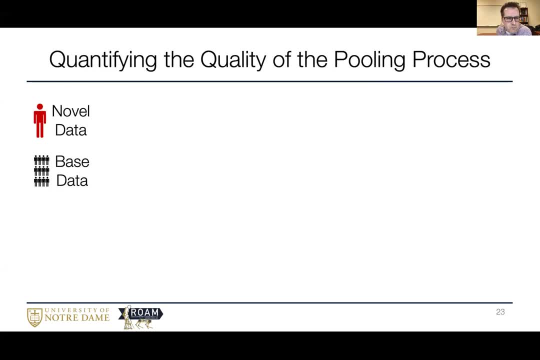 from a specific new user in order to get a personalized estimator. we've been doing that, i, through the following means: let's assume we have a bunch of this base data and some additional novel data. we first take that base data and we kind of shift it so that it matches the novel data. we we shift it so it has the same mean and same standard deviation. 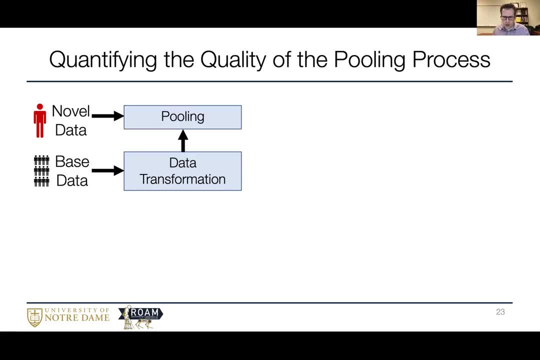 and then we pull this together with the novel data and there's, you know, a number of different things that you consider, consider here when doing cooling. you could, you could, ask the question: you know, which base user should i, should i use? you know, should i bring the data of person one and 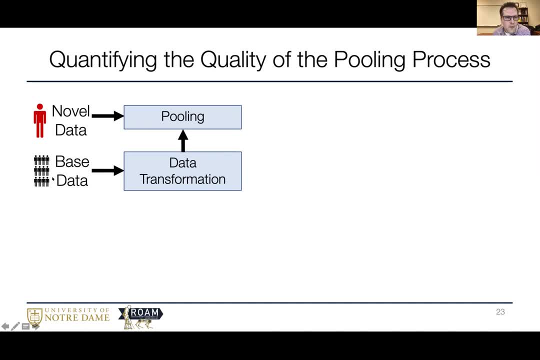 two or or three and four, which would be most informative. um, right now, we've just been using all of the base data that we have. another question that you might have is: if i have some novel data, should i use all of the trials? and i think you know our conventional 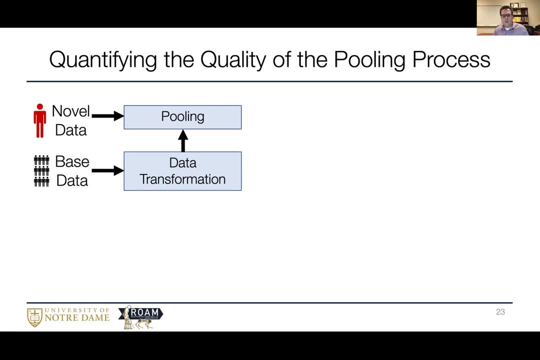 wisdom is, you know, use all of your data, um, but in our case, for people that have an incomplete spinal cord injury, they might have some, you know, motor spasticity such that some of the trials are, you know, not so informative of their behavior overall, and so what we've been looking at is um. 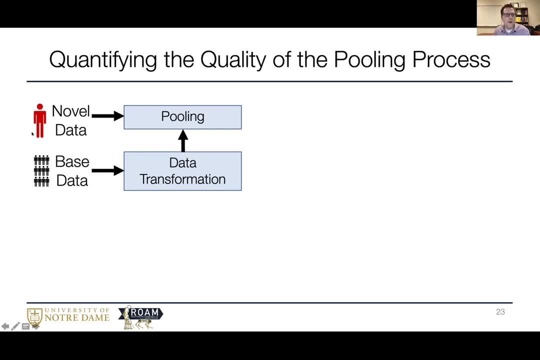 how do you, how to basically, uh, be selective about what novel data to use in this pooling process? once we are done with the pooling, we have some- i, you know- data on the desired velocity, using that trick from the previous slide, and some gate features that include, you know, the step length. 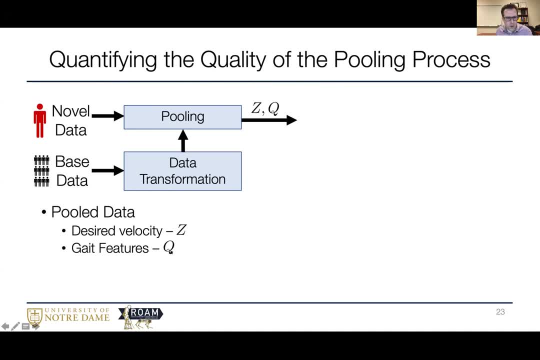 step, frequency and that type of stuff. we're then evaluating the quality of this pooling using some information, theoretic notions, in particular using the mutual information between this, these desired velocities, and the gate features that we measure. so this mutual information kind of represents the- uh, kind of formally it's the kolbeck-leebler divergence between, you know, the joint. 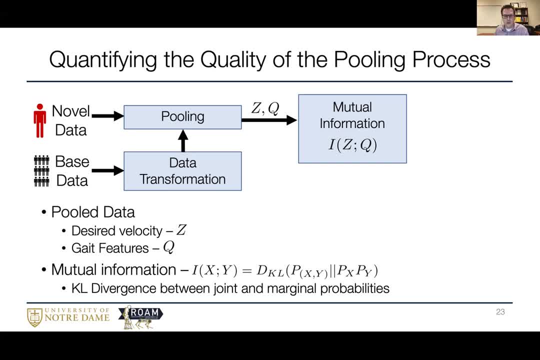 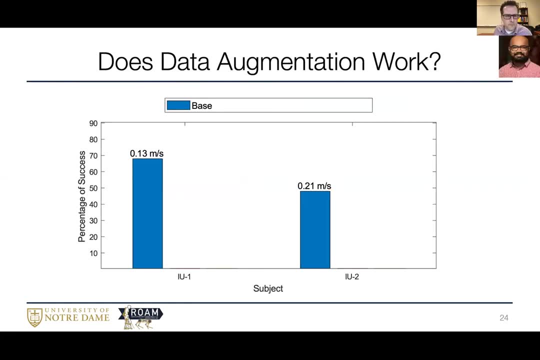 probability distribution and the product of two marginal probability distributions and kind of captures the uh, kind of information in the correlation between these variables and this gives us basically an anticipated quality uh for our estimator. let me show you how this does. so if we just use uh, the the base data, here i'm showing you the performance of our estimator for. 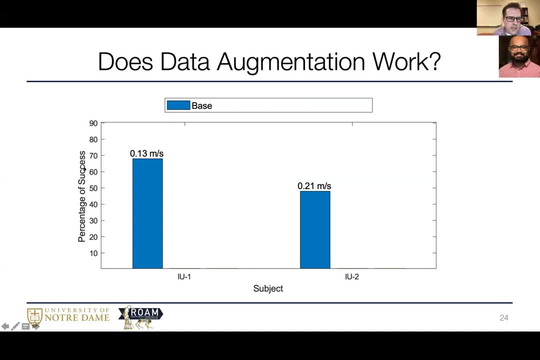 two of our subjects: um, and the height of the blue bar represents the, the percent percentage of success in correctly identifying speed up or slowdowns. and here this number represents the rms. uh velocity error in terms of the difference between the measured and the, the estimated velocity. one thing that you 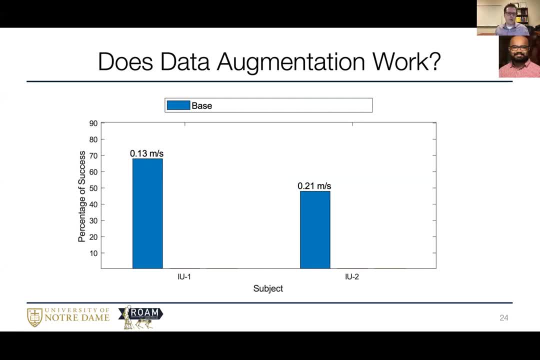 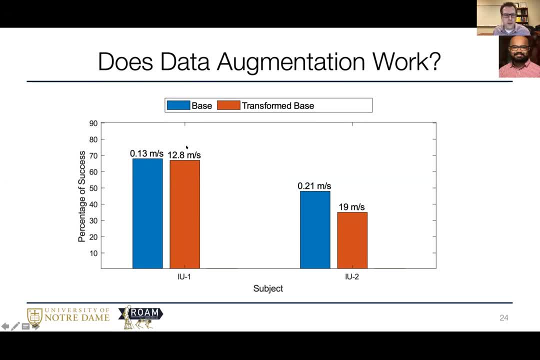 the probability of success and makes the velocity estimation quite, uh, quite bad. so you know, just for reference, 12.8 meters per second is about twice the speed of an olympian running in 5k. so that's uh, it's a lot of velocity error. but if we take this data and we just sprinkle in just 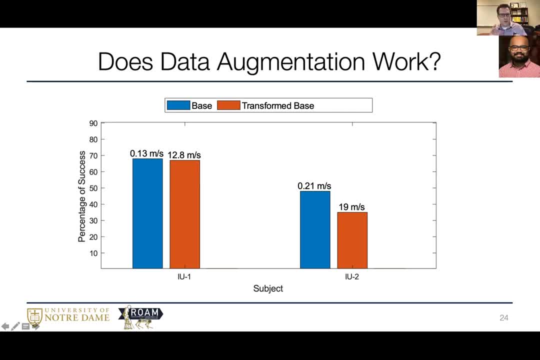 a little bit of novel user data talking, you know, 8 to 12 steps worth um, we end up getting estimated performance that is even better than we had before. so we're going from 70 steps worth of training data required to 70 steps worth of training data required to 70 steps worth of training data required. 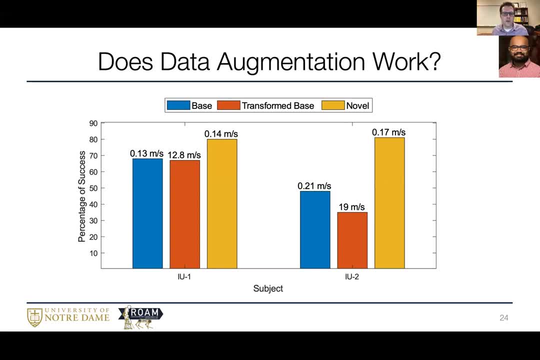 down to 10 and by pooling this with with base data, we're able to uh, amplify the performance of our estimator, which i think is really exciting. i should mention this is work done by my student, rupak karulkar, who's getting close to graduating. okay, so that's some of the work we've been doing. 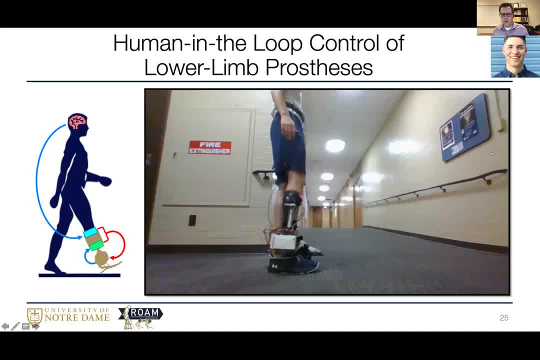 on the exoskeleton side, i'd like to quickly plug, uh, some of the work that we're doing on lower limb prostheses in terms of getting the human in the loop. there's many options with that exoskeleton. we were looking at sensors that we were looking at sensors that we were looking at sensors that we. 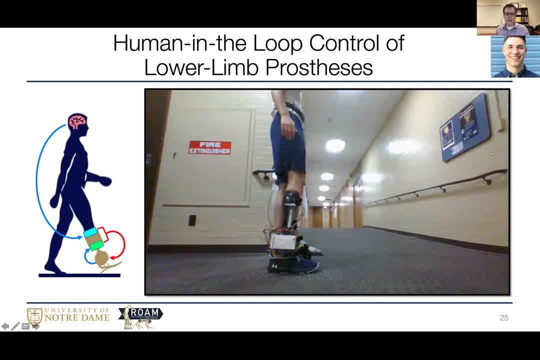 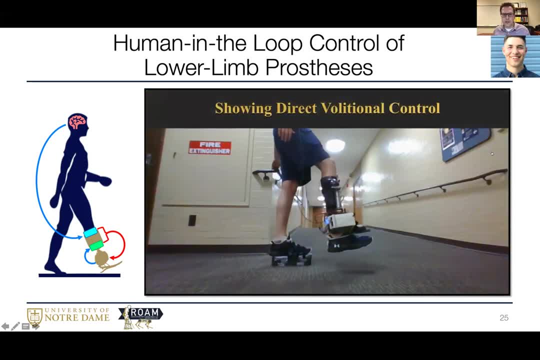 were already on board the device, but, in terms of uh understanding the user's goals and intentions, there are other sensors that are available, um for instance, emg electrodes that we're we're looking at using, and so in the past um a lot of control strategies have either been purely autonomous, 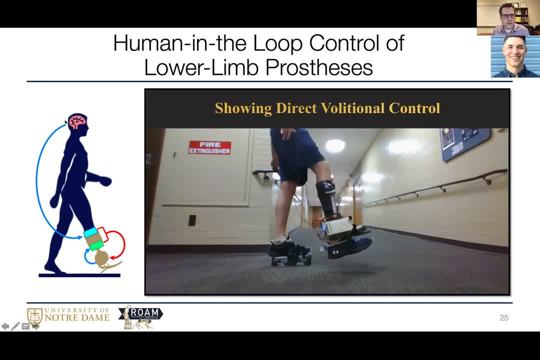 taking feedback from the prosthesis itself, or purely volitional, in terms of, uh, taking readings from an eeg skullcap or emg sensors on on board the prosthesis. and so what my student, ryan posh, is going to do is he's going to take a look at some of the sensors that we're already on board. 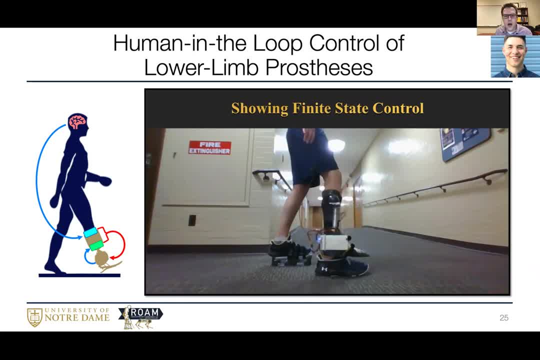 the device, but in terms of understanding the user's goals and intentions. there are other sensors. that ryan posh is looking at is: how can we combine these two together? um, so that if you just want to walk on level ground, you don't have to think about it. you can let the autonomous controller 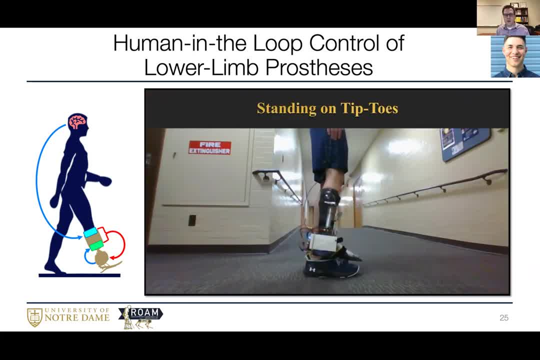 take, take care of it. but if you want to do something special, like stand up on your tiptoes, you have the flexibility of doing that. um, and so ryan's uh done some great work on this for right at the beginning of some human subject studies on it, and i again kind of look forward. 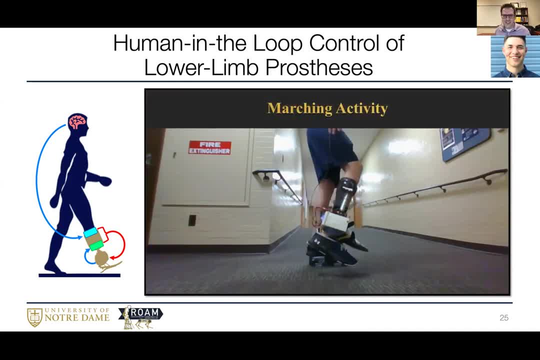 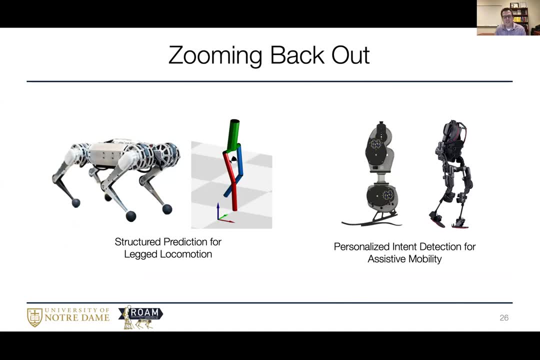 to telling you about down the road. okay, so kind of zooming back out, uh, as we look to send our robots out in the wild. uh, for our autonomous legged robots managing the complexity of the environment, having ways for our robots to think through the consequences of their actions. 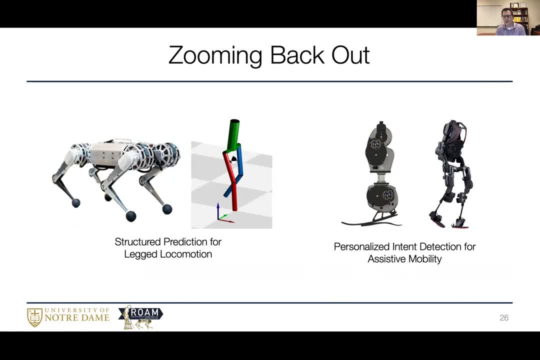 is, uh is real challenge that we've been taking a look at. and for our assistive devices, i think the main challenge comes from kind of the variability of the different humans that are using it. i'm excited about some of the recent work that we've done there, so with that i thank. 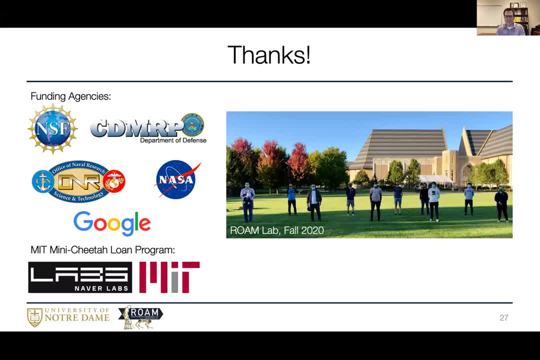 you for your attention and i'll i'll thank my funding agencies and looking forward to laura's talk. thank you, uh, patrick. uh, very nice talk. uh, i would like the audience to write down their questions or just type them into the chat. um, at the end of laura's session we can group and have 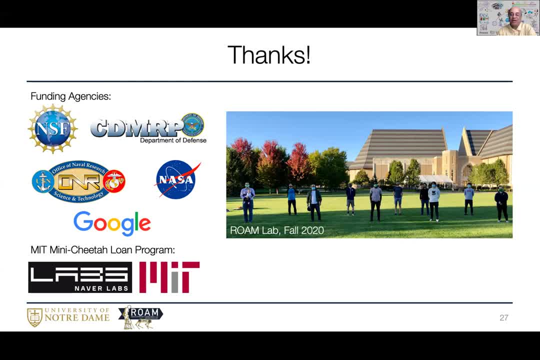 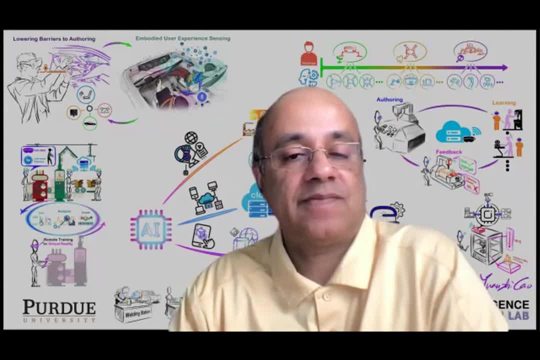 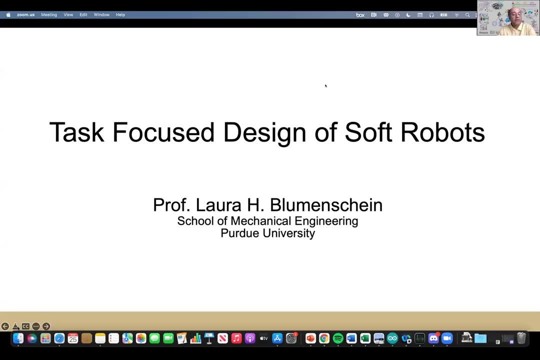 a nice discussion uh, now that we have a really interested group uh present in this talk. so, laura, you want to go ahead? sure, let me go ahead and share uh. let me know if you can see that. thank you, um, uh, okay, uh, yeah, so, uh, obviously, i'd like to also thank the organizers uh of this uh. 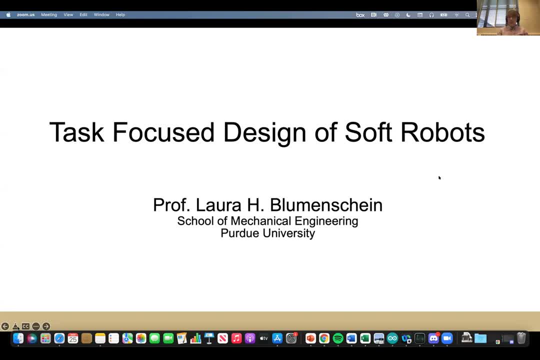 this webinar. uh, very glad to be talking about some of my interesting work and some of the more recent work that my students have been up to um, as well as just uh following uh patrick's excellent talk on. you know some of the wonderful things that i think you can do with web design as well, so 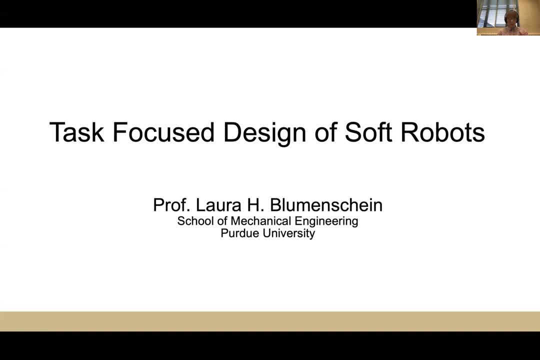 thank you so much for joining us today. thank you rigid robotics, now that you have these really established things, really established kinematics and dynamics and all of the modeling he was talking about. So I'm going to be taking a step back and let's go to kind of the infancy of another growing field, soft robotics, And within 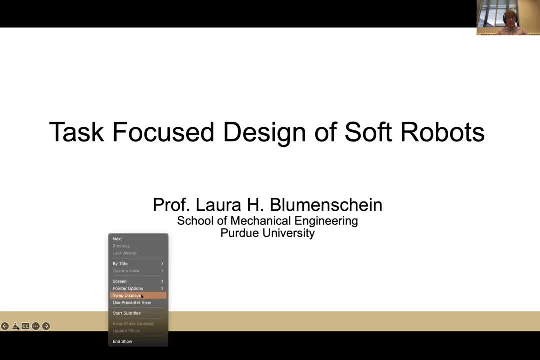 this field. I'm going to be talking about what I'm going to call- let me get a pointer up- what I'm going to be calling task-focused design of soft robots- Task- here is a word that I'm going to be a little liberal in using- where I'm just more talking about kind of fitting the morphology of 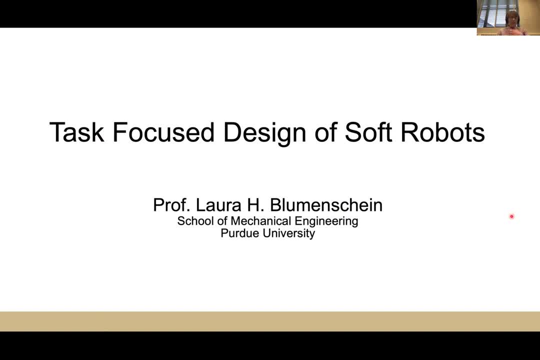 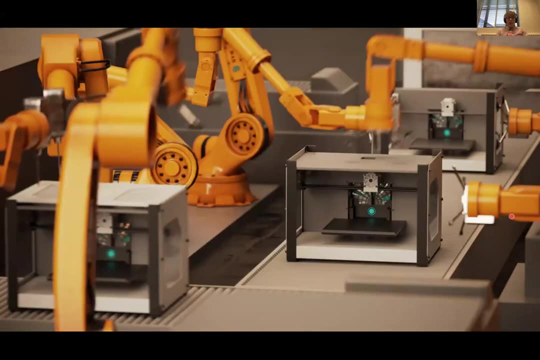 the robot to what we want it to do, And I have a secret sub header for this talk, which is: can you tie a robot in a knot? So look forward to that later in the talk here. So we've already seen a lot about kind of more traditional rigid robotics. Patrick had a great 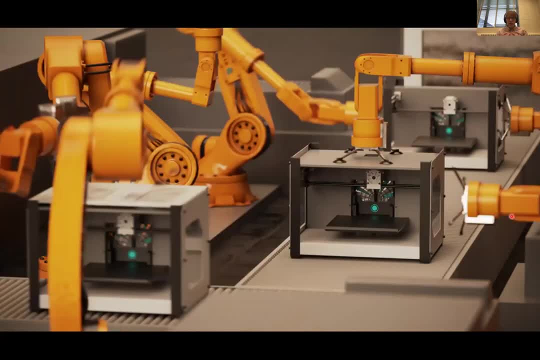 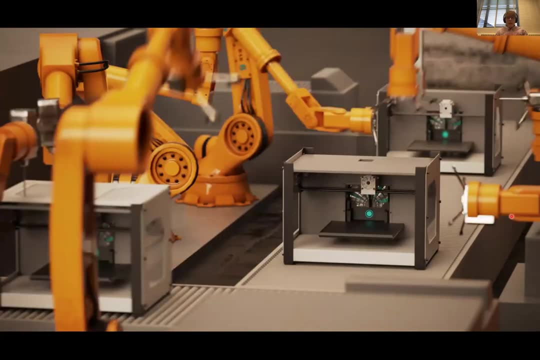 intro on. you know sort of where robots have gone As we're looking from traditional, you know factory robots like this, But I also like to start from that kind of perspective when talking about soft robots. right, So soft robots are. 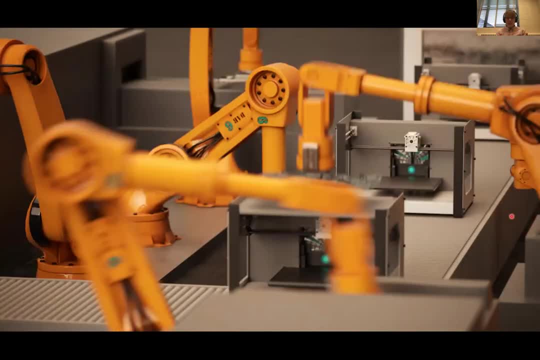 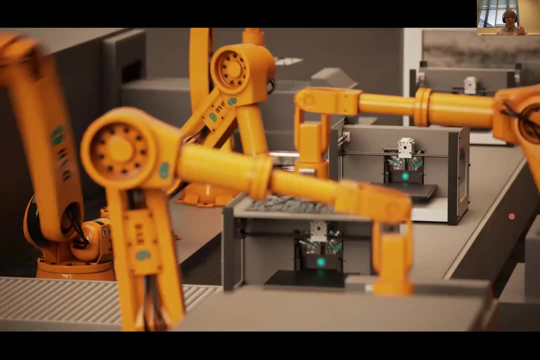 coming into this existing field of robotics, where we have a lot of robots that are really really good at doing precise repetitive tasks, And these robots are not friendly for humans to be around, but they are very, very good at what they do. 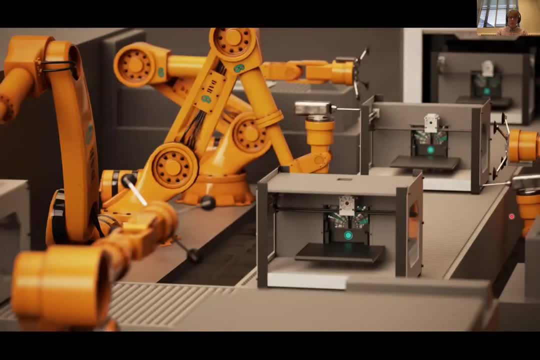 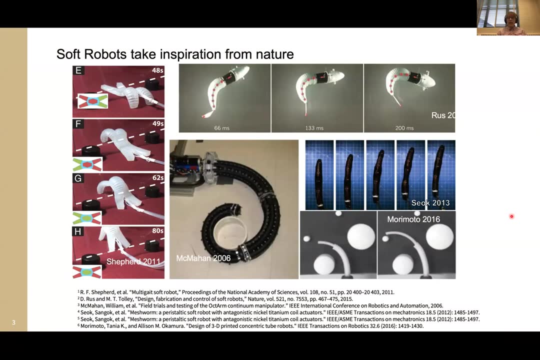 And so this is a great contrast, then, to what I'm going to be talking about, which is the field of soft robotics. So soft robotics, on the other hand, take a lot of their inspiration from nature. This is not my work here. This is the work of a lot of other, you know. 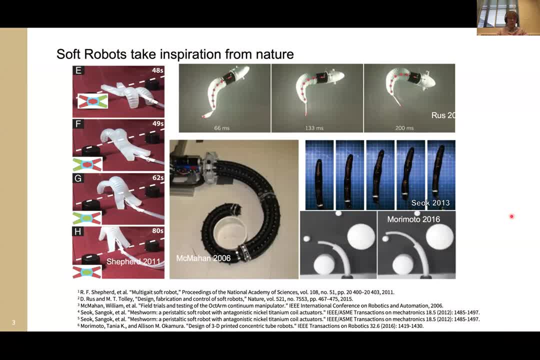 colleagues in soft robotics. But it's a nice representative slide I like to show of the vast variety of different inspirations that soft robotics has. So we've got little crawling robots, We have fish-like robots, We have, you know, like you know, like you know. 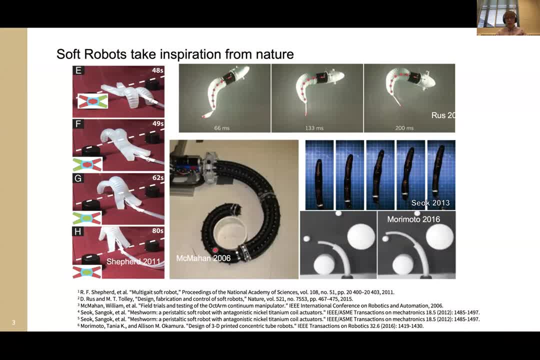 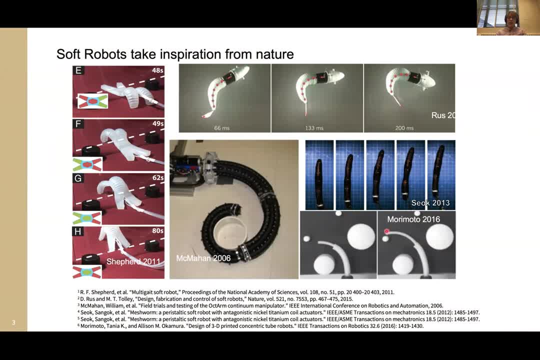 And then you know even systems actuators, that kind of act like a proboscis or something like an insect structure. And besides just having this inspiration from nature, what the underlying feature that all of these robots have is that they are changing their morphology through compliance, in order to change their behavior and adjust to a task. 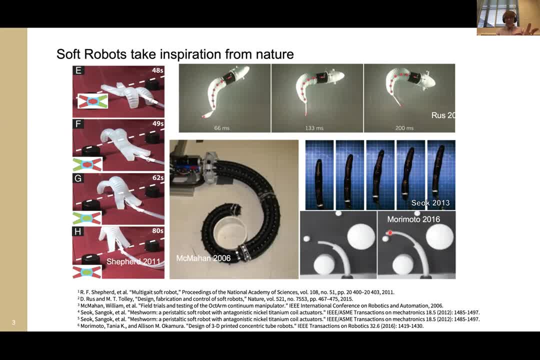 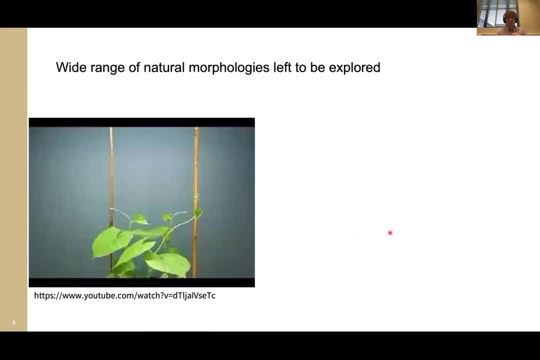 Now, a lot of the systems here, or all of the systems here, are taking their inspiration from kind of the animal side of nature, And so I think I'd you know. I'd like to just briefly say that there's a wide range of natural morphologies left to be explored which I think are really interesting for softer bikes as well. 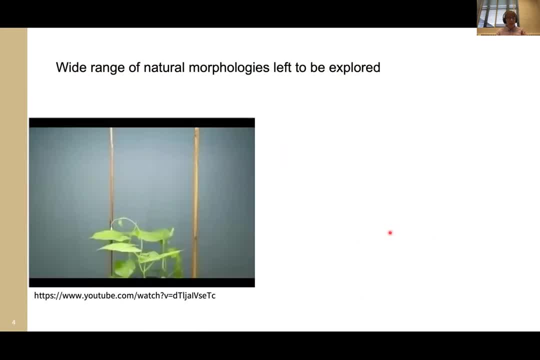 So one obviously near and dear to my heart is plants and vines. So we think about looking at this sped up video of a vine trying to find a point to grab onto its environment. It eventually does and it wraps around Again. this is a behavior. 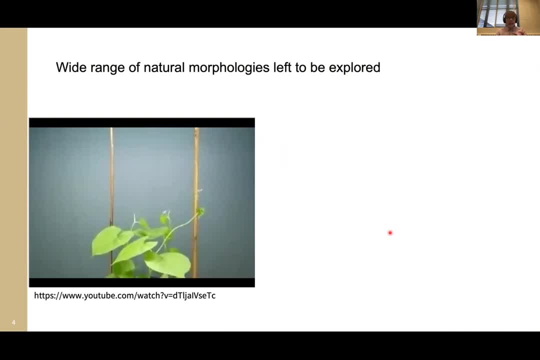 That is, in the morphology of the vine itself. It's not. There are some chemical changes when it actually does find this, this structure, to grab on to, but for the most part it's kind of just repeating this behavior and the morphology is what allows it to grasp this structure. 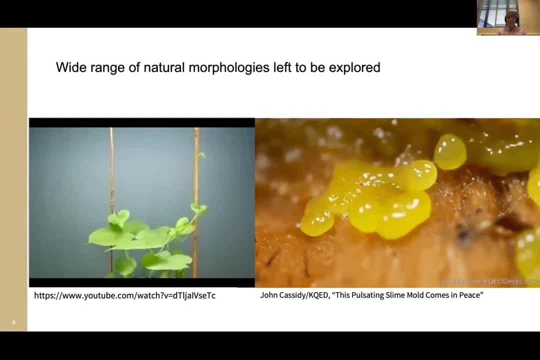 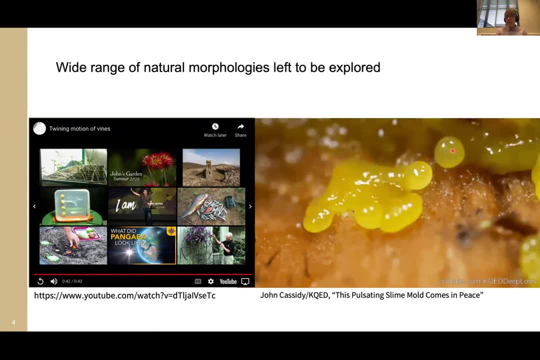 And then we even have very weird systems, right, these are slime molds. if you've never seen a slime mold before. There are very odd creatures, But they have Interesting movement capabilities based off of their bodies, And so this is just to inspire that there's lots of new directions to go. 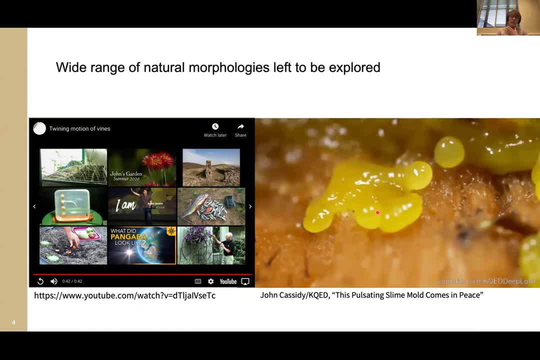 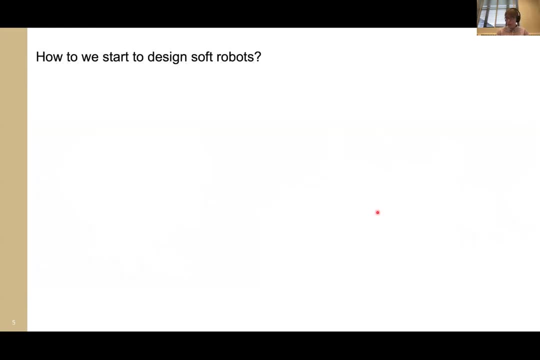 And this sort of building that we've been doing with software robotics into these kind of animal forms is not the only way we can go. Okay, So I'm saying that that's not the only way we can build software about. so How do I propose we do design software robots? What should we do if we're not just going to imitate animals or if we're not just going to 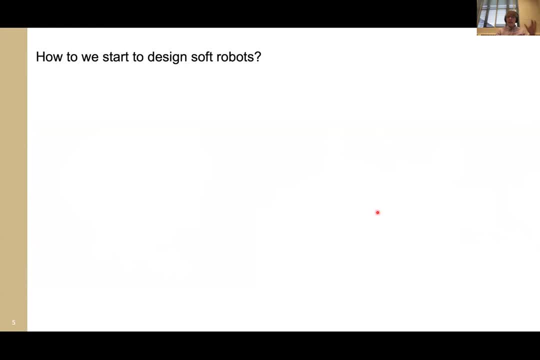 How do I propose we do design software robots? What should we do if we're not just going to imitate animals, or if we're not just going to kind of make rigid robots but compliant? Well, for me at least, it starts with acknowledging this high link between morphology and behavior of software robots. 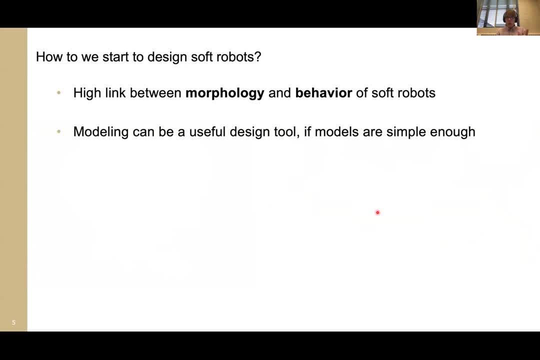 And, as a result, our primary tool that we're going to look at using is modeling, As long as our models are simple enough- Patrick talked a lot about this- and model predictive control as well. Patrick talked a lot about this and model predictive control as well. 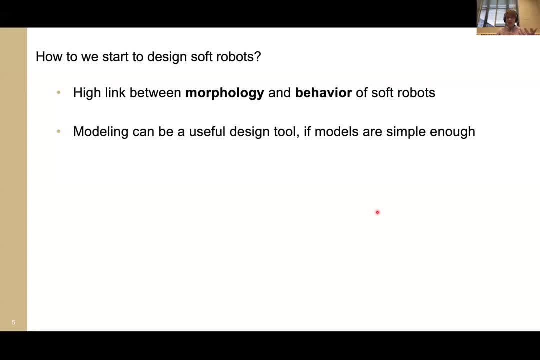 How the complexity of the model changes how you approach things. but for us, if our models are simple enough, that makes a modeling and good design tool. And the models I'm going to look at specifically are models that pull from geometric constraints, And by using these geometric constraints we're going to build simple kinematic building blocks. you can think of this akin to the joints that you have in a rigid robot. 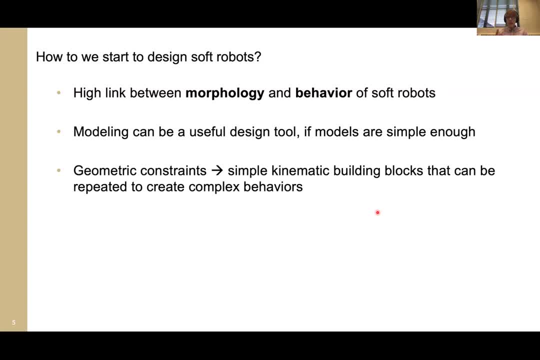 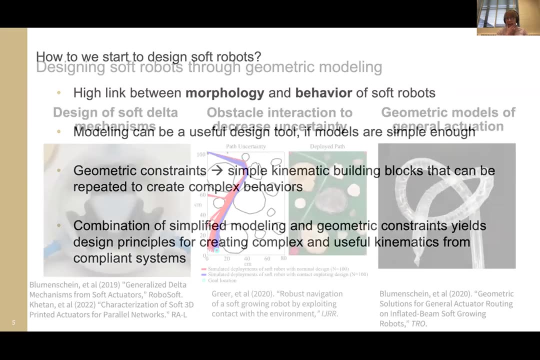 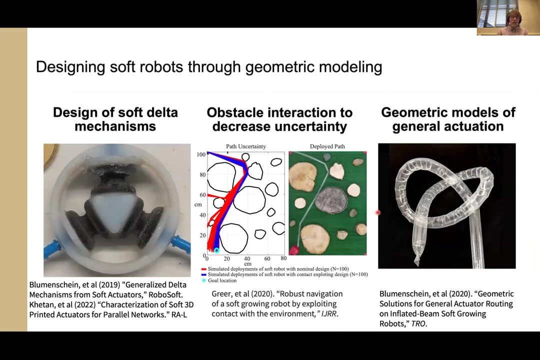 And we're going to use these building blocks Repeatedly to create complex behaviors, And the goal here, then, is that this combination of modeling and geometric constraint constraints can yield design principles for creating complex and useful kinematics. Okay, so, with that, as a sort of intro to the work I'm going to be talking about, Here are the three little projects I'm going to go through, that kind of build off of this designing software robots through geometric modeling. Okay, so with that, as a sort of intro to the work I'm going to be talking about, Here are the three little projects I'm going to go through that kind of build off of this designing software robots through geometric modeling. Okay, so, with that, as a sort of intro to the work I'm going to be talking about, Here are the three little projects I'm going to go through that kind of build off of this designing software robots through geometric modeling. 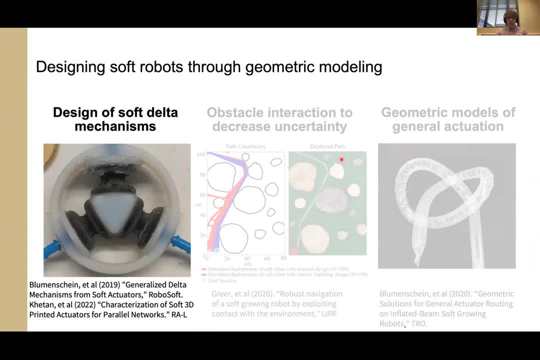 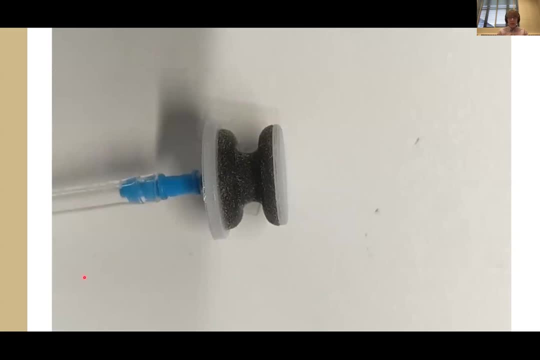 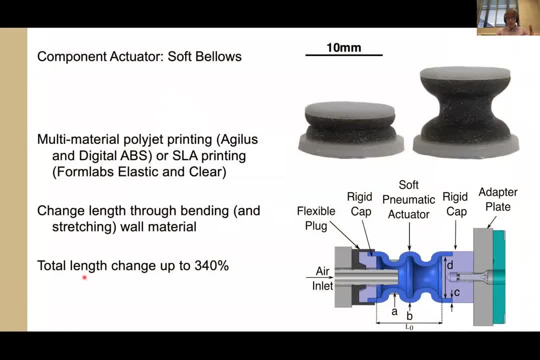 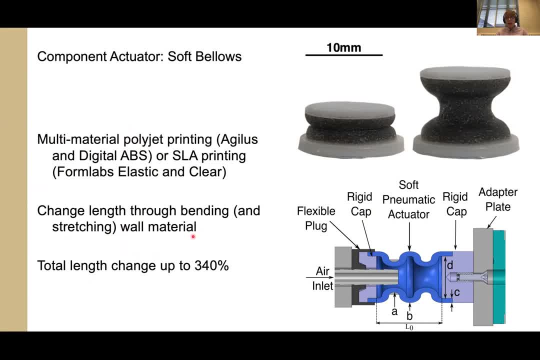 as opposed to primarily through stretching of the wall material. The reason why this is a big benefit is that these elastic materials can have very nonlinear models when we talk about straining them. But here through bending, we're not creating a lot of strain of the material itself. we are mostly creating strain in the actual structure. 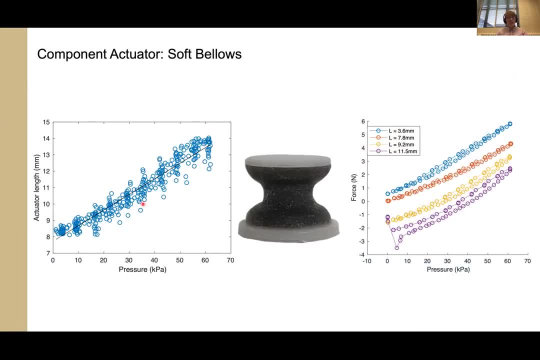 As I said, to cut to the chase, we get very nice linear behavior out of these bellows. So here is pressure versus length over here we have pressure versus force at different lengths, And so we have this nice linear actuator based off of pressure. 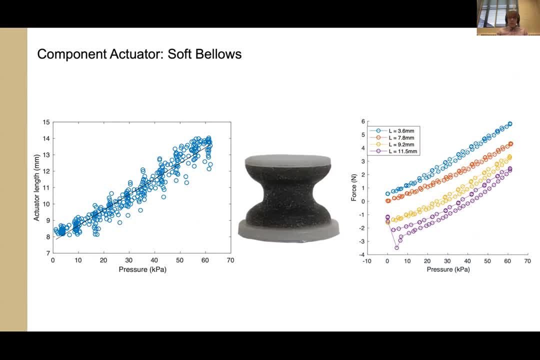 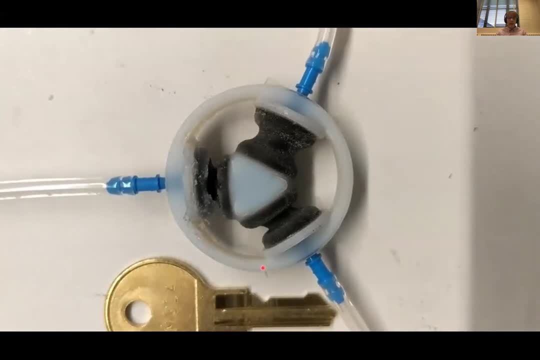 And so immediately we think let's build something more complex with this. So let's take three actuators, let's put them into a structure together And we can get a little complex structure. This is the compliant delta mechanism. If you've ever seen or tried to work with the kinematics of parallel robots, you might know that usually they're a lot more complicated than this. 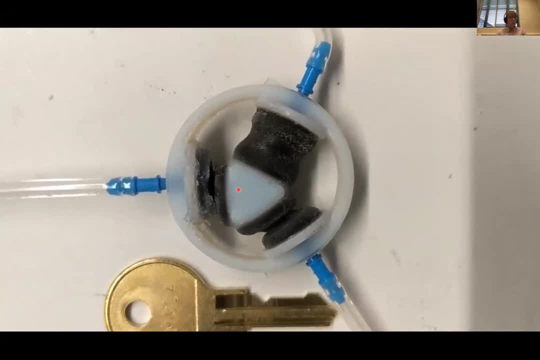 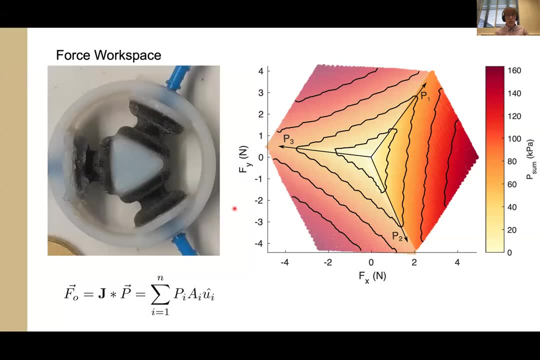 But here we just turn on different actuators and we get this center point to move about in space. So go ahead and put that. So where does the modeling come in there? Well, I'm going to cut to the chase, cut out kind of a lot of the experimentation in math. 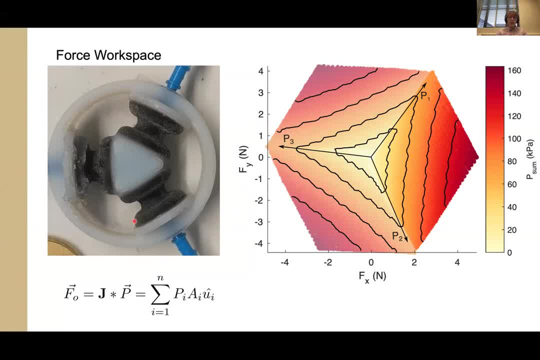 Just to get to the results here. But when we look at this system- and we just talked about the force, workspace, so we're going to hold this point in the center constant, The output force that we get is just a linear combination of the forces of the actuators we have. 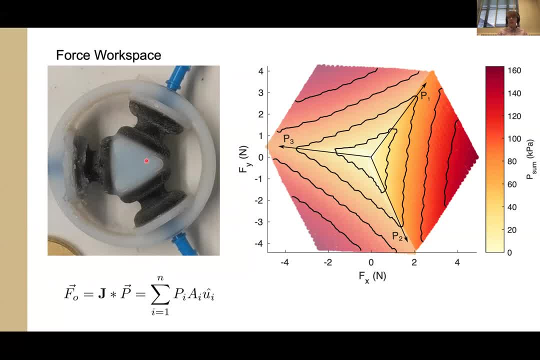 This makes sense because this is, you know, just a force balance equation And we can see that essentially we get preferential force direction aligned with the actuators. So it's a little easier. we have less total pressure. we need to get to a point aligned with one of the actuators, as opposed to in between the actuators where they kind of have to work together and we get a little bit of loss energy. 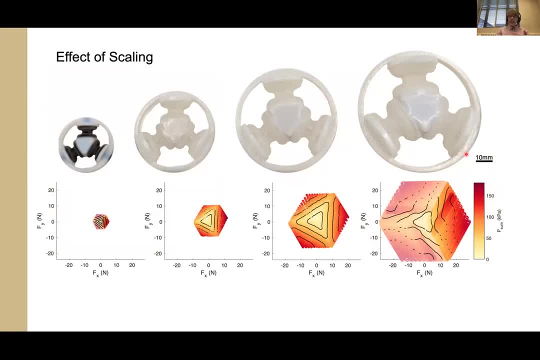 This scales very well. so we can take the same design and the same model for our actuator and scale it up up to 250% in size, And if we look at the max force output we get, we can see that that scales as well. 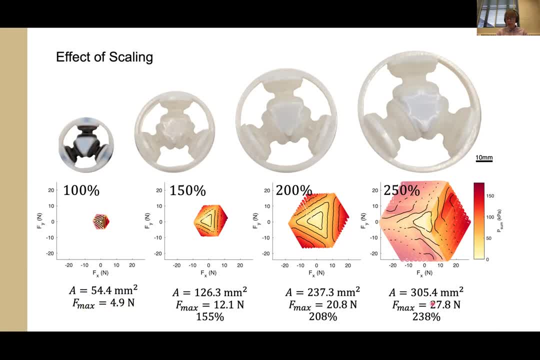 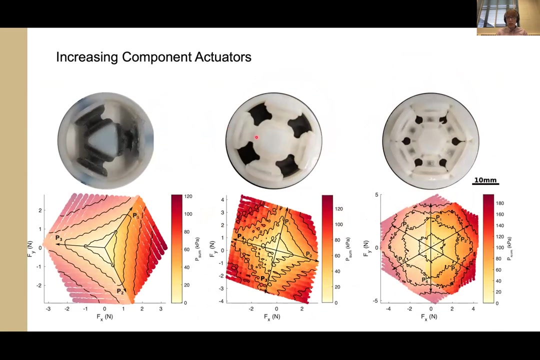 So here we get a max force of 4.9 newtons And here we get 28 newtons of force out of 250% increase in the force. So that's nice as well. And then we also get really nice behavior if we just start adding more on so we can over actuate this point in the center. 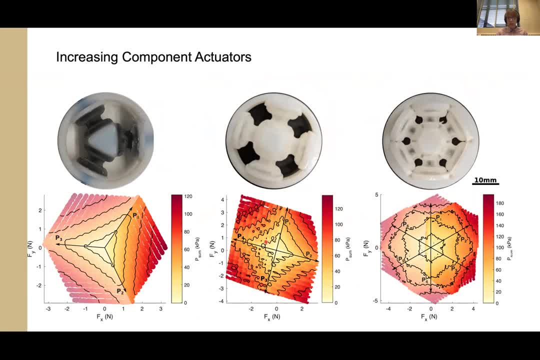 And we get well predicted behavior from just linearly summing the forces. so again, Here is a four actuator and a six actuator system where we're measuring out these forces in the directions as, and the sum of pressure required to get to those forces. 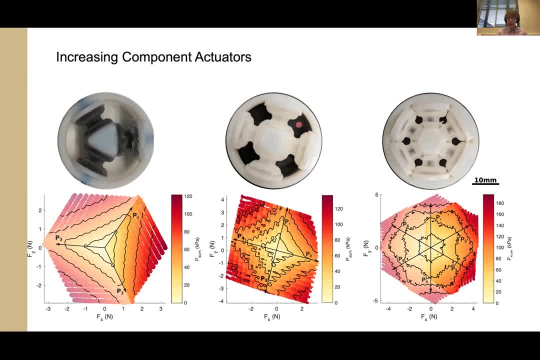 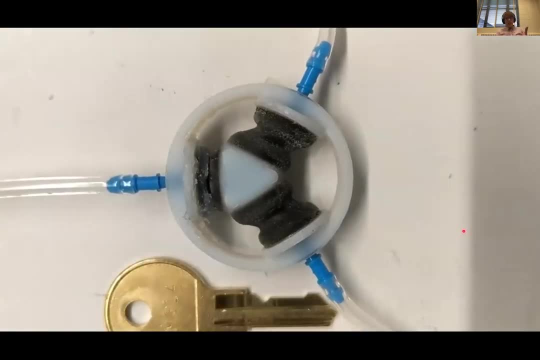 And we can see essentially the benefits of adding more actuators in. is we kind of smooth out the force distribution Over our workspace a little bit? Okay, I've been talking about force, though, but when we go back to this video we see this point actually moving around in space. 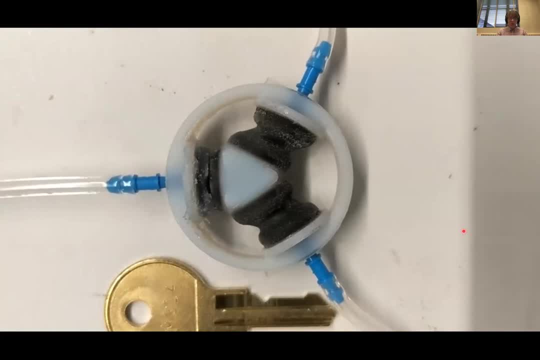 So what if? what, if we want to model that part of things, Can we just use this linear combination model? Well, the answer is yes and no, And it kind of comes down to what we're seeing here right, which is sheer. So we're sharing these actuators in addition to linearly summing. 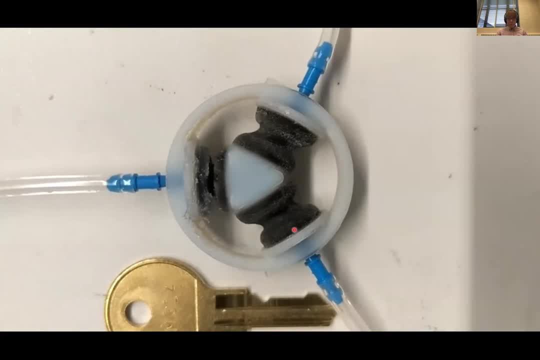 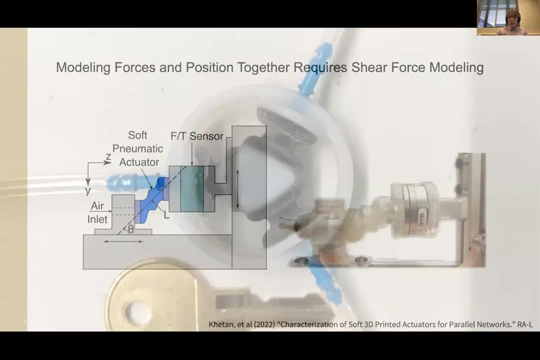 And then we're going to add in the shear. And so now we're going to model both forces and positions together by adding on some sheer force modeling of the single actuators: again, we're only going to be looking at the single actuator as our building block and we're going to use that to predict the behavior. 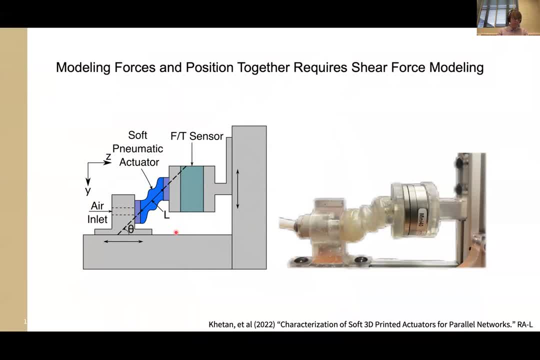 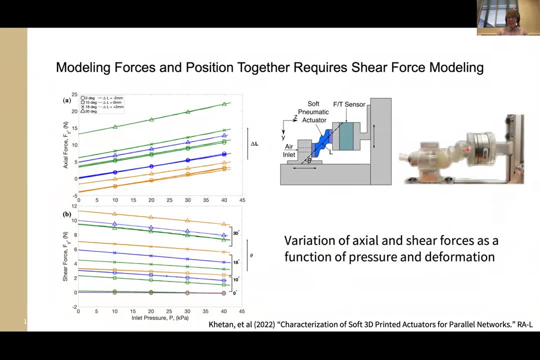 of multi actuator system. Okay, So in this case, if we take this system, we deform it in at various angles, very sheer angles, various length changes. We get out a lot of nice data here which shows us that we stay linear with pressure, which is very nice. 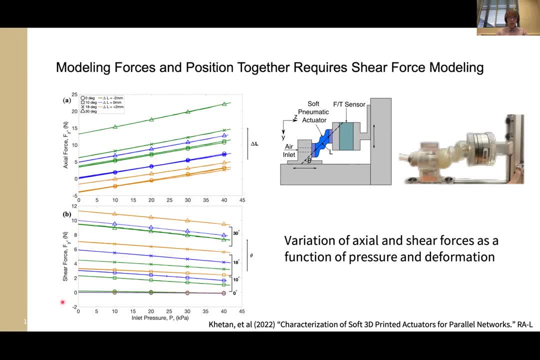 But our kind of relationship with pressure, based off of our sheer force and our axial force, changes, based off of our length, change. So that's color here, or the angle of sheer that we have, which is our symbols here. So we get a variation of axial and sheer forces as function of both the pressure and the deformation. 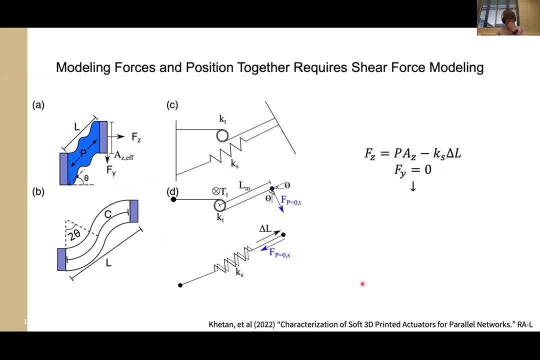 To model this again. we want these to kind of simple geometric models, And so we're going to take two approaches. we're going to have one part of our model that is based off of the sheer angle changing kind of the pressure Or, sorry, the area effective that the pressure is acting on, looking at it as this sort of deforming tube. 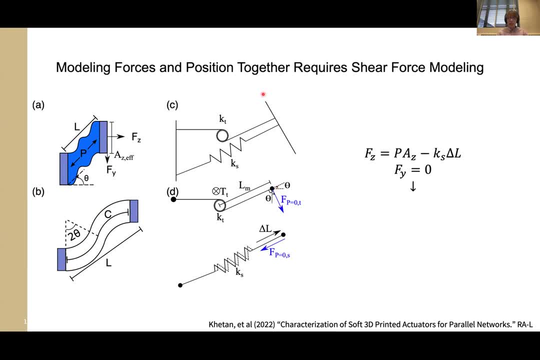 And then we have one which is sort of this linear combination of torsional and linear springs to describe the deformation behavior. So if the model we had before was something like this, where we had just forces in the linear direction based off of pressure and scaled based off of our delta L, 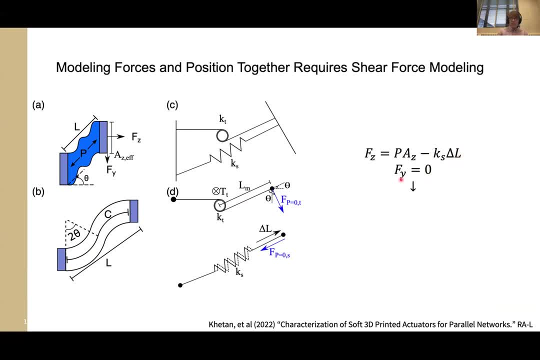 With no consideration of sheer. our new model looks something like this. So it's not linear anymore. we've got some theta squared and delta L times theta, But it's still relatively simple overall with our linear stiffness and our torsional stiffness and then our pressure. 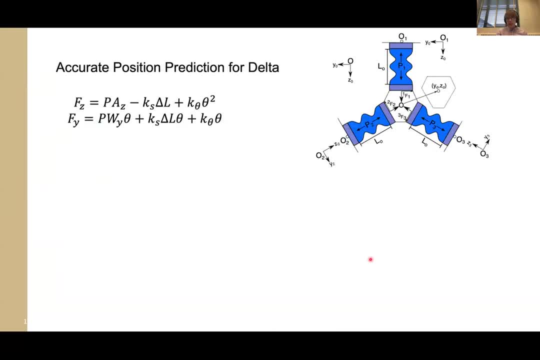 And if we take this model and we build our delta again here, And if we take this model and we build our delta again here, Now we can look at whether we can predict the output position based off of the input pressure. And long story short again, so I can get on to some of the other topics. 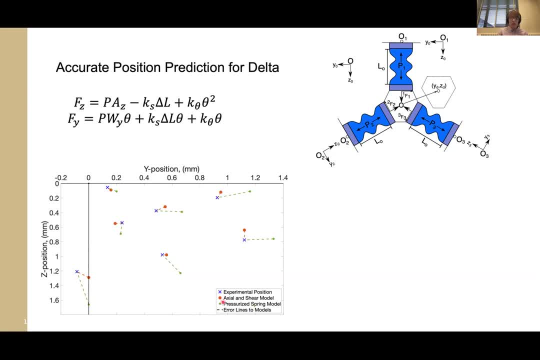 The answer is yes and it works better than just our pressurized spring model from before where we're just considering the axial forces. where we can see here the orange dots are our new axial and sheer model, the blue crosses are where the position actually ends up in the green dots for our previous model. 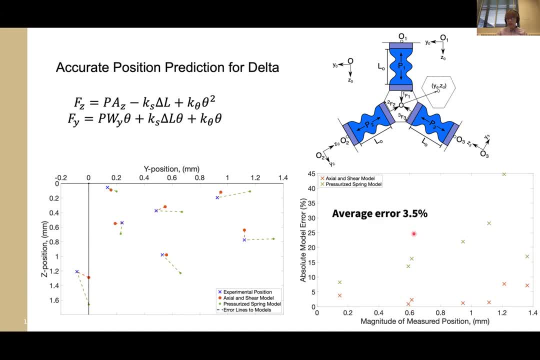 And so we get an overview. Overall average error of about 3.5%, which is really really good for a software robotic system, if you've ever worked with a software robotic system. So this is how we would then build from building blocks like single actuators. 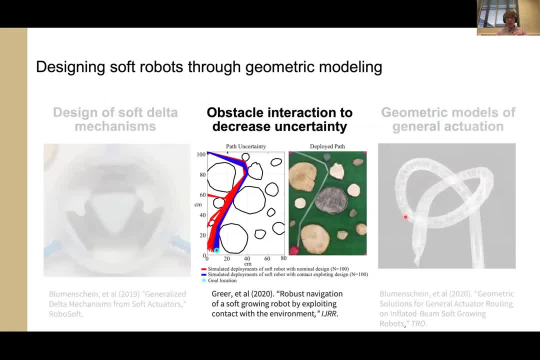 What if we're trying to describe the behavior of a full software about, can we take this approach of kind of compartmentalizing and tearing apart the pieces? What if we're trying to describe the behavior of a full software about, can we take this approach of kind of compartmentalizing and tearing apart the pieces? 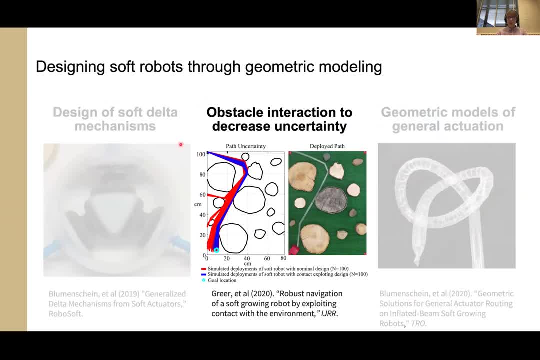 And building up a geometric model like that. So to answer that question, let's go on to the second topic which I've told here: obstacle interaction to decrease uncertainty, And the theme here is going to be kind of looking at heuristic behaviors of soft robots in order to build these building blocks of our behavior. 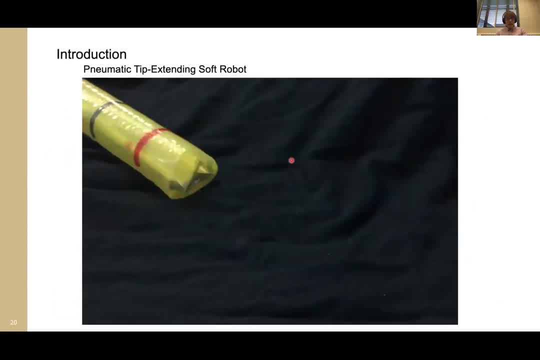 So, to describe this section of the next section of work, I'm going to have to introduce the growing robot we have here. So this is our growing robot. This is the the kind of main Interesting new degree of freedom that we have with the growing robot, which is this extension, using pressure and growing from the tip. 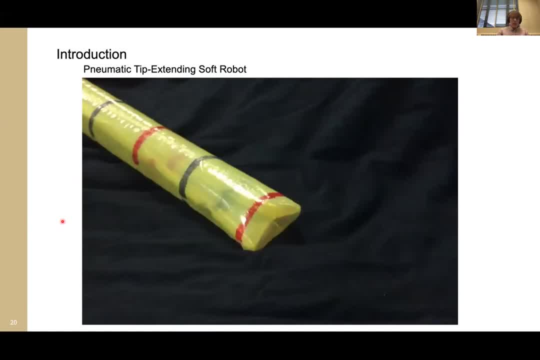 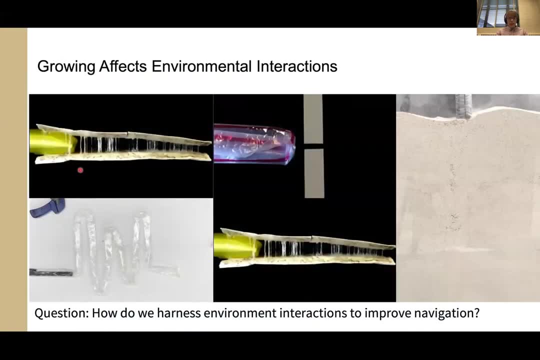 And overall the. the body of the robot is very akin to a continuum robot where we have this long, slender body. If you're unfamiliar with the growing robot- Some kind of going back to this- let's click on some of the videos here. Some of the can't seem to get these videos play. 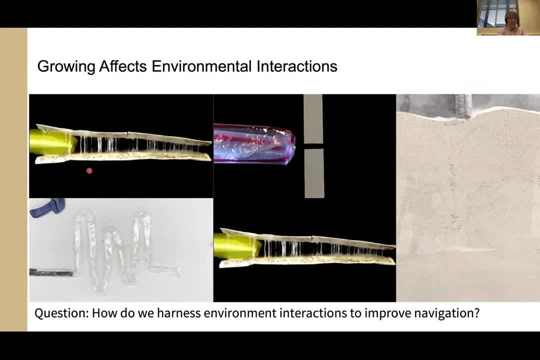 So some of the benefits of the growing robot here is that it has a lot of nice interactive behaviors with the environment. So if these videos would play, you would see we have. the robot is able to grow through these incredibly sticky sub structures. it naturally navigates around bends. 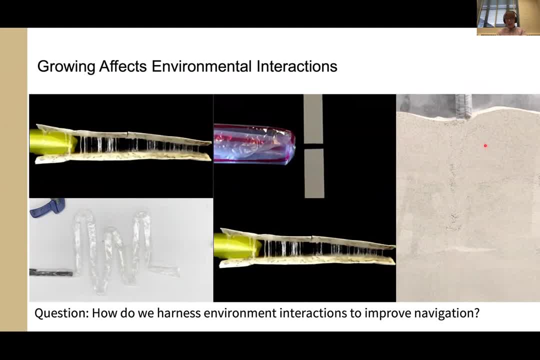 It grows through very small gaps and it can even do some digging. It can even do some digging If we give it a little bit of extra air pressure. So a question we might have then is how do we actually harness these environmental interactions? 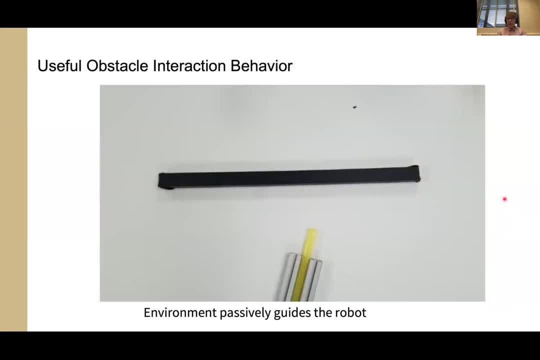 And we can do that by observing a really nice heuristic behavior when we interact with an obstacle in our environment. So we grow into an obstacle, The tip of the robot moves tangent to the obstacle And then we have a pivot back At the base, wherever we most recently contacted an obstacle. 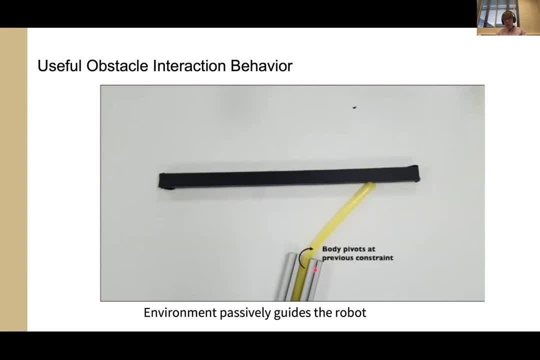 So again, tip grows tangent to an obstacle, Pivot at a previous constraint and we grow until we leave the obstacle, which point we just kind of follow whatever direction we're going. So this means that our environment will passively guide the robot. This is a lot of times- if you've heard of this in software box before- people refer to this as morphological computation. 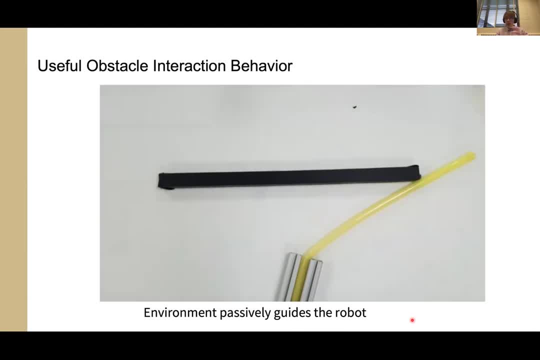 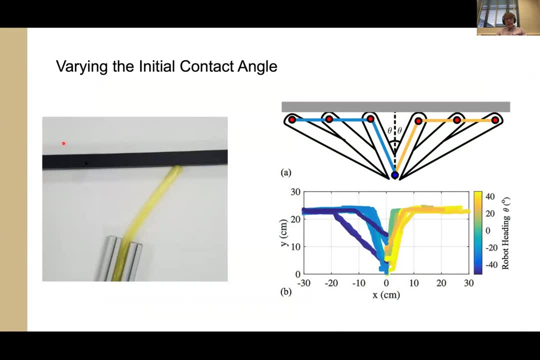 To do that. it is about to test an something. It really just means we're seeing an interesting or potentially useful behavior from the natural response of the robot. The heuristic we come up with is very simple: It's just depending on the initial contact angle, right? 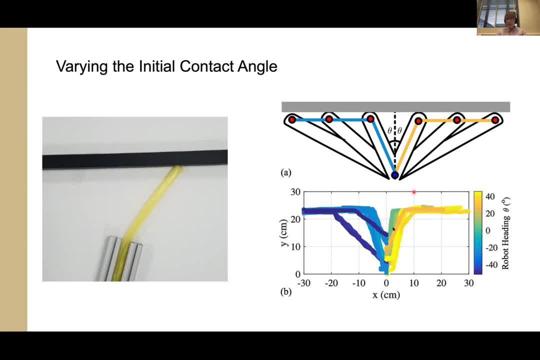 That's gonna tell us which direction we're going to grow. So if we hit it at greater than 0 degrees positive interaction angle, here We'll go 1 direction, And if we hit it at greater than 0 degrees positive market angle, we're going to see an difíautic interaction here. 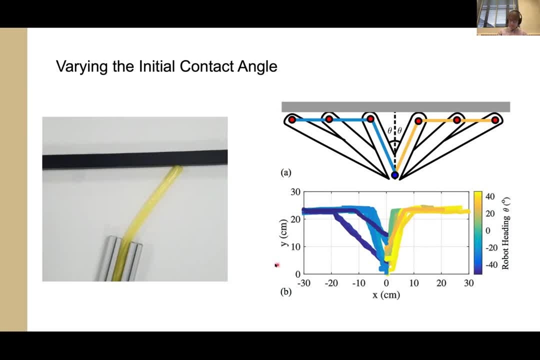 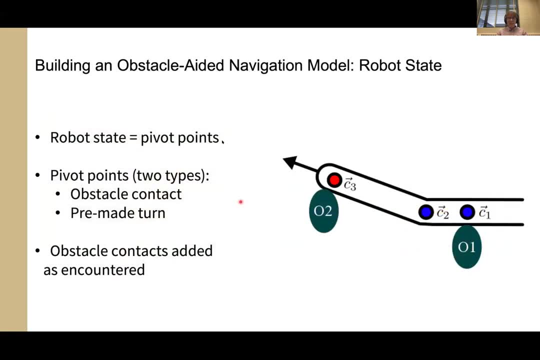 But we're going to also increase the speedcen. a negative interaction angle will go the other direction, And that's that's essentially it for the model. Now, this gets a little more complicated when we think about all those previous contact points we have, but not too much more complicated. So we just need to define these pivot points. 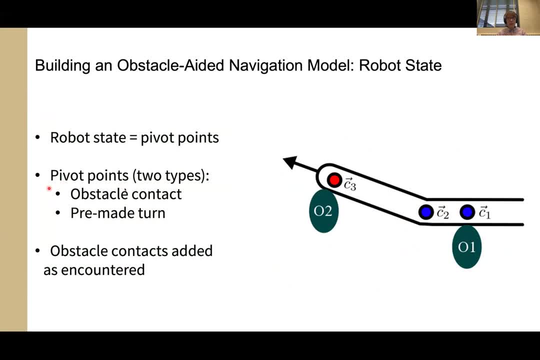 where the robot could pivot about. There's two types we'll define: ones that are based off of obstacle contacts, which is what I've shown previously, and then ones that are made based off of pre-made turns that we build into the robot ourselves. So that's something akin to this. 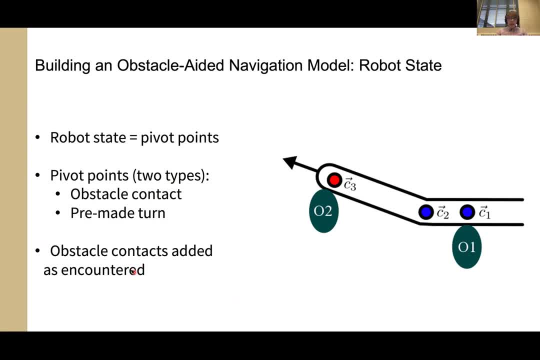 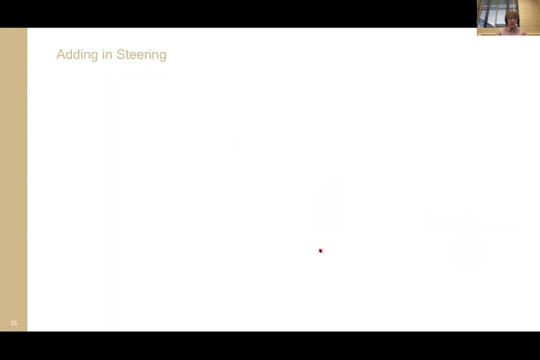 And then, as we have more obstacle contacts, we're going to add those into our potential pivot points or our potential obstacle contacts that are deforming our system like this. So just talking about the steering rule, quick, how do we actually do that? Well, we're just shortening one side of the material. 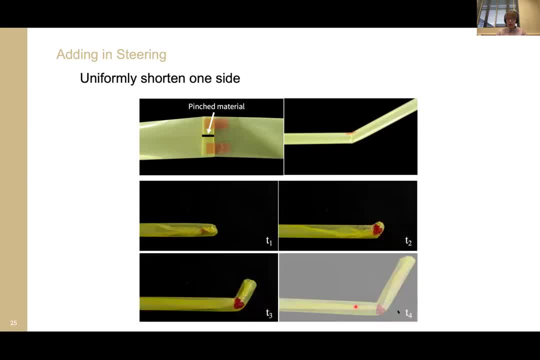 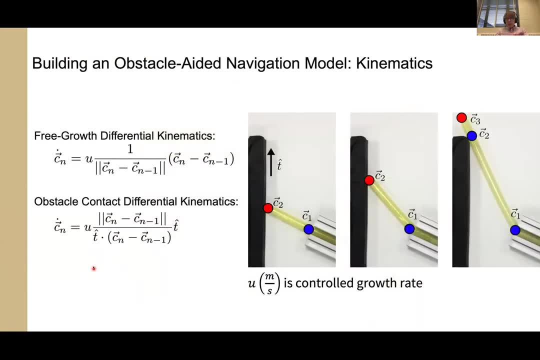 which gets us a turn as we go. So that's all we mean by those kind of design pivot points, So obligatory math slide. this is what the kinematics come out to then, Just in terms of what we see. we have one kinematic equation to describe when we're 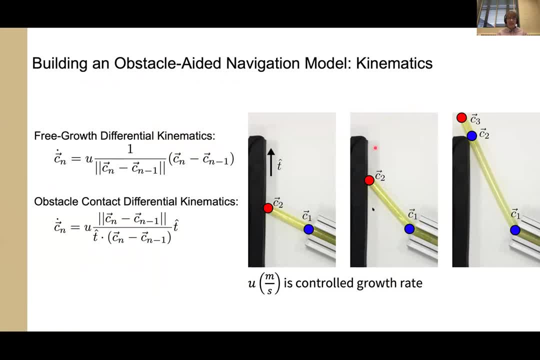 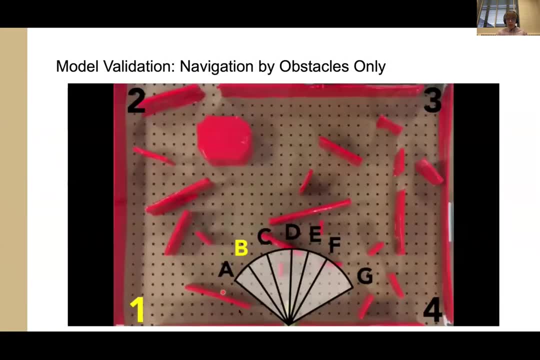 not in contact with an obstacle. and then another one describes following the tangent of that hockey stick during the selection, And this is more something we can finish up as if you hit a ten-point circle. but we have, you add two more �เอ to very, very low. 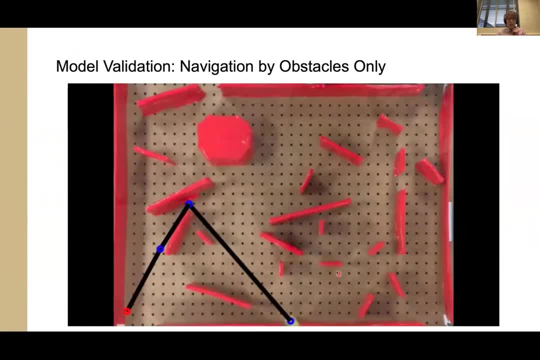 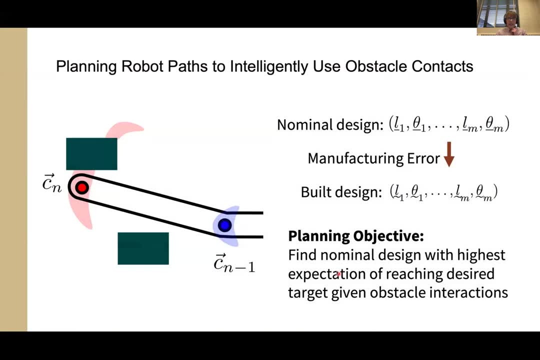 fineness Grandma's way right, because the answer to most of the ideas is: we don't have any KYRST move wings, but we can still affect the horse. So with that in mind, we have an example of how people like Michael radar build a. первый kid within the quadoux wheel section safely. Now what we know is that these kids we've had over two, three years can, craving certain kinds of alters, effectively identify with mimics in the记. besides, when we make decisions or magically run out of time, to have this bite combination To reduce limitations on disabled kids. 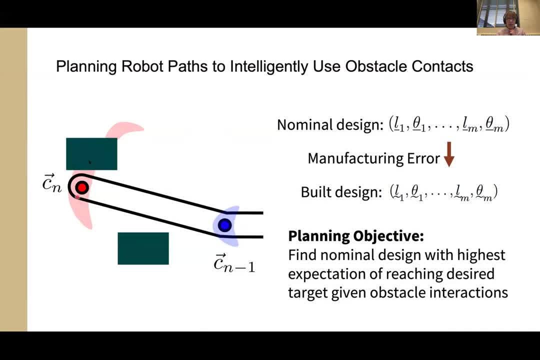 have some amount of error potentially in our robot And if that error gets big enough we can have this kind of chaotic bifurcation where the behavior of the robot naturally goes in the direction we don't intend it to. So we want to plan in a known environment to reach a desired 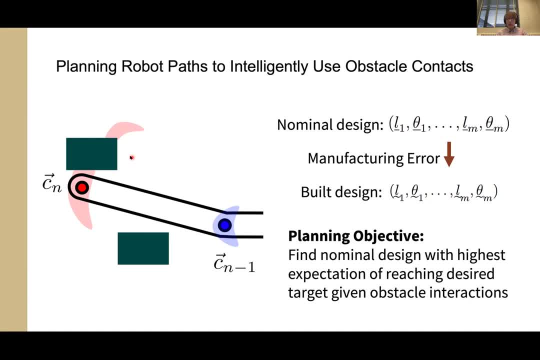 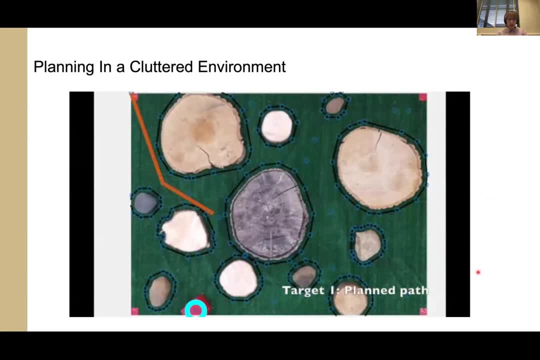 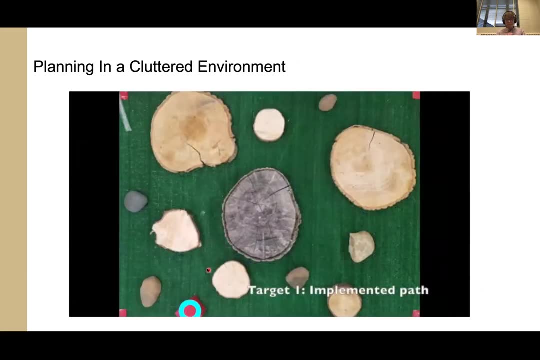 target with taking this potential uncertainty into account. So the results from that look something like this where, if we've got a target location, we plan out a series of turns and a series of intentional obstacle contacts that get us to a desired target in space with some amount. 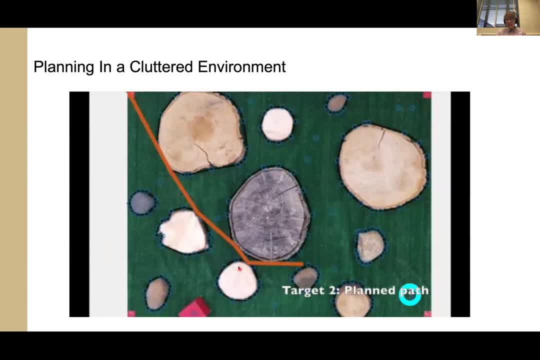 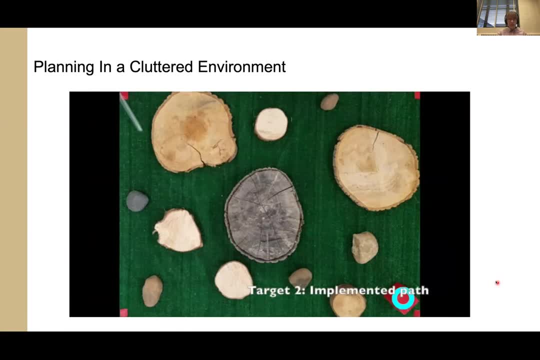 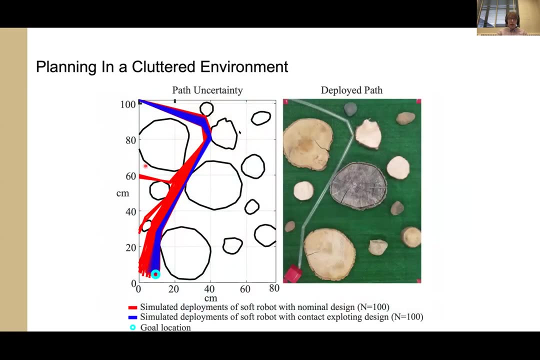 of accuracy. You know this is all open loop so there's only so accurate the target hitting can be here. But again, this is very, very nice results for just a kind of a tube growing into space. And you know, if we simulate this we can see that if we compare this to something like 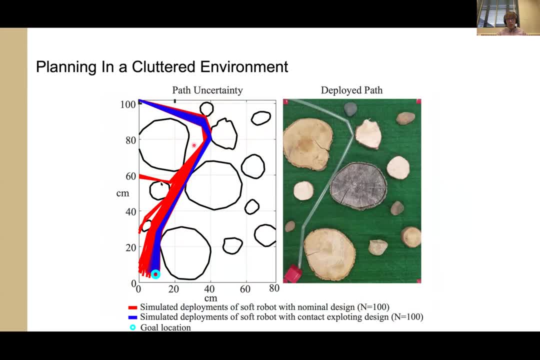 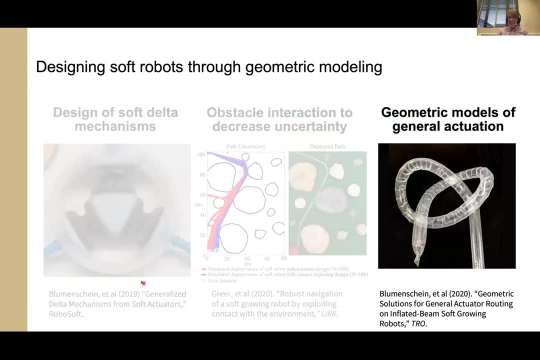 traditional robot planning, where we avoid obstacle contacts. intentionally using obstacle contacts is reducing our uncertainty overall. Okay, to keep inside of the 25 minutes, I'm going to move on to this last topic here, which is my promise. can we tie a robot in a knot? I've already kind of given away the answer with. 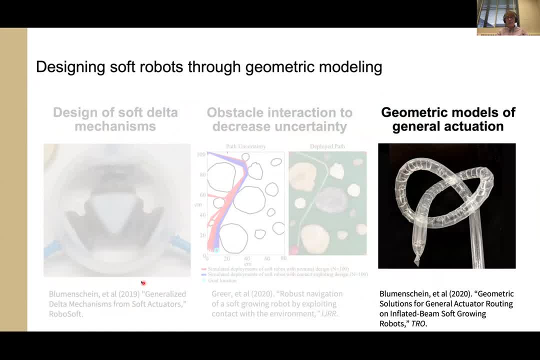 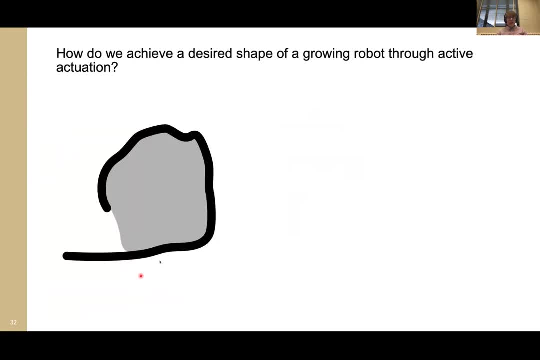 that picture there, but let's get started. So let's get started. Let's talk about how we actually get to tying a robot in a knot. So we're going to be with growing robots again, but now we're going to add active actuation to get a desired shape in space. So maybe we want to wrap around an obstacle. 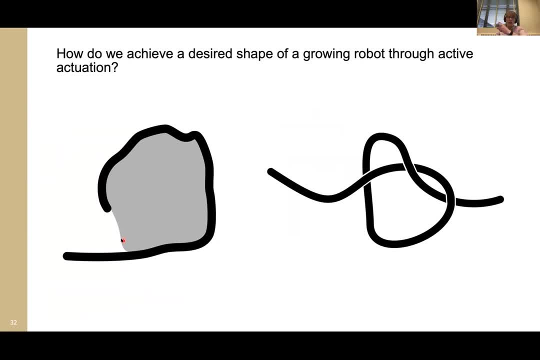 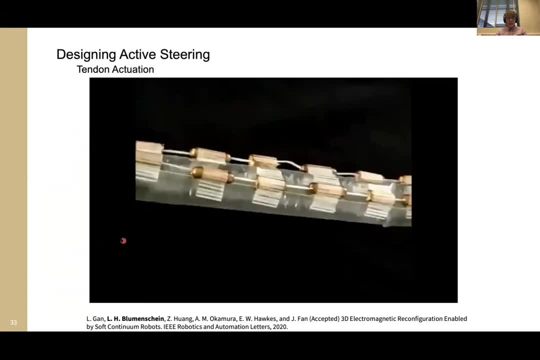 or, as I said, maybe we want to do something like tie a robot in a knot so that we can grasp onto something in our environment. The small addendum to be able to do this is we need some way to actively control our shape. So the two ways we do that is either through tendon actuation. 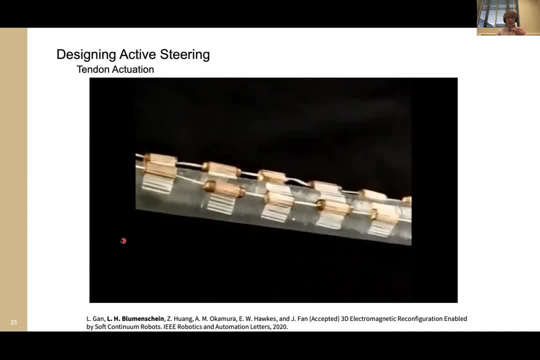 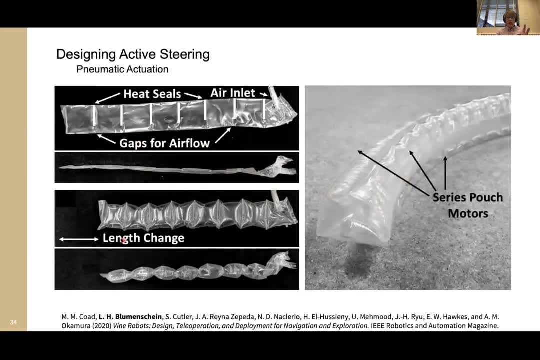 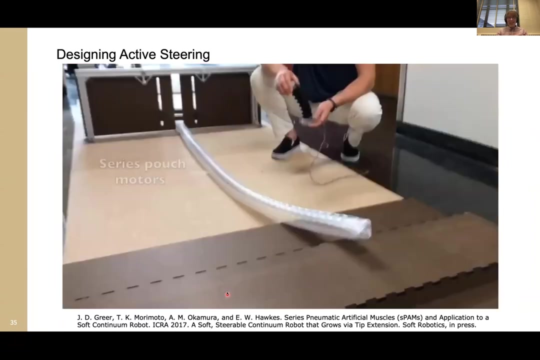 which is shown here, essentially pulling a string and collapsing these little pieces along the length to control a shape or pneumatic actuation series. pouch motors is what we have here, which essentially gets shorter as we add air in And this allows us to steer the robot in space. 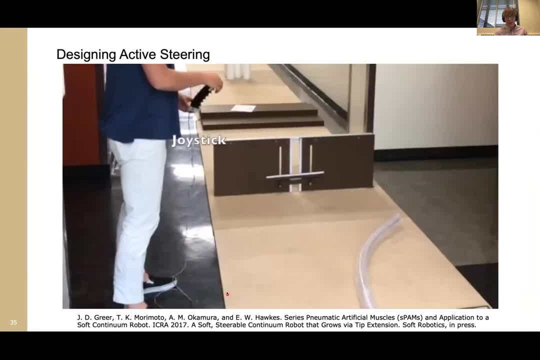 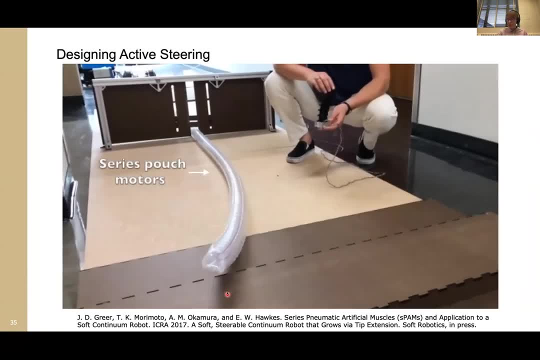 This is a previous colleague, Margaret Code, who I believe is in the audience right now, who is steering the robot here, But we are using the pouch motors to kind of steer it back and forth. So we want to create more complex shapes. So what are we going to do? 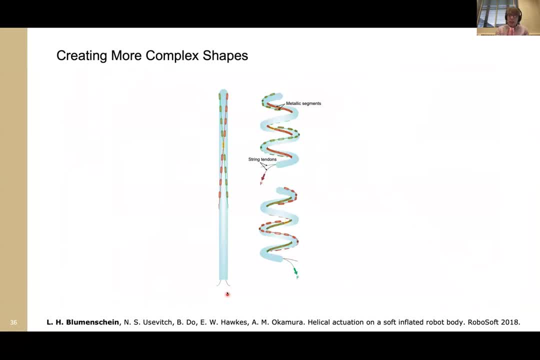 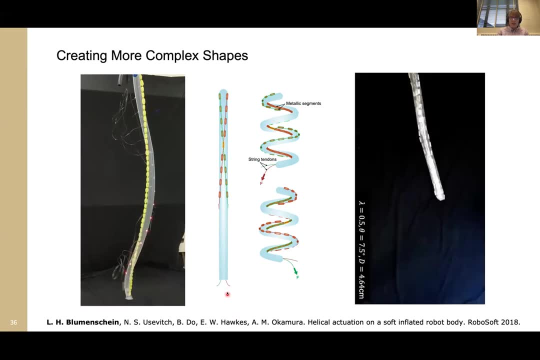 Well, we're going to start with a again kind of building block, And our building block here is going to be a helix. It's pretty easy to make a helix. All we have to do is just wrap our actuator in a helix around the robot and we can get a helix out. 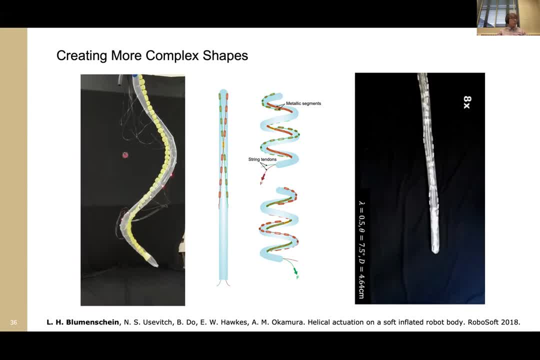 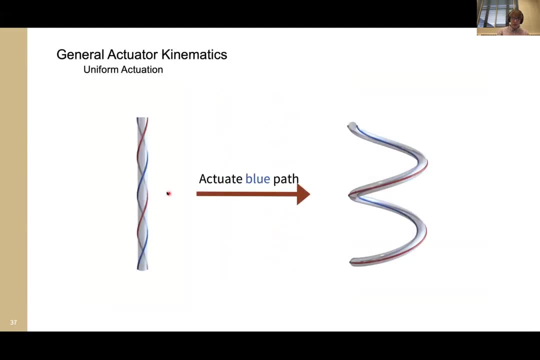 And the reason why we're going to use a helix as our base shape here is because it gives us a variable curvature and a variable torsion which we then can use to make a wide variety of shapes. But we're not done by just choosing a helix. We actually have to figure out the kinematics here. 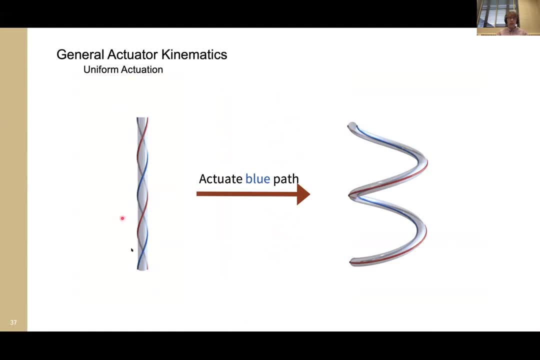 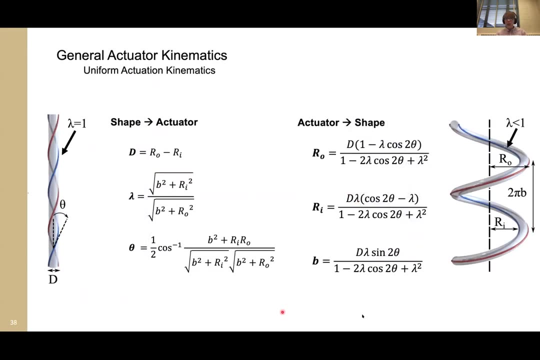 So we want to know, based off of this initial shape of our actuator, defined by some variables, what is the shape of the robot? we get out Long story short again. just cutting to the obligatory math slide, we're actually able to find closed form kinematics for this, which is really nice. 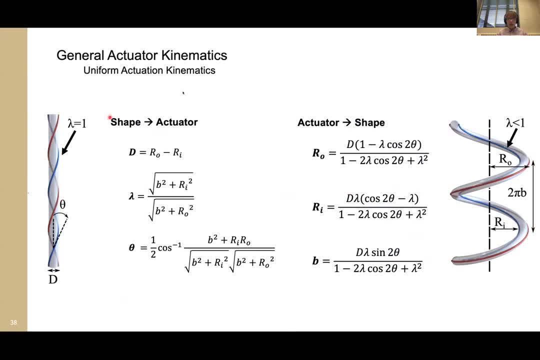 Now we've got three equations on each side. Again, you might think of these as sort of your inverse kinematics and these as your forward kinematics. Now, even though we have three equations, we don't have three degrees of freedom. This one here is kind of our actual actuation. 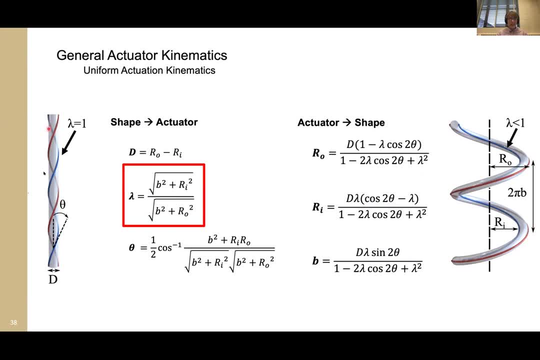 This is changing how long this line. that's what we're pulling on, if we are actually actuating one of those tendons I showed earlier. But these kinematics work well. We're able to predict the shape of helices that we construct. 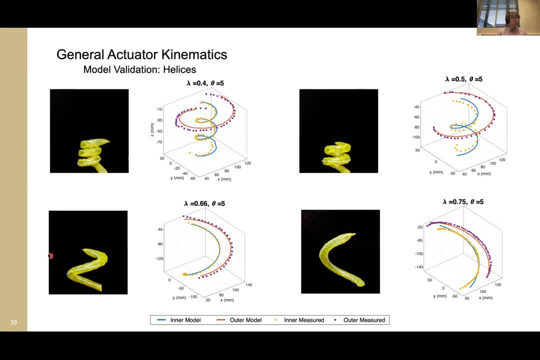 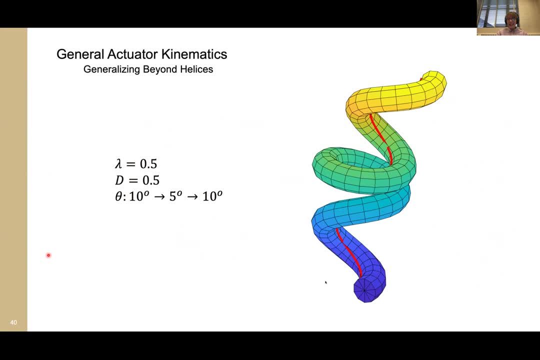 measuring their shapes and they match well to our model. So now we're going to take this and we're going to generalize it beyond helices by just stacking a bunch of helices together, So we're going to change one of the parameters over the other. So we're going to change one of the parameters over the other. So we're going to change one of the parameters over the other. So we're going to change one of the parameters over time and we're going to get a more interesting shape. 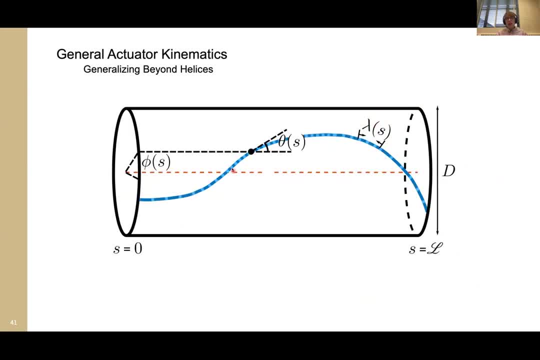 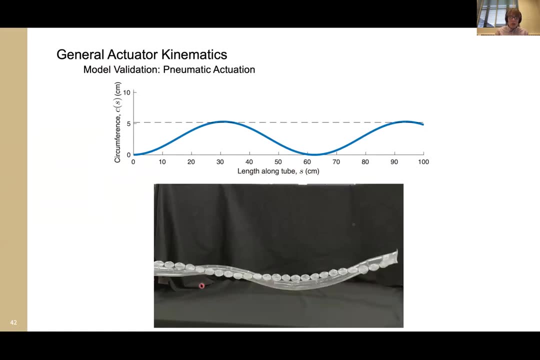 And if we do that at a fine enough resolution, then this interesting shape can become a wide variety of shapes that we want it to. So in the interest of time I'll briefly show kind of the results here. So this is one shape that we've got. 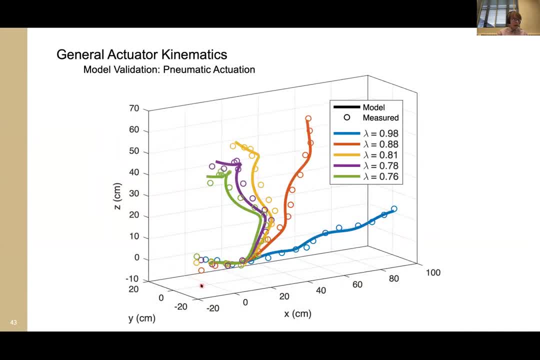 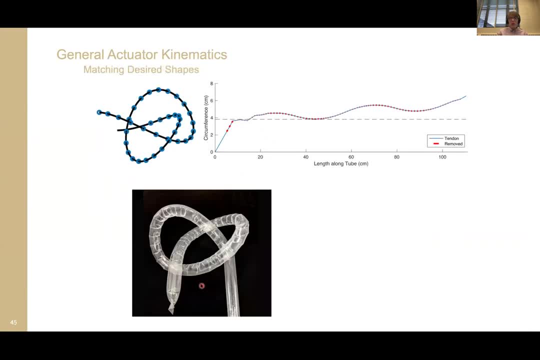 And again, our model predicts well that shape let me go to, so we can use this then to design with a lot of kind of maybe a little, a little less intelligent optimization than Patrick was talking about, but using some of the optimization toolkits we can find a shape that allows us to match a shape that is desired like something. 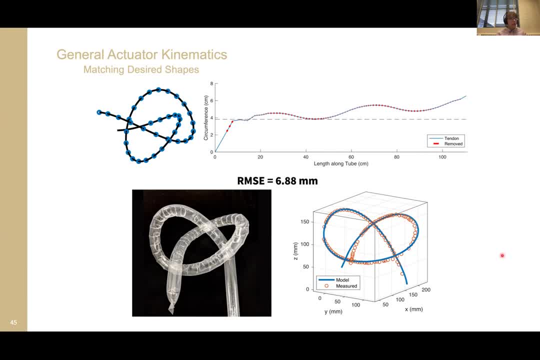 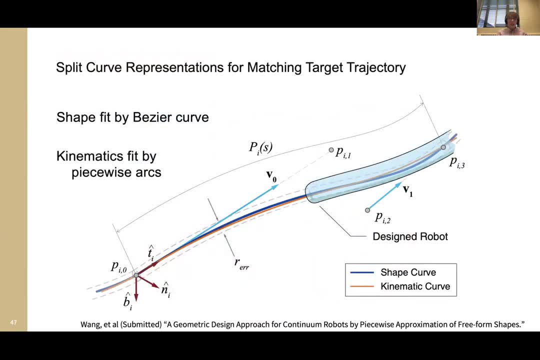 like tying a robot in a knot. But what I want to talk about briefly before I end this talk, here is some recent work that we've just submitted by one of my students where we are looking at better ways to do this. So that previous work that I showed with tying- 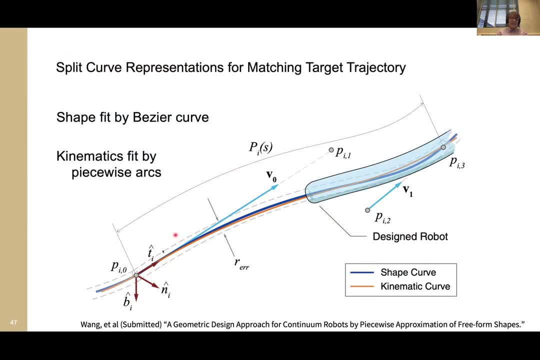 a robot in a knot. it works, but it's a little cumbersome on the actual optimization side. So here we're talking about now more intelligent ways to match a shape that is desired, like something like tying a robot in a knot- Target trajectories, And the main thing that we're doing is we're going to have a shape fit. 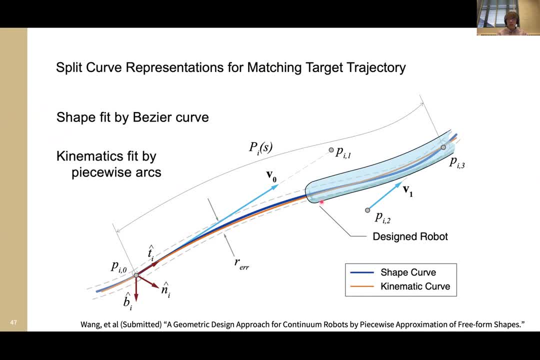 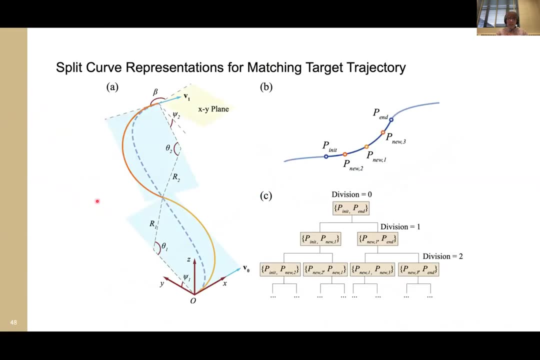 by a Bezier curve. That's going to tell us the shape we're trying to match through some desired points and desired tangents, And then we're going to fit to that Bezier curve with piecewise arcs. The just going through the results here. briefly, we are essentially 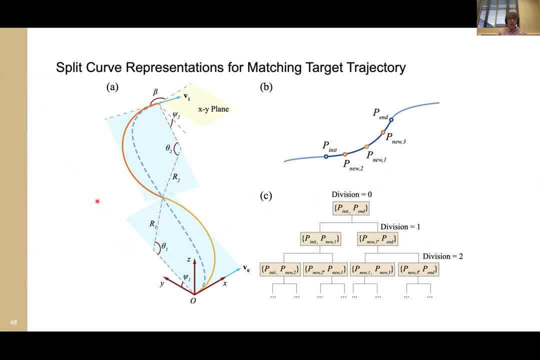 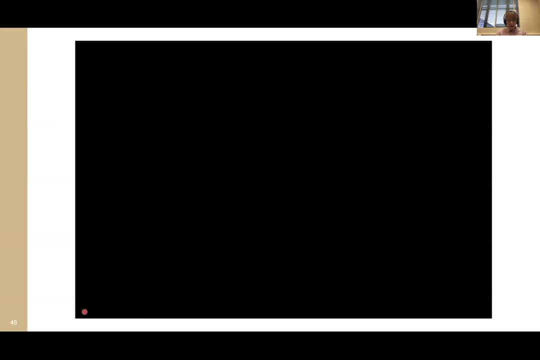 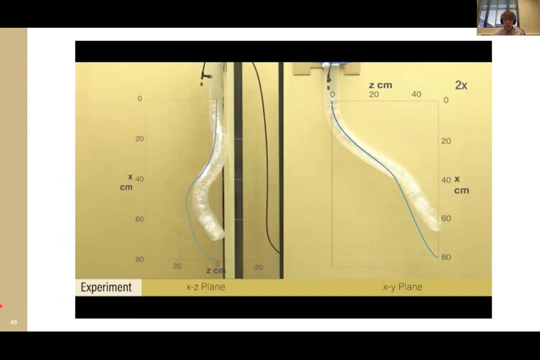 taking that Bezier curve and breaking it down into segments as we need, to get the accuracy we need And we can then match in space. you know these arbitrary curves through points fairly well. again for soft robotic shapes, with both these preformed shapes. 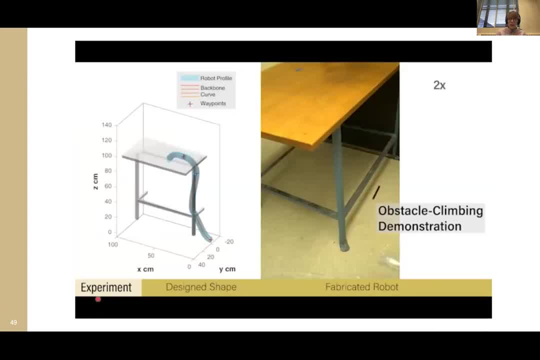 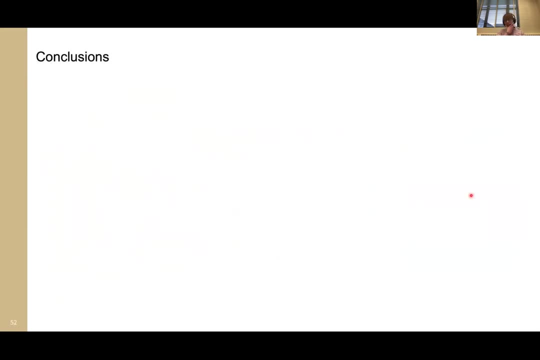 and with actuated shapes We get a little bit of error due to gravity, but overall we are pretty well able to match our target shape in space. So with that I think I'm just about out of time, So I will finish with just some kind of concluding. 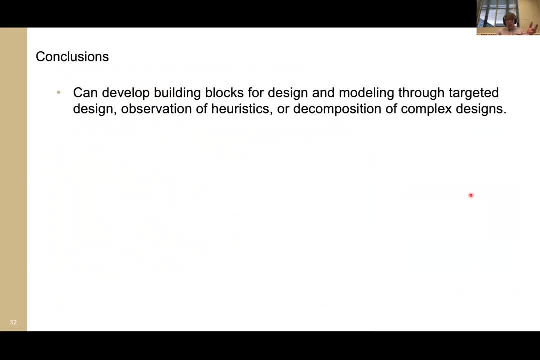 remarks here. So again, my philosophy here is: we can build building blocks for design and modeling for soft robotics through targeted design, observation of heuristics and decomposition of complex behaviors, And these creative models are able to predict our behavior well enough to design. 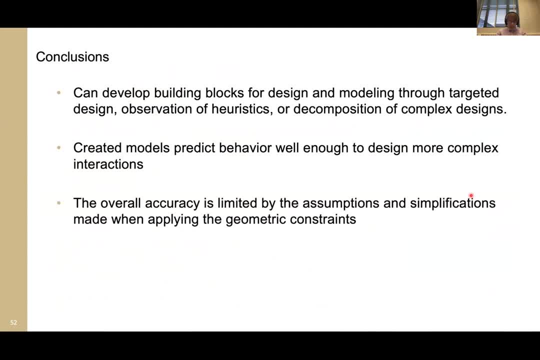 more complex interactions. So I'm going to stop there And I'm going to go ahead and wrap up the presentation Now. the overall accuracy is going to be limited by our assumptions and simplifications made. This is very true in soft robotics. We have to make some simplifying assumptions, Otherwise 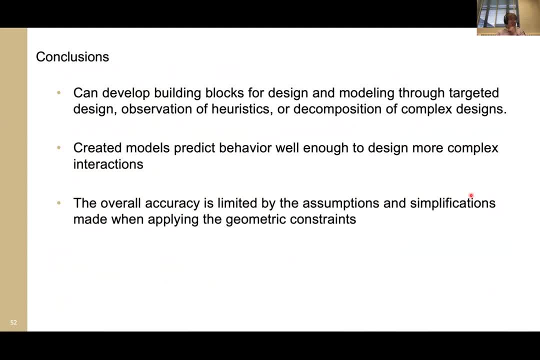 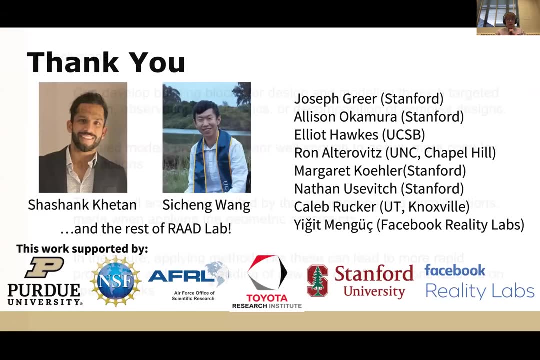 we're going to get locked up in kind of calculations all day And in the future, hopefully, I hope we can apply these methods to get some more rapid prototyping and understanding of new soft robotic functions focused on specific tasks. So with that I will. 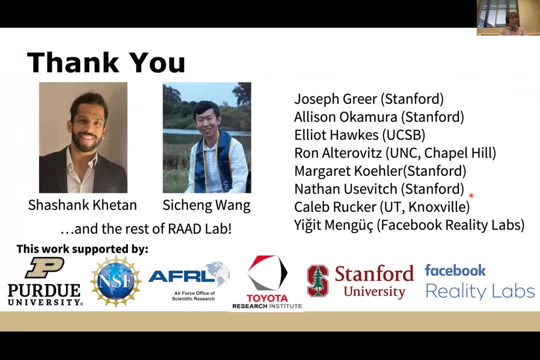 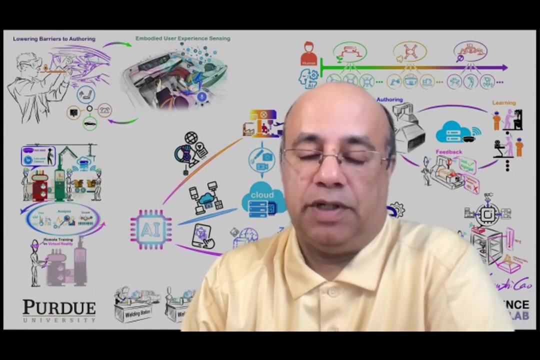 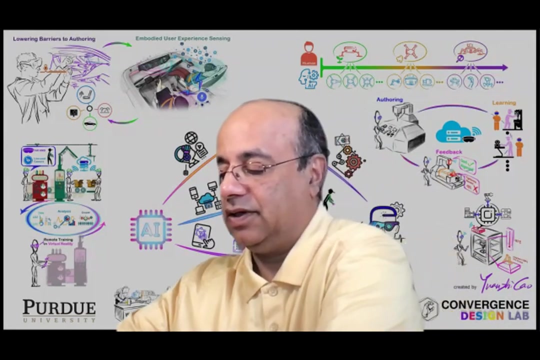 thank the speakers. Thank you all so much for joining us today And we'll see you in the next session. Thank you so much. Very inspiring talks by both of you. If the audience want to type in questions, please start typing them. I will start organizing them and asking our speakers to answer, But also 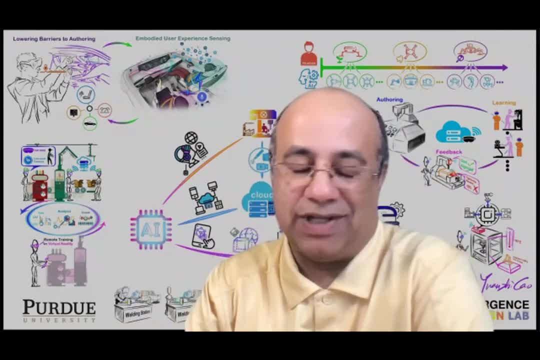 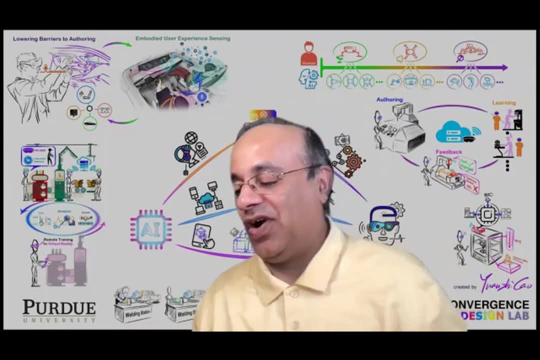 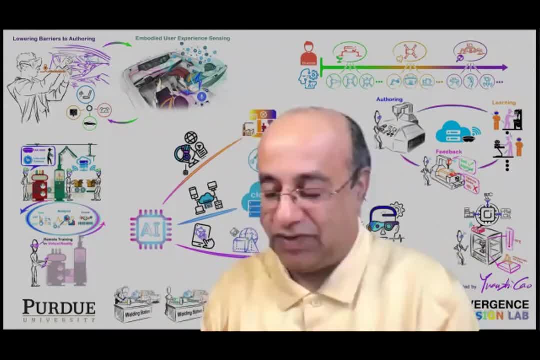 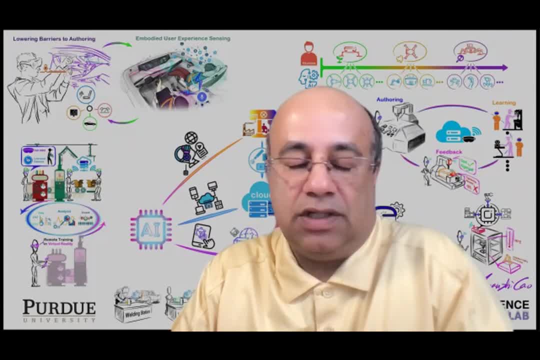 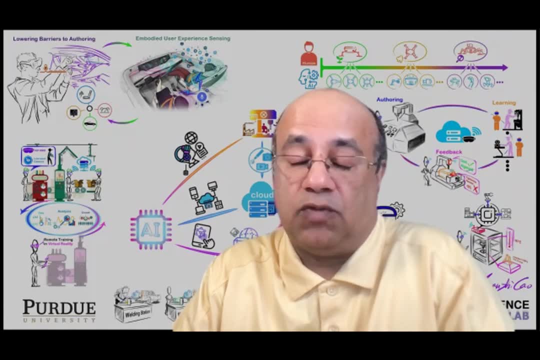 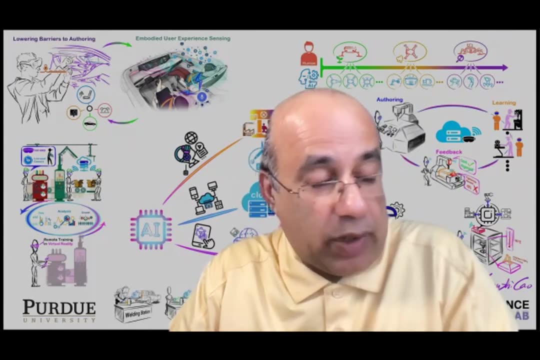 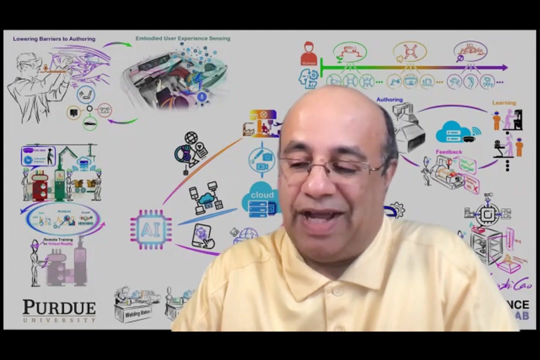 So let me start off with my general question, One question I have. you know both your philosophies of thinking about robots are somewhat different, and there's some commonalities among them. What if you can try to make a more jointed robot- cheetah and exoskeleton- that Patrick is working on with some of the ideas that? 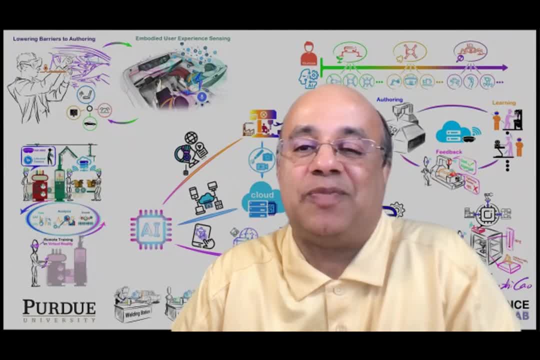 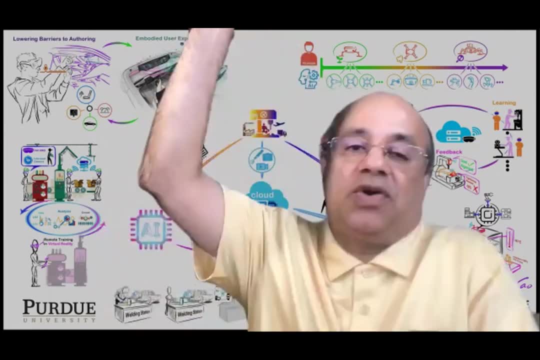 Laura presented the more soft ones. you know can you make a soft robot become hard and do hard tasks, And one of my class projects this time is actually climbing the coconut trees. Apparently, the coconut trees in India are very tall, that variety and all the people that cut coconuts. 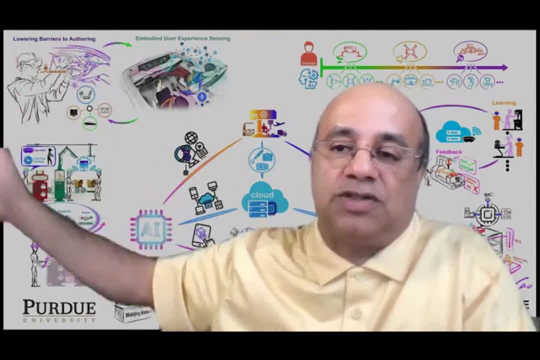 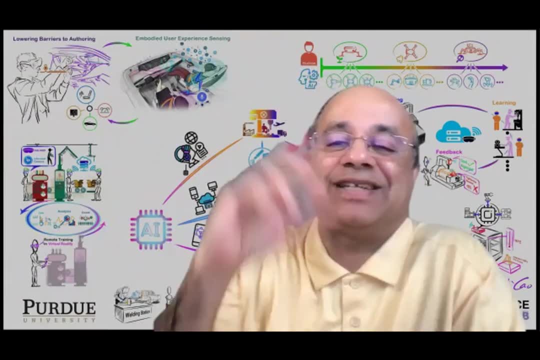 very risky to climb. they all have gone to the Arab countries to work, So they're training monkeys to climb up, and some of your solutions, like this wine climbing robot, could go there and become hard somehow and start cutting the coconuts. 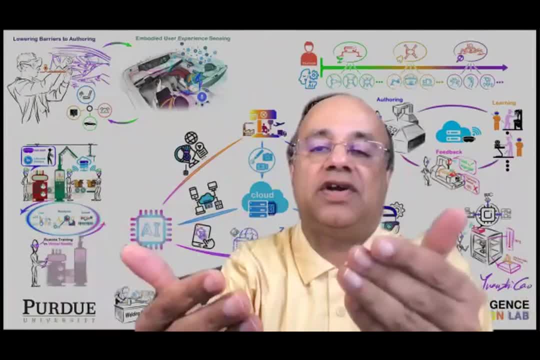 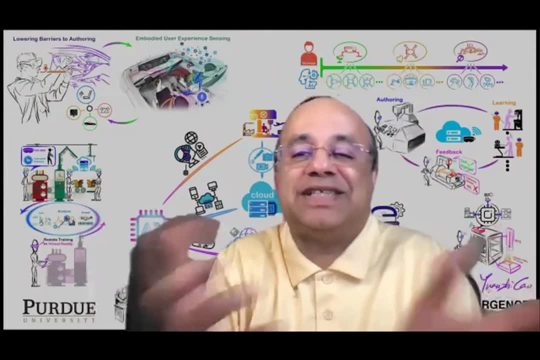 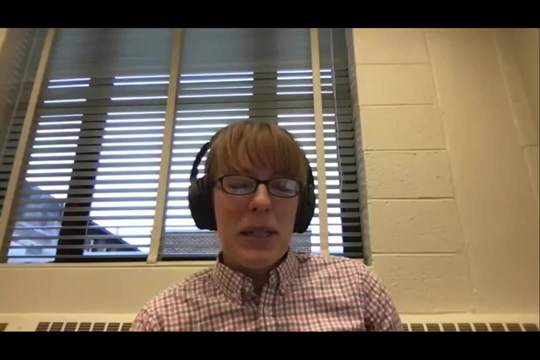 So maybe both of you can come to sides of your own research on perhaps how we can fill this in between ground that we all want to produce robots that can do both your sides, and being one robot, Yeah, I think, maybe, maybe I'll start on that. 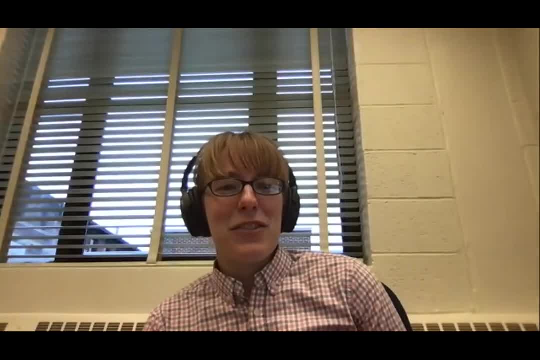 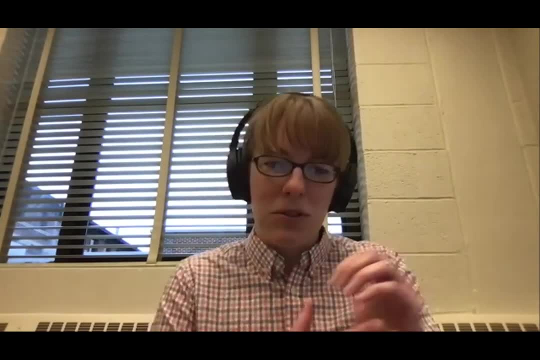 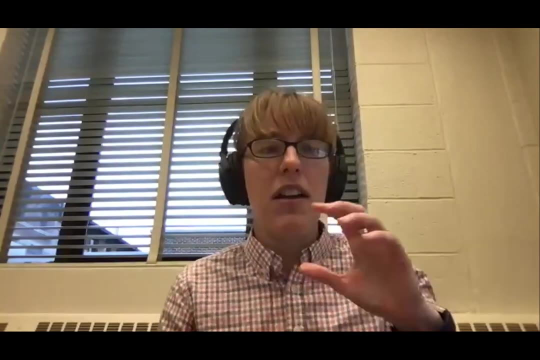 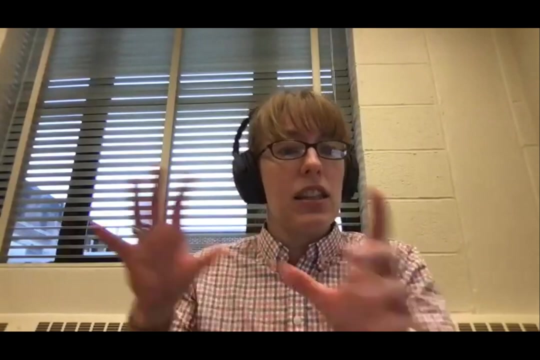 That's a great question And I think, at least from my perspective, this is a big thing for soft robotics as a field to sort of figure out. There are some big steps that need to be taken in terms of building up the control, the modeling of the sensing that is expected at the more traditional 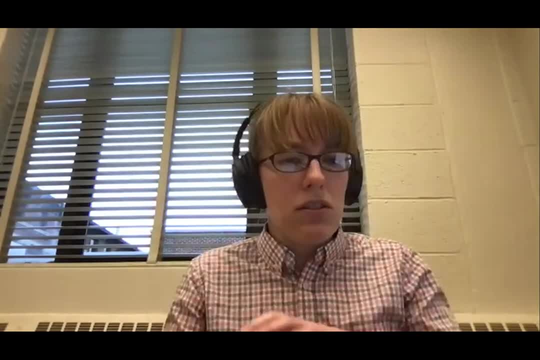 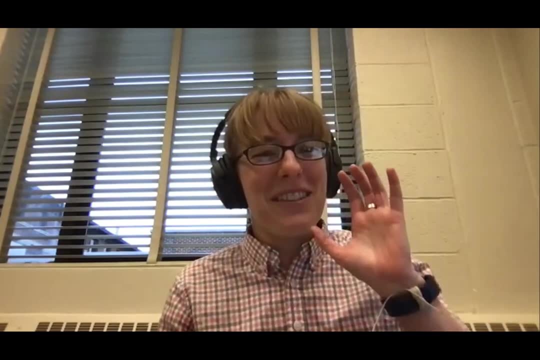 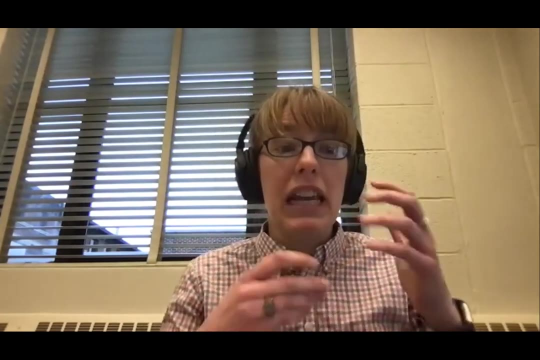 the rigid robotic side of things better merge the fields. Now, interestingly, I'm not sure I'm settled on whether you know the language that traditional robotics talks about. robots will be the same language we talk about soft robotics, But I think we're going to have to have something along those lines. 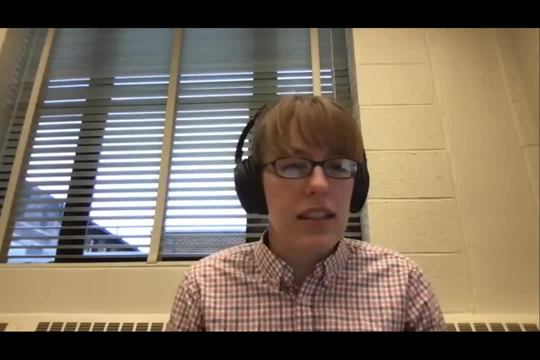 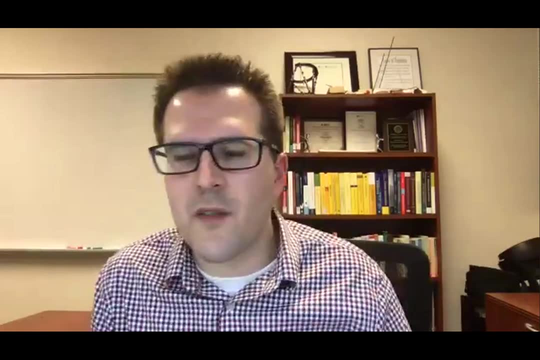 in order to understand sort of how these systems work together. Yeah, Yeah, I mean, I think it's right now. there is a divide, right? The people that work on rigid robots are, you know, they're worried about precision down to, you know, maybe tens. 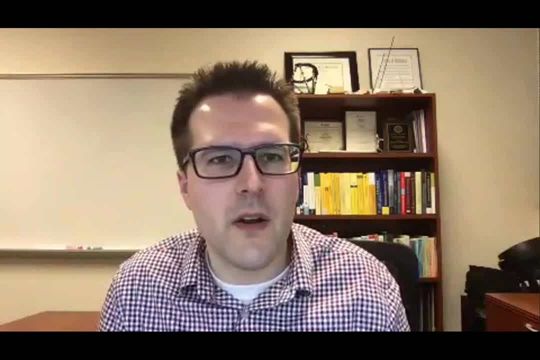 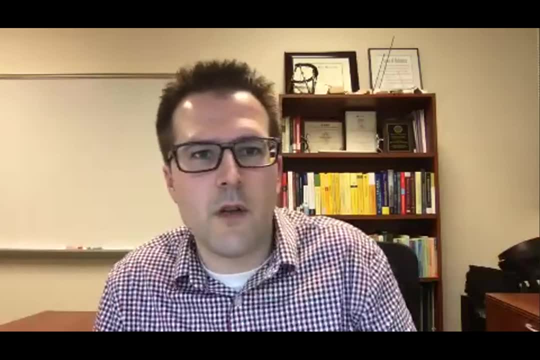 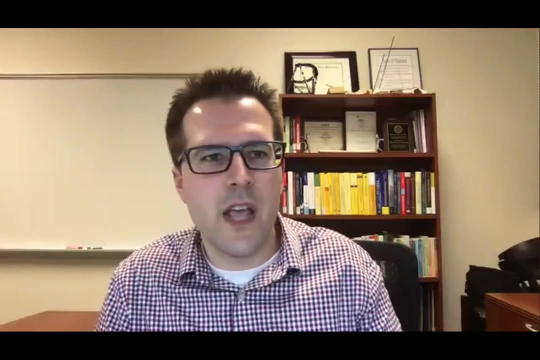 of microns if you're working with an industrial manipulator And you just can't get that with soft robot models or with soft robots- And each had their, you know, unique benefits And we've seen, you know, attaching soft robot grippers to the end of rigid manipulators And those have 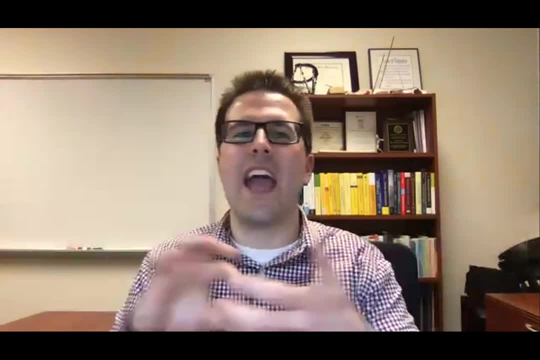 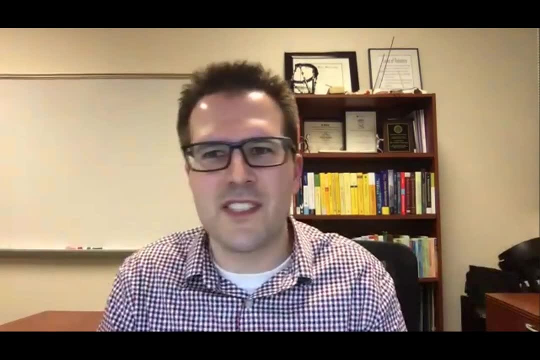 had a great deal of impact, I think, without these two worlds really having to mesh and combine with one another. but they're, you know, our human bodies, right, are made of bones and all these soft, squishy materials, And we'd like 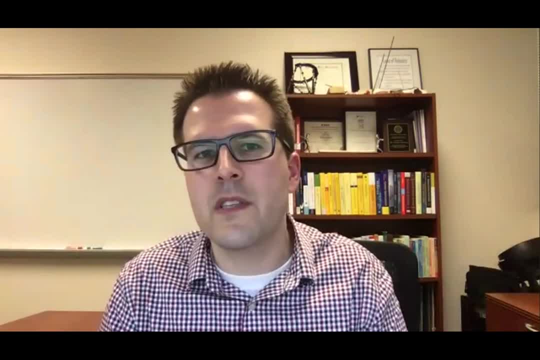 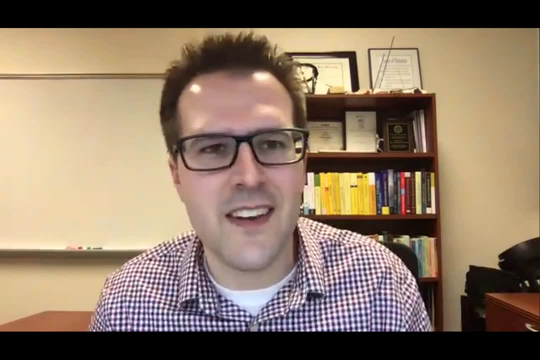 to be able to design robots that incorporate, you know, both types of components. I think it just takes some intrepid collaborations to really kind of bridge the different types of thinking that traditionally inhabit these different sub-disciplines. And I think the one thing I will 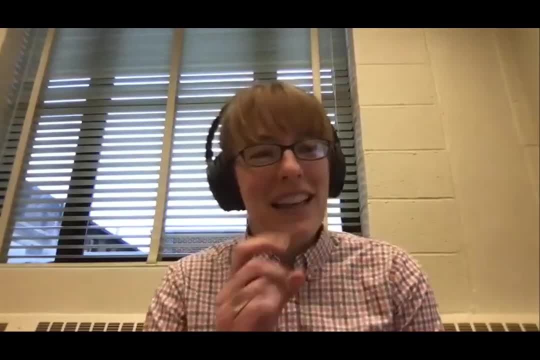 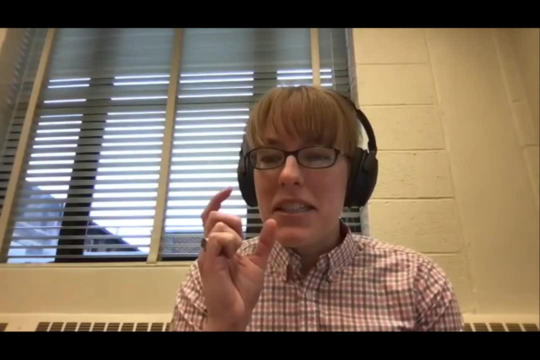 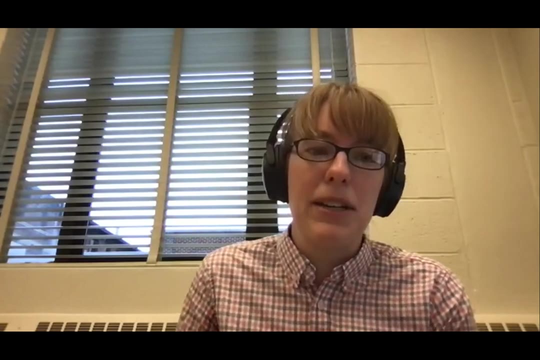 say, is Karthik to your point of: can we make a soft robot that becomes like incredibly rigid? I think you know that is a very much in the materials problem. That's where I think we need to get more people on board in terms of collaboration. This is a thing that I'm incredibly interested in. 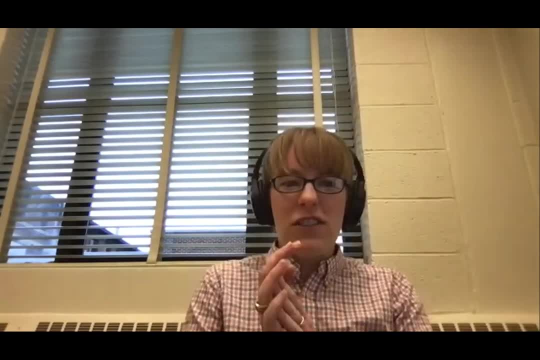 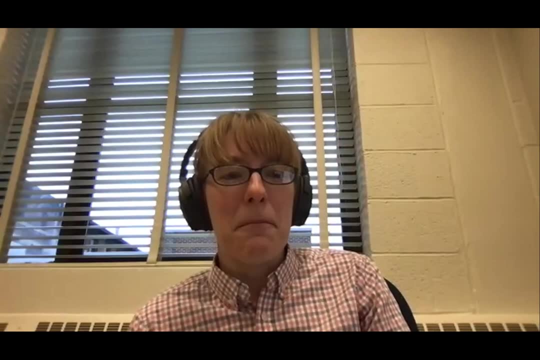 because I think that that is one of the you know, if you can have a soft robot that shifts to this very rigid system, then we're talking about you know, something that inherently bridges this gap, But the orders of magnitude. we're talking about the ability to stiffen. 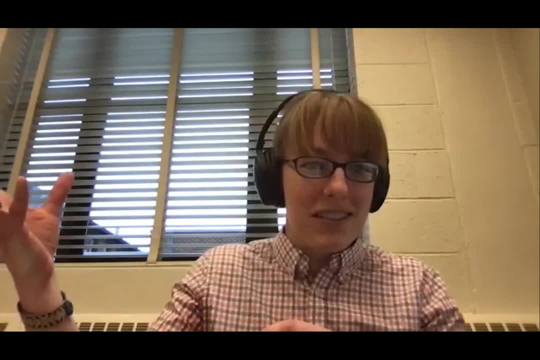 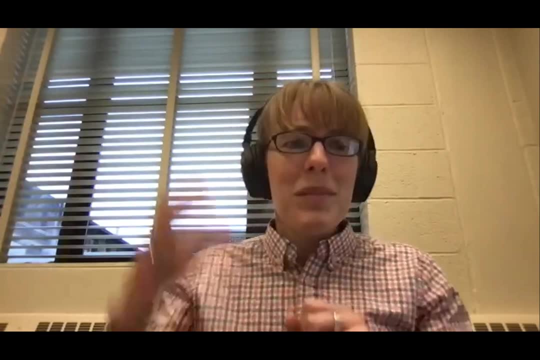 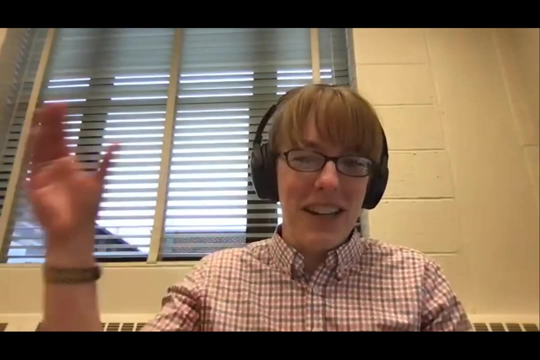 a soft robot is nowhere near the rigid robots level. You know we can get one order of magnitude maybe stiffer than the materials we start with. And it's also interesting: on the rigid robotics side of things I started off doing a series elastic actuation, So I know kind of coming. 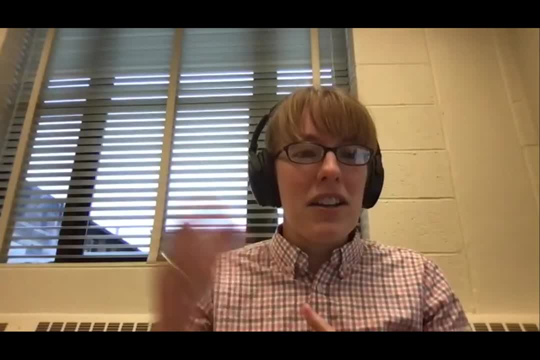 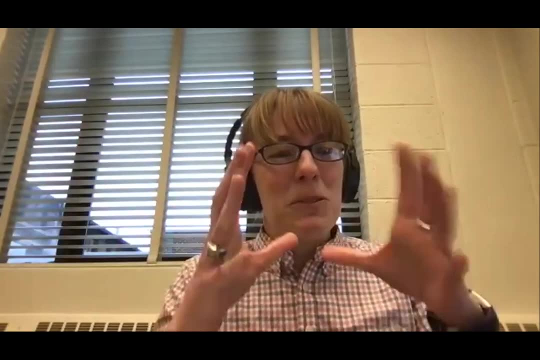 from rigid robots going to compliance, where even there you're not going very soft ever for controls reasons. So we're kind of going in both of these directions, but we're not really meeting in the middle of the same area. So I think that's a really good point. 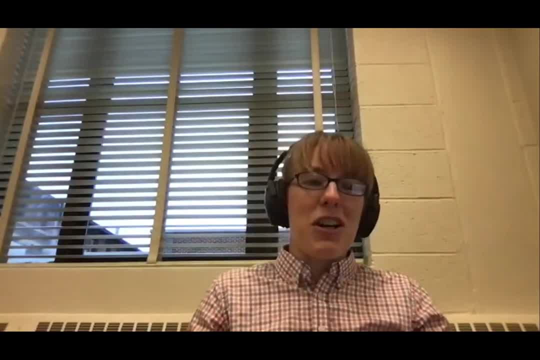 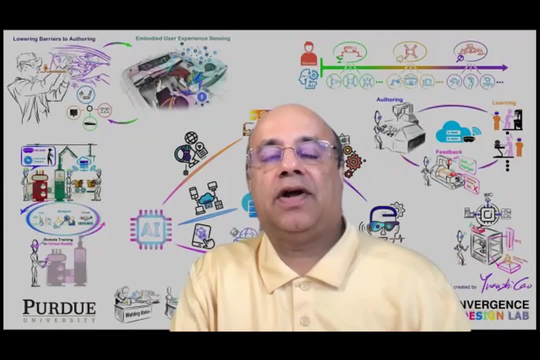 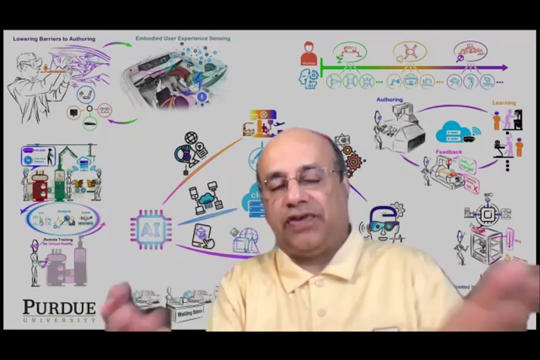 In terms of the stiffness levels we're talking about. Yeah, Great comments from both of you, Sort of along your directions. I recently did some homework on what's happening in the commercialization side of both your sides, or everything in between, And I was surprised to see that Soft Robotics. 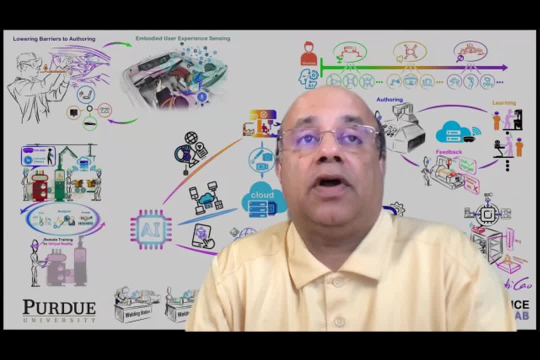 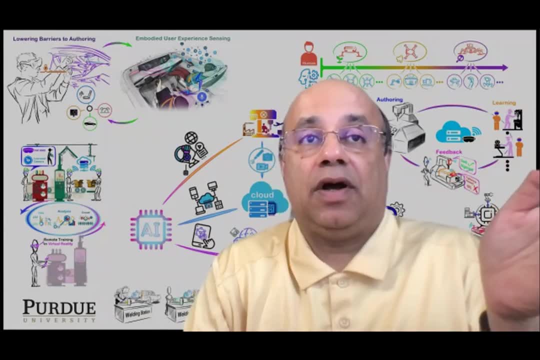 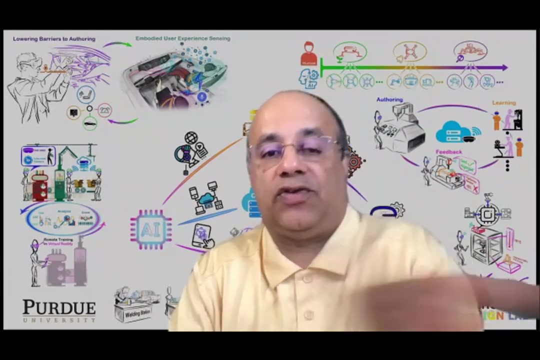 one of the companies actually cited increased demand for soft grippers for their hard robots And raised an additional 10 million. I think they raised close to 50 million or so. That's kind of surprising to me that they could make a case for such a race, And also on Patrick's side. 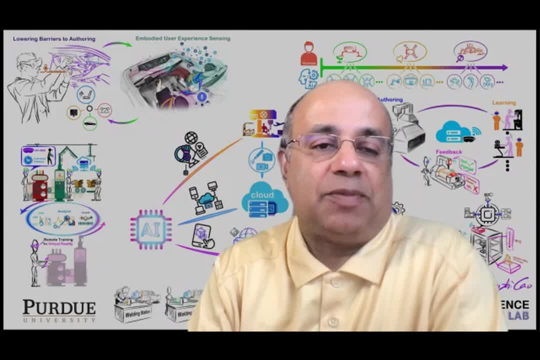 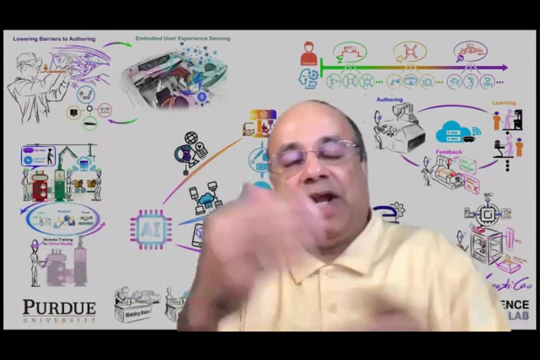 I was wondering when I can go to the market and buy a galloping cheetah for the kids- and I teach toy design, So that's kind of cool. So I'm kind of curious, from both your perspectives, how you see the future evolving and 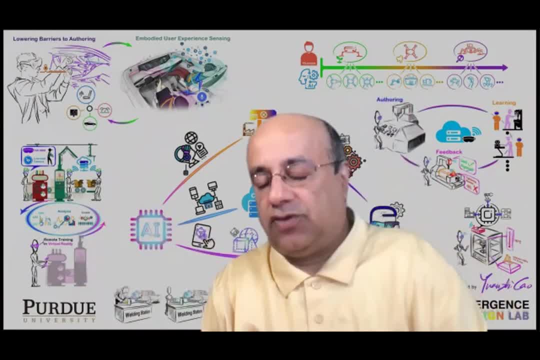 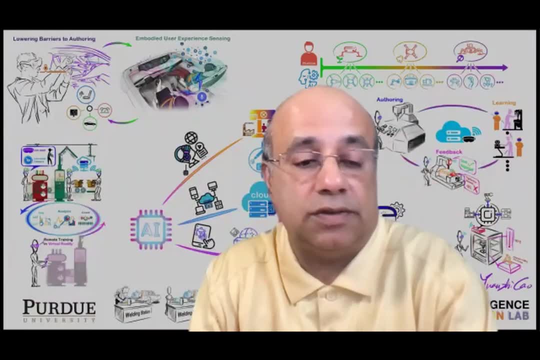 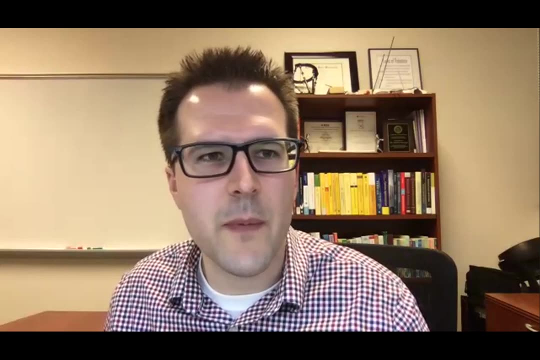 both your sides becoming more ubiquitous. Maybe it's from the exoskeleton side or from soft grippers themselves becoming more like robotic forms like what you're talking about. Yeah, I guess, Karthik your question of when can you purchase a galloping Quadribet. 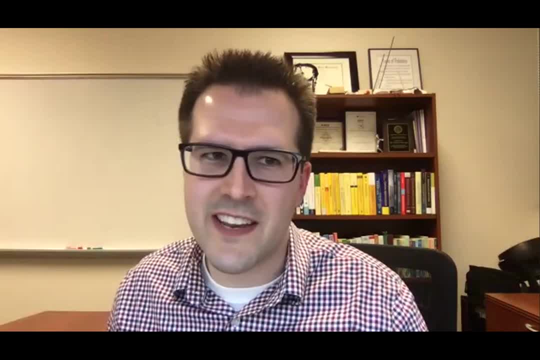 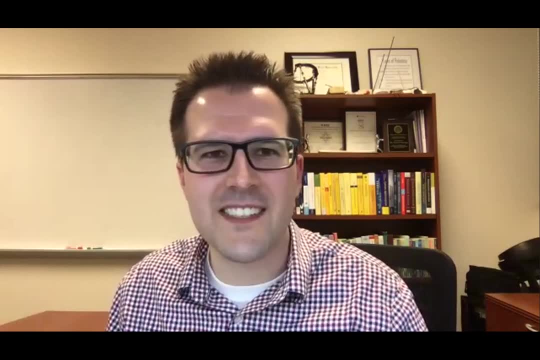 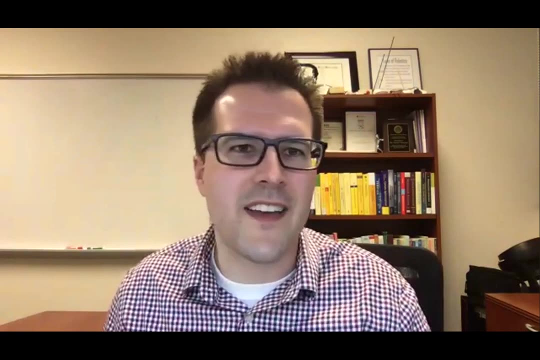 it depends on the limit on your Amex card, because if you can go up to 70K you can go onto the Boston Dynamics website and get yourself a spot. But I guess, in all seriousness, You know we've seen a lot of market penetration on the quadruped side and you know surveillance type applications. 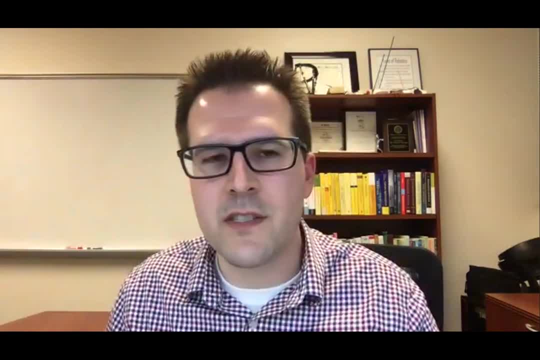 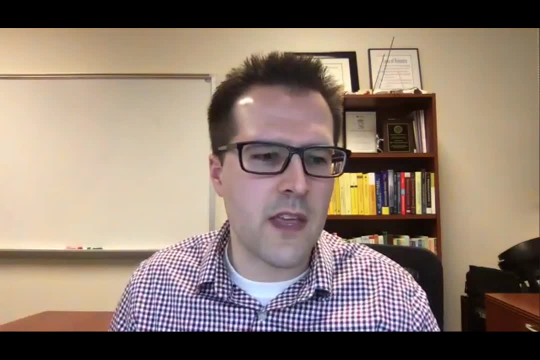 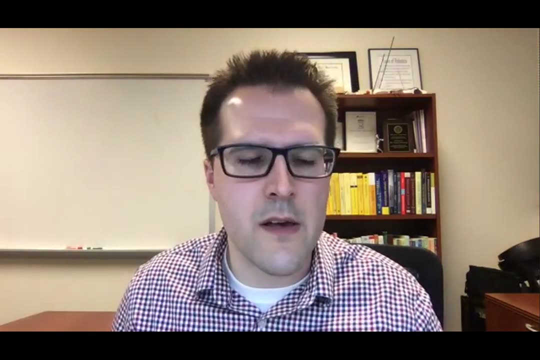 Again he's like: look, but don't touch type applications, surveillance and monitoring at work sites and at chemical plants. And you know, I think as economies of scale kick in and more people can get their hands on these hardware platforms, then we'll see more applications opening up. 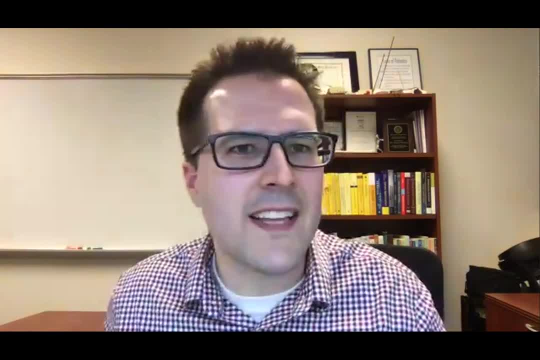 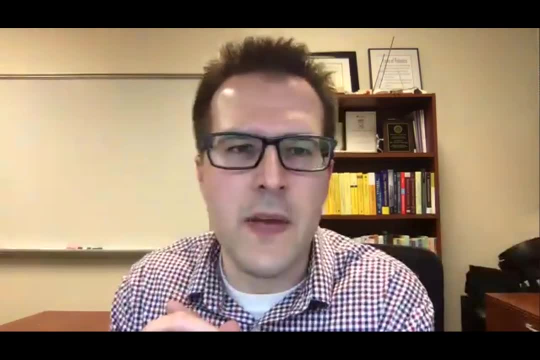 But yeah, you know, in terms of soft gripper hands, I think you know the manipulation landscape is just really, really difficult in terms of the complexity of the environment. In locomotion we have to worry about different types of terrains, but for manipulation I have to worry about different types of mugs and plates. 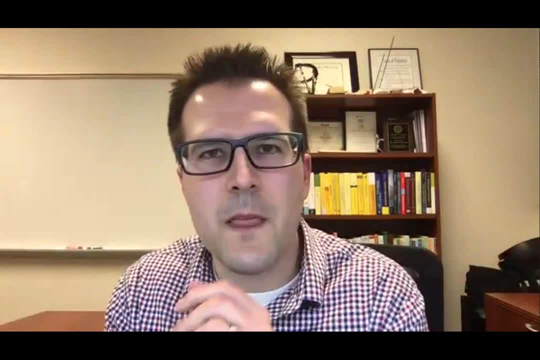 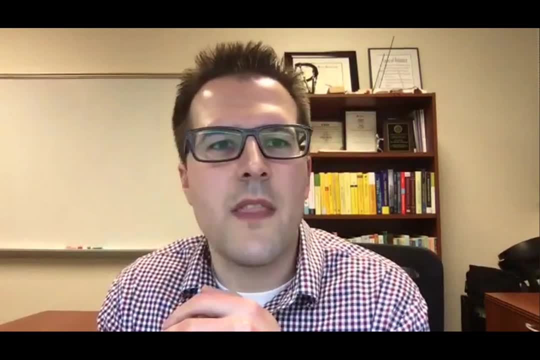 And all sorts of crazy different shapes. And so I think you know, in terms of quadruped applications, you know the maturity of manipulation in the coming, you know five to 10 years is going to open up many, many more applications. 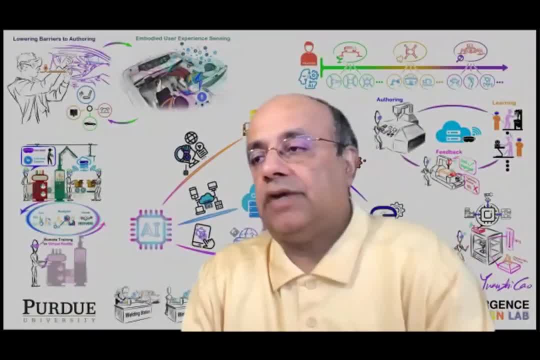 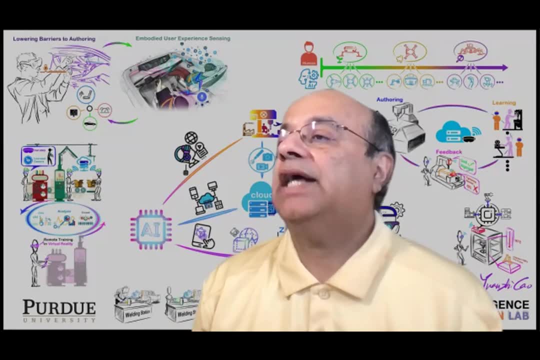 And I'll be excited to see where that goes. Great, great Yeah. So I'm going to post one of the questions asked by here on the chat. So he's asking both of you: do you think you can use your modeling techniques to model the soft robots? 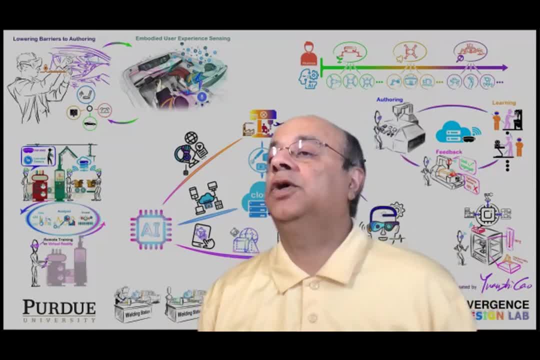 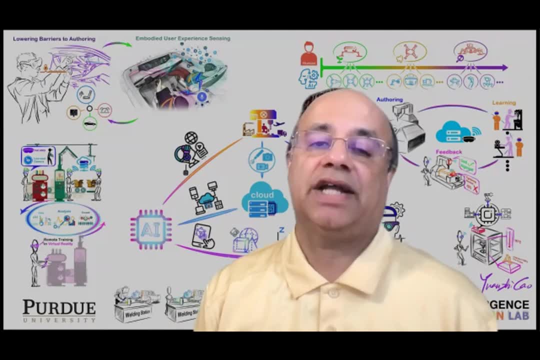 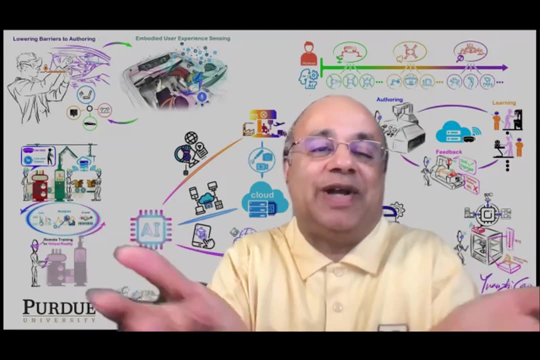 That make up the human body, muscles and other soft tissues, to predict rigid human robot skeleton system to inform the exoskeleton prosthetic actuation and reactions- sort of- perhaps a coincidentally- use case for the first question we asked. Maybe this should be our joint paper next time. 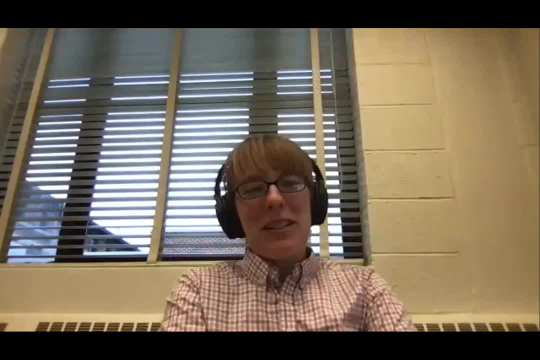 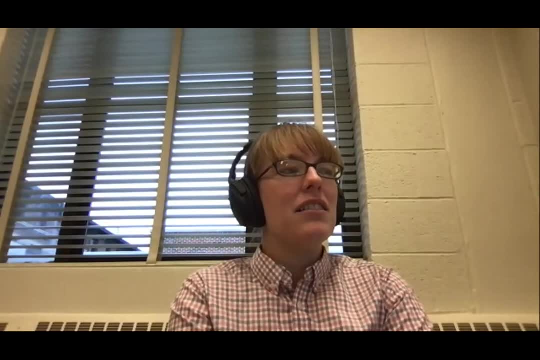 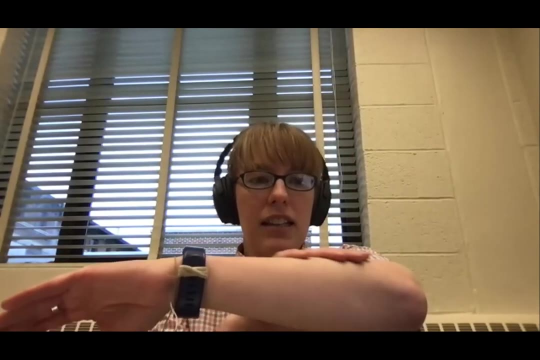 This is a very interesting question. I'm sure Patrick has more more exact things to say on it, So I will just say by one comment from my side, which is Soft tissue modeling, especially when we're talking about, like how you can attach to the body and like localize the body, is incredibly interesting and looking at. 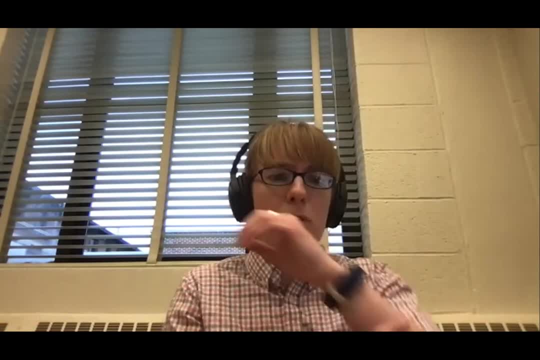 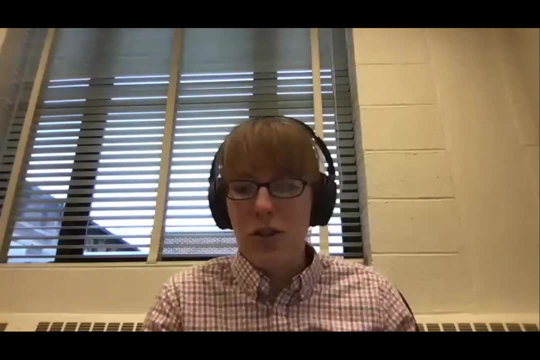 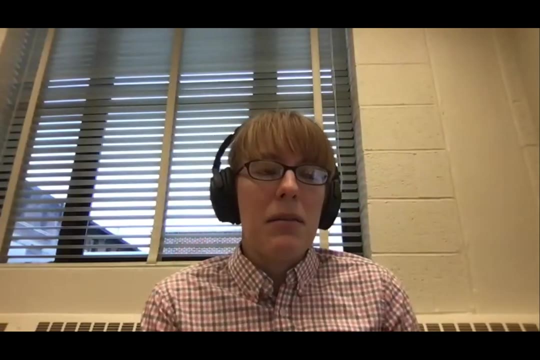 There's been some recent work just looking at how do you understand, you know, the stiffness of someone's skin and their, their kind of soft tissues for things like haptics, exoskeleton. So I think that that's a growing field and I'm 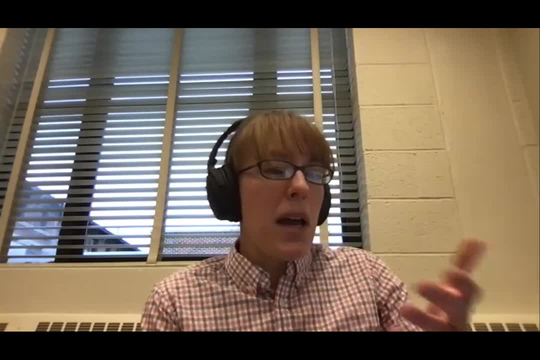 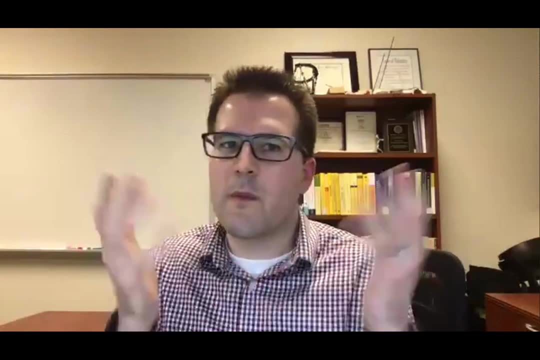 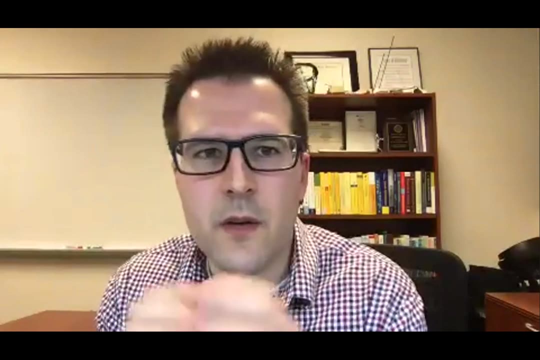 And to maybe we'll see some results for that, for better melding of robots and humans, in the next few years. Yeah, so I guess you know we've been looking at estimating the goals and desires of humans from the standpoint of walking speed and you know, getting models of this kind of one number, 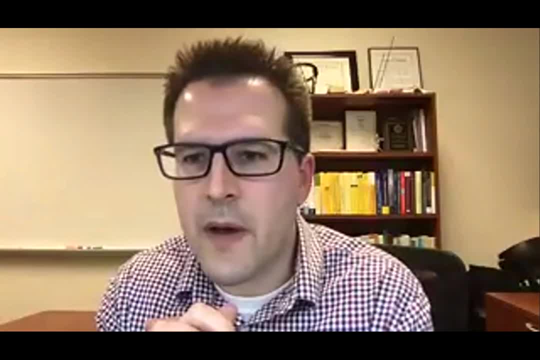 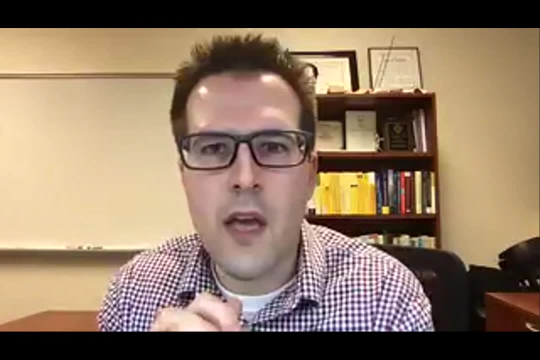 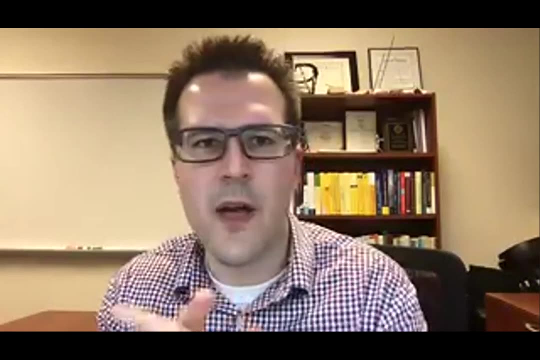 is challenging. Now, if you start thinking about modeling the entire human body, we're talking about, you know, hundreds of degrees of freedom, more hundreds of actuators, and you know that's just an incredibly difficult modeling task in terms of, you know, every muscle itself has. 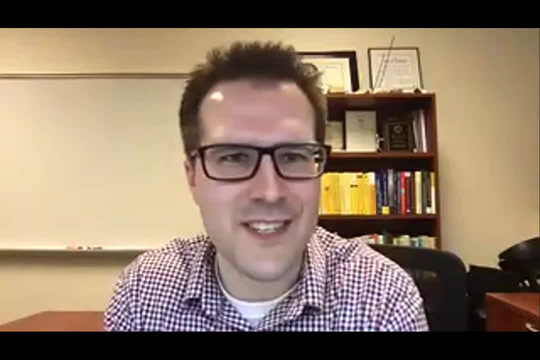 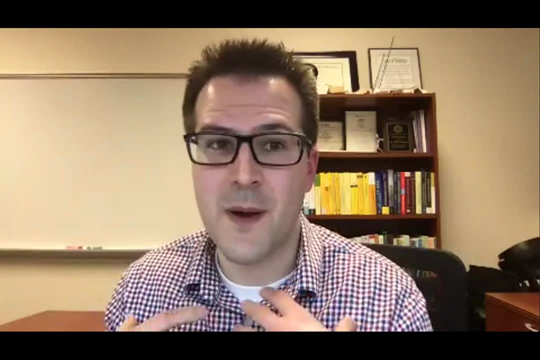 different parameters that govern its. you know, force-length relationship, force-velocity relationship, and so I think it's just I personally feel like it's probably too much to ask to try to get right Like you can model it and get close. but if you 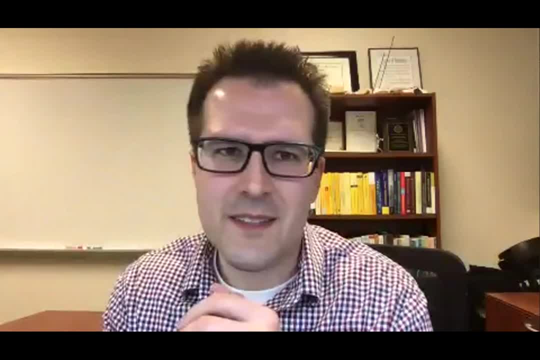 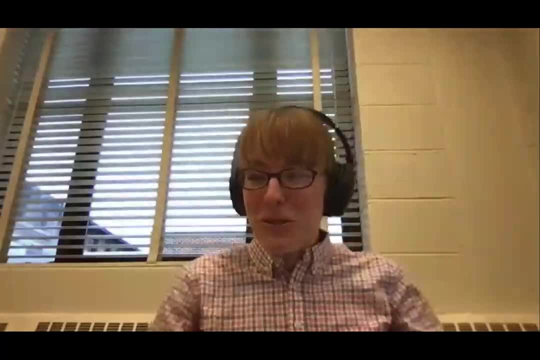 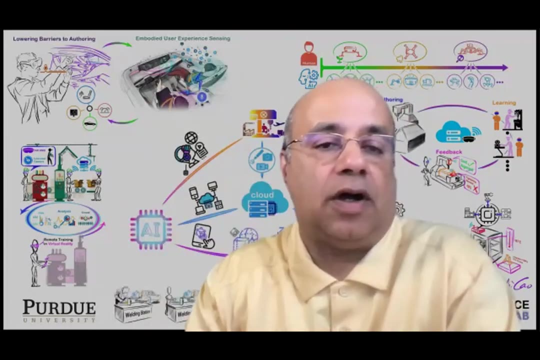 you know, in terms of getting the minutiae right, it's just: yeah, that's more complexity than I want to bite off. Yep, I would agree with that. I guess what you're saying is there's going to be some diminishing returns after some level of modeling on that part, but you certainly appreciate that. 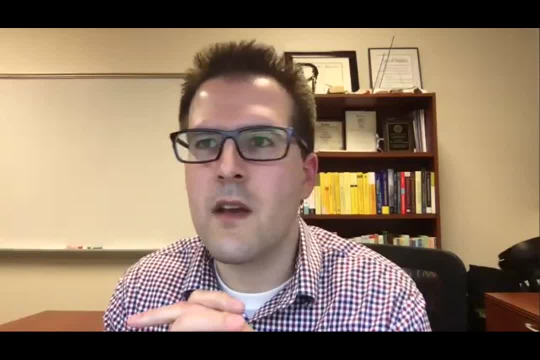 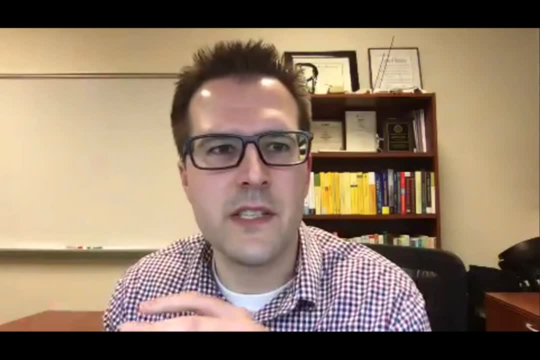 direction of thinking, I guess, Yeah, and I mean you don't, you know, I think in terms of some of the work out of the work out of Scott Delp's group, in terms of optimizing assistance and that type of thing. 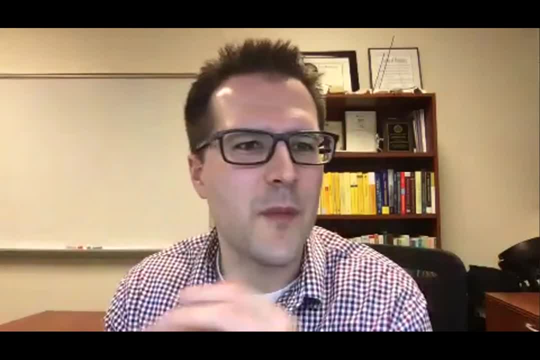 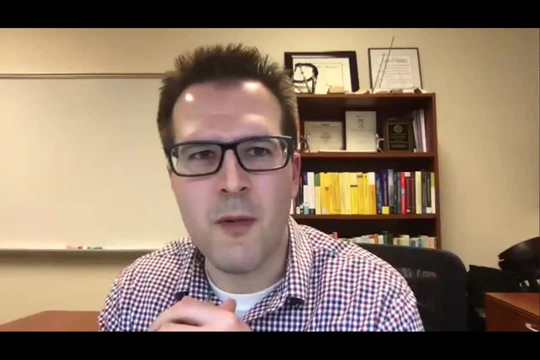 you don't have to get things perfectly right to make more informed choices about how to control your assistive devices. and I think, yeah, like in any engineering problem, all of our problems are complex and it's a battle of managing complexity and making the right choices. 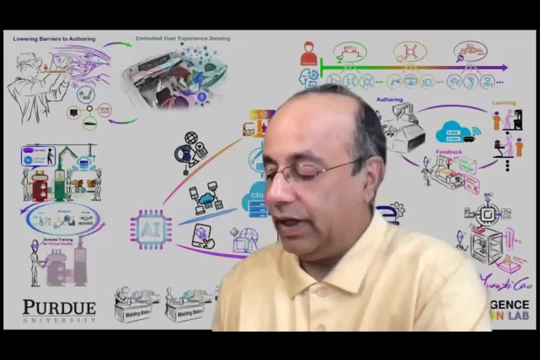 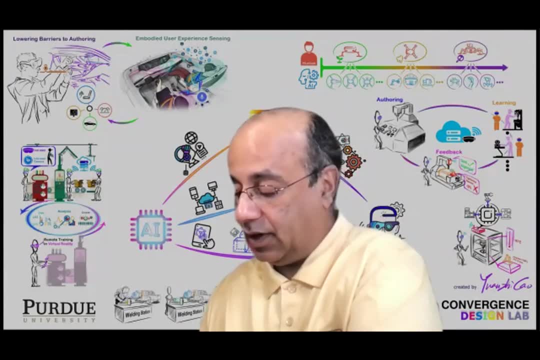 to give us the most bang for the buck, Right? so any other questions from the audience? There's only a few of us here, so feel free to unmute and ask. If not, I'll get to them all. I do have a lot more questions. when I was talking to Patrick and Laura, we very soon finished our 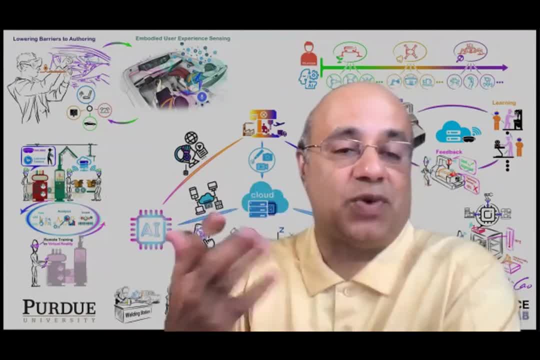 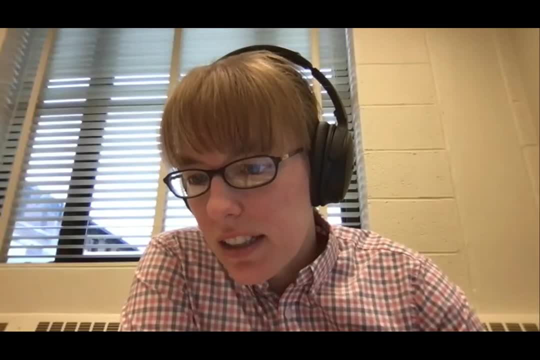 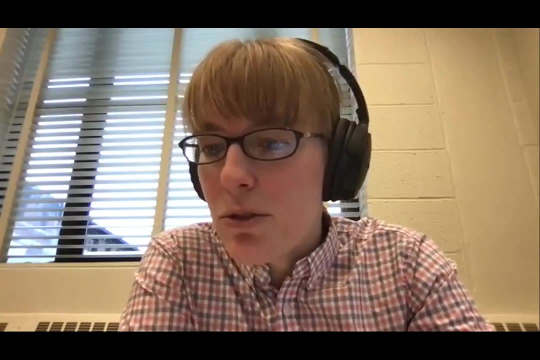 half an hour and still had a lot more different questions to think about. So anybody in the audience wants to. I think I do see one question from Margaret in the chat. Go ahead. She said: how far are we from being able to apply the model-based control schemes like Pat talked? 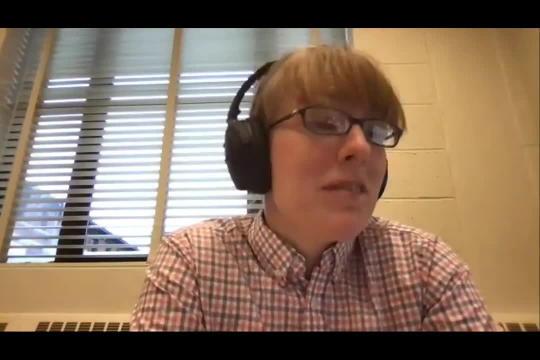 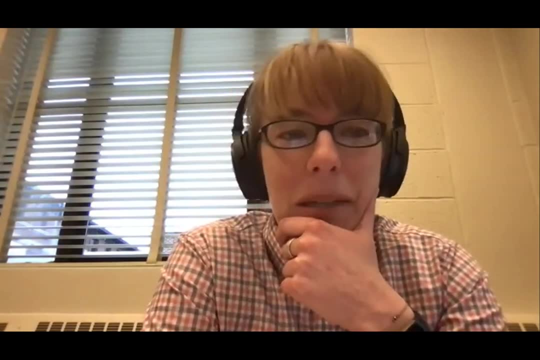 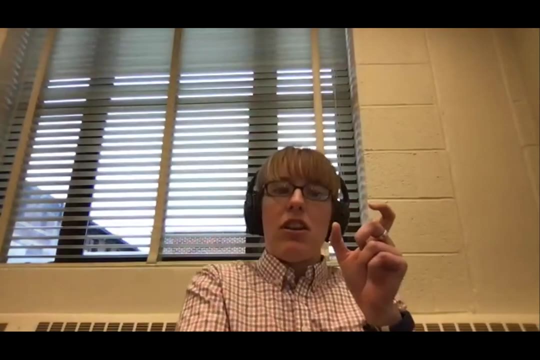 about to the soft robots like I talked about. I think that's an incredibly interesting question and one that I would place- I would kind of place to Patrick as well- of like, what do we need to be able to do in terms of actuation on soft robots to then start applying this model-based control? 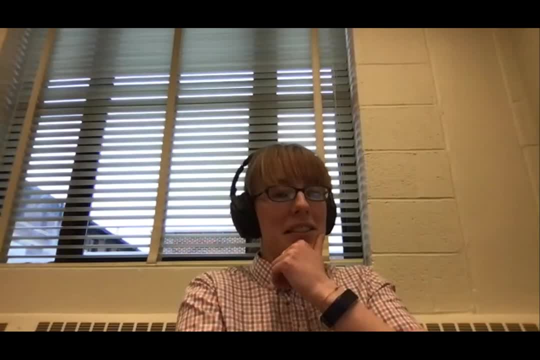 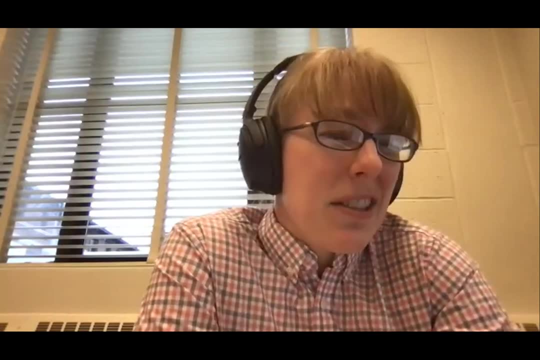 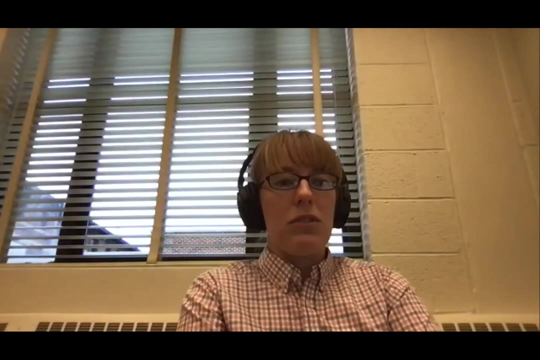 Because I know that some soft robots, some compliant robot systems, especially continuum robots, have done some amount of model predictive control, but it's not. it's not really widespread, and my first thought would be that we just don't have enough control authority over the resulting shape in order to make it make sense. But maybe we're also just not. 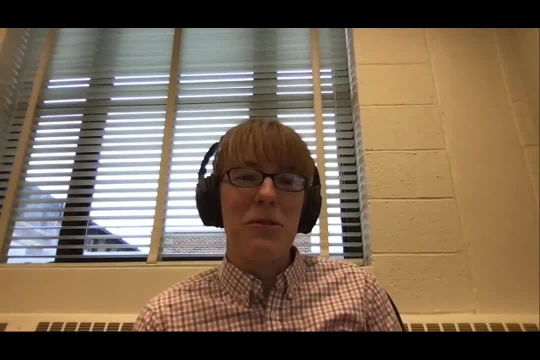 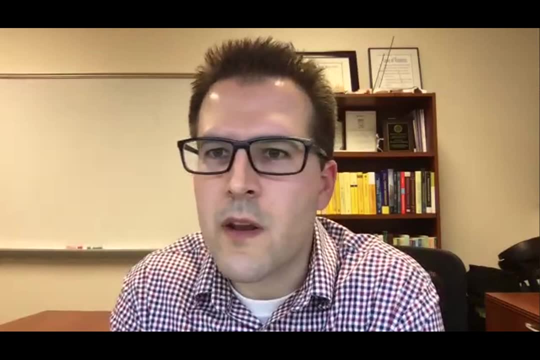 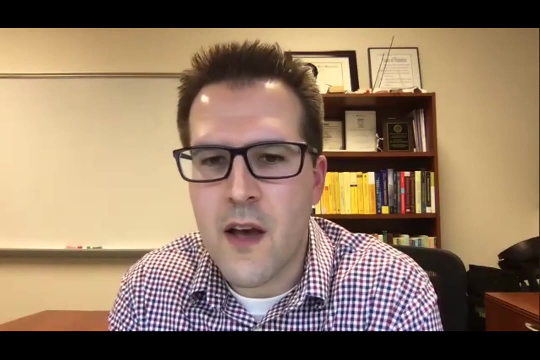 we're missing models that are good enough to do model predictive control. Yeah, I totally agree with your second point that you know these PDE models for how soft robots move around the world. There have been some very impressive numerical methods that folks have. 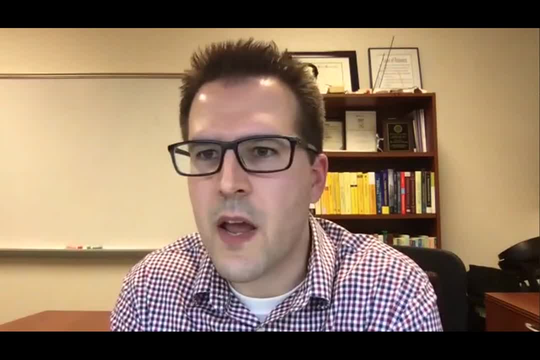 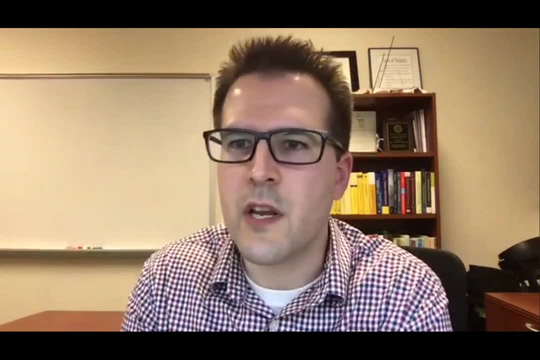 developed over the past- you know, five years or so- for simulating these systems. but I don't think that the field has got to a point where those are kind of like a you know, take it to the bank- technology in the way that we have for dynamic models of our rigid robots in terms of you know. 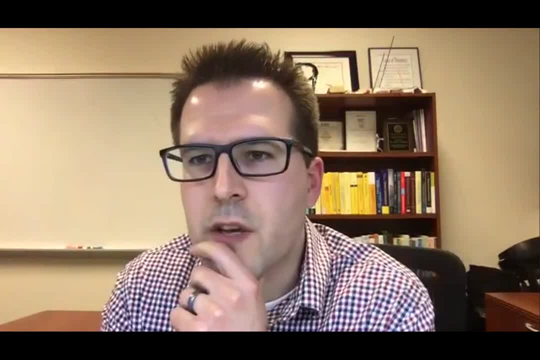 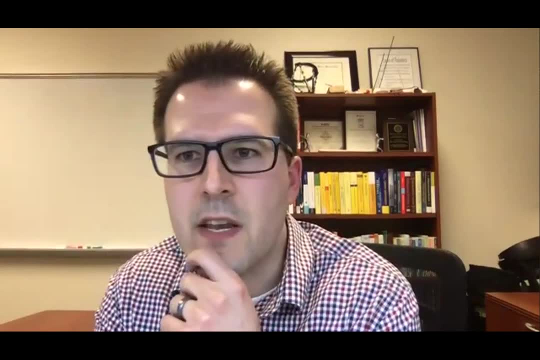 there being a textbook method? Yeah, And so I think that's a, you know, just an aspect of maturity of the field that hopefully will change over the next five to 10 years, and I think then we'll be ready, Yeah, Yeah, And to that point I think. 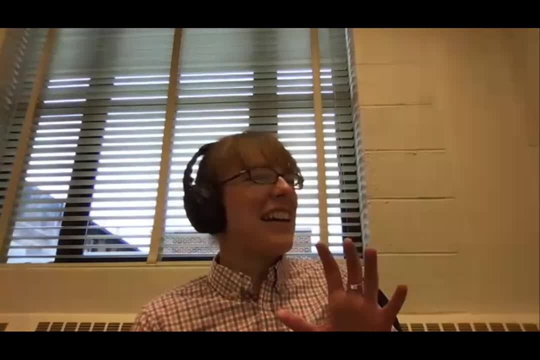 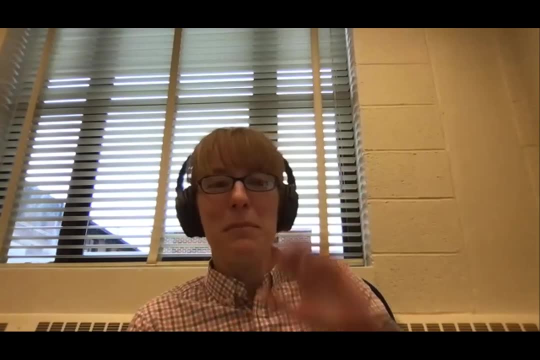 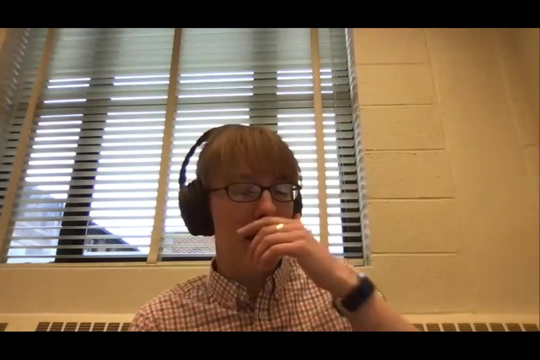 you know, you maybe got a sense from the talk that I gave, but the different ways we- model systems, soft systems- are very kind of scattershot. now Some people are very on the team of you know finite element simulation and things like that, And I think that's where Patrick 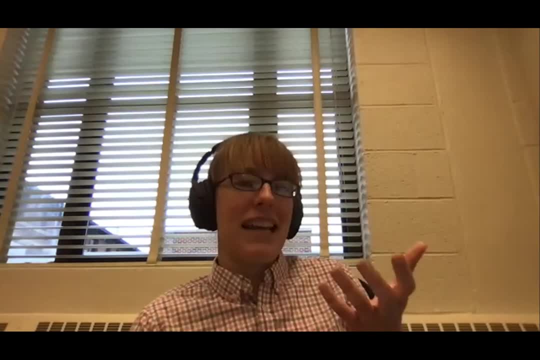 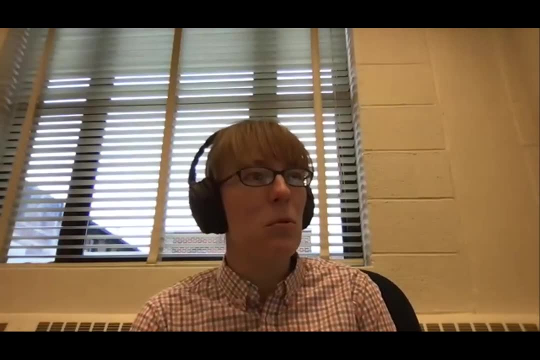 a lot of the results you're talking about have come out of that, But there are a lot of downsides with that as well, in terms of complexity and computation time, which you know don't necessarily make them one size fits all solutions. 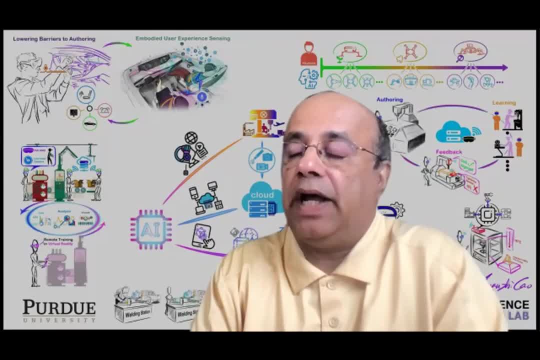 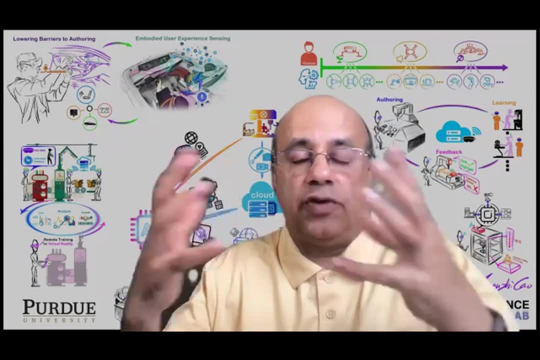 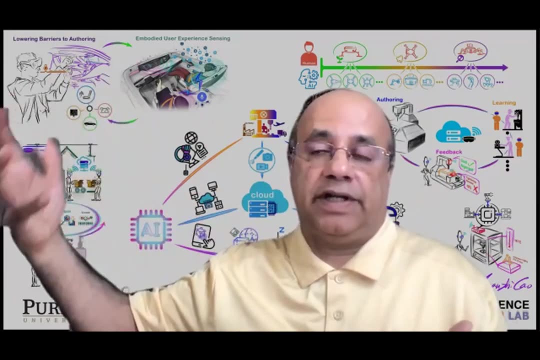 Great. If there are more questions, that's good, But meanwhile I have another question or thoughts for you to comment on. Both of you had some use of this personalization right. Like Laura was sort of almost saying, like you know, one robot for every different task. 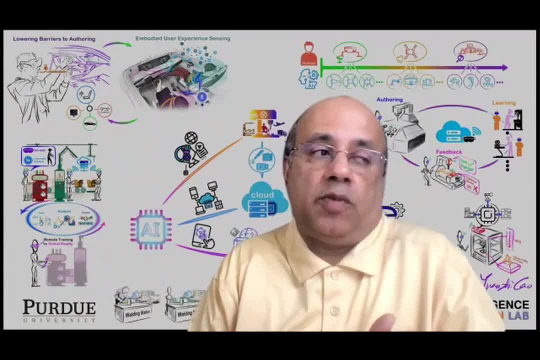 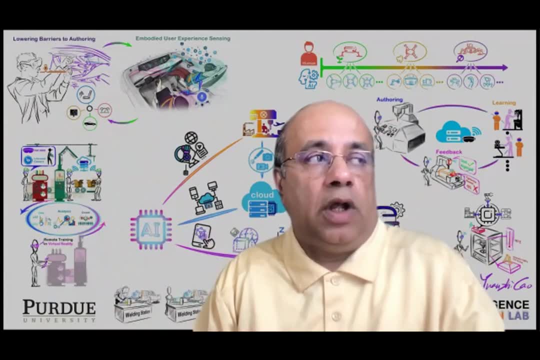 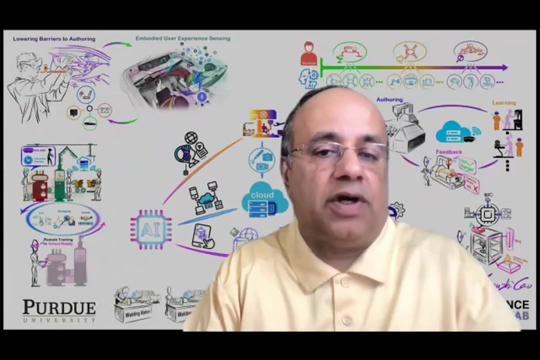 and for a side I would say, you know, I might want to make all kinds of legged robots of different kinds and try them out. So from that point of view, clearly there's need for toolkits, tools, education, for the lack of better words, textbook-based ideas, right. So I would like both. 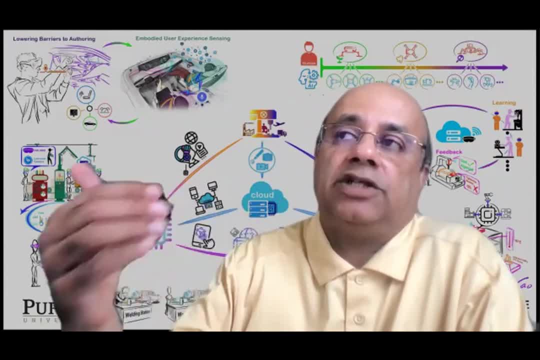 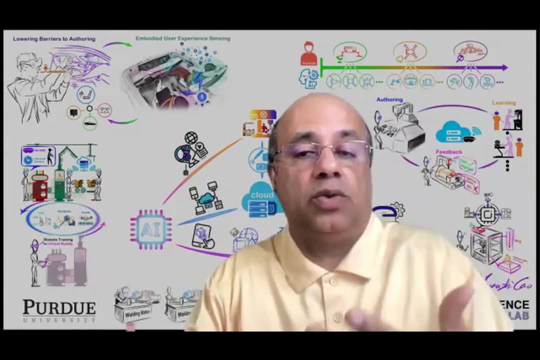 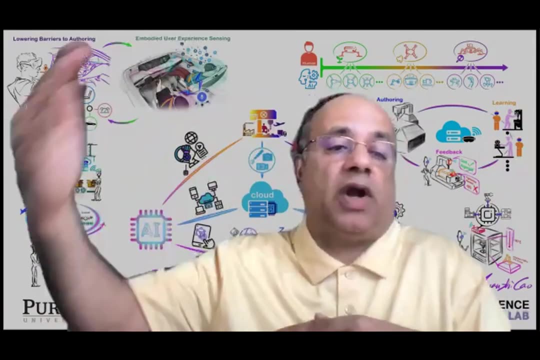 your comments on what do you foresee as the nature of research, and especially open source kind of research that people can reuse in order to experiment and create new types of robots, perhaps in senior design classes and so on, just elevating the level of projects that? 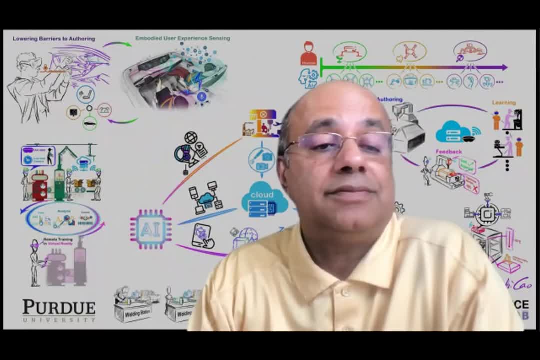 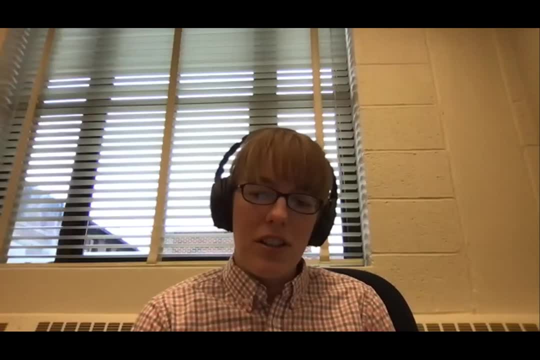 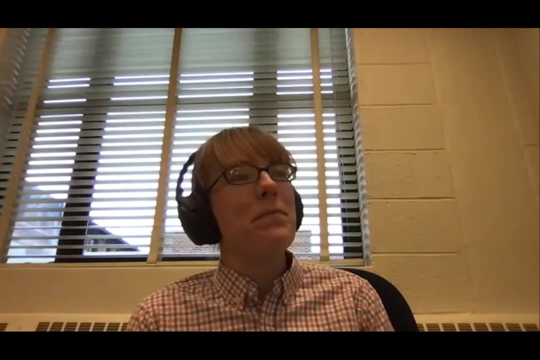 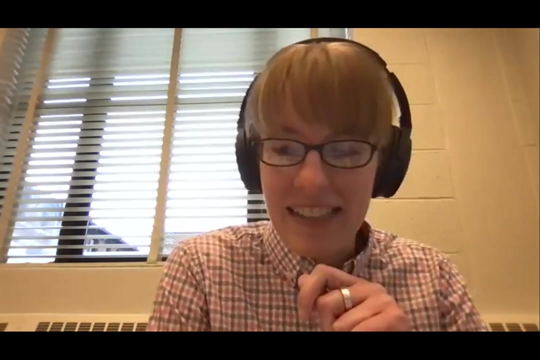 come out of universities. Yeah, I think one part of that- maybe that's just a comment before answering the question on like how do we transfer these into the education setting- is I do wonder. I think there's some philosophy behind the idea of one robot for every task. 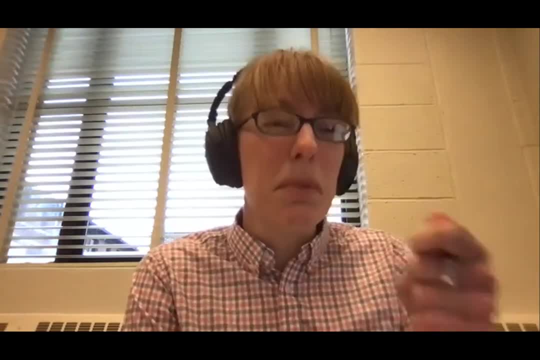 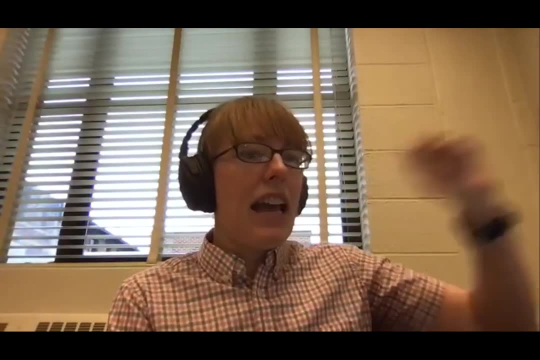 but I think it may also be a limitation of the capabilities of soft robot systems right now, Because if we could, if I could, build a soft robot that made that actuation, that tied itself in a knot and also made you know that shape, that kind of curled itself up and also made this other shape. 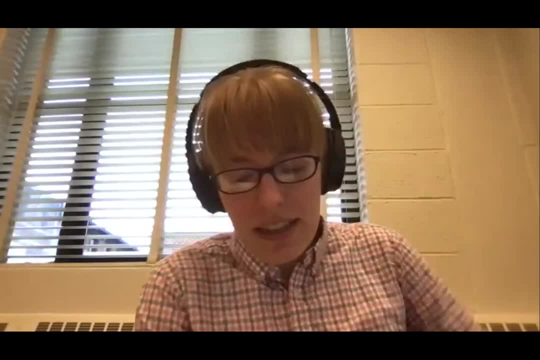 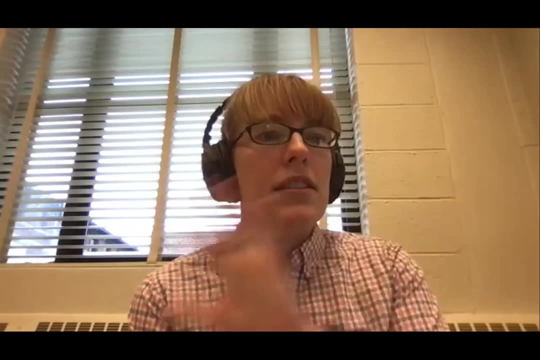 that's probably what I would be working on right now, And maybe I'll get to that point sometime soon. you know we're looking at directions to go there, But at this point there's this disconnect between how many degrees of freedom you can control. 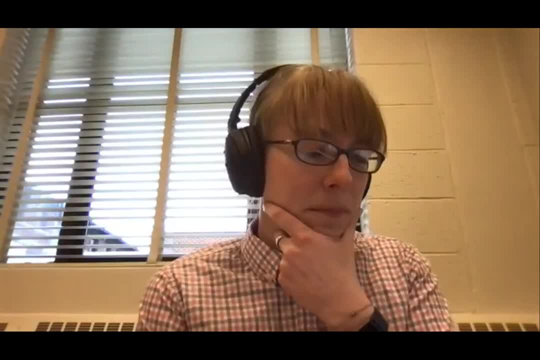 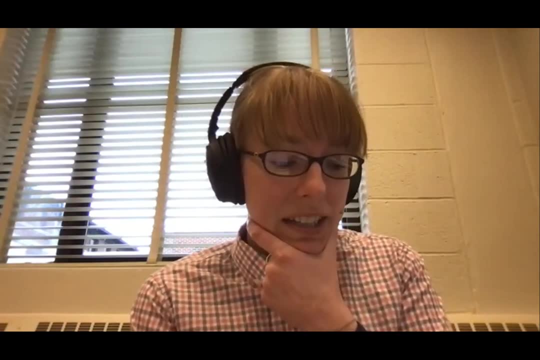 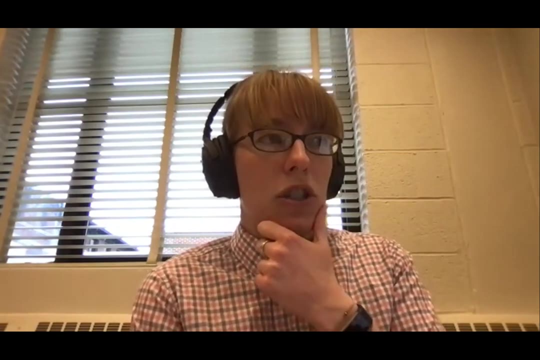 well and how complex your shape can get. So that's sort of one comment on that, And you know I'm interested to see where that goes soon. But what that does mean is that, in my mind at least, this sort of like targeted design is a very interesting teaching tool. 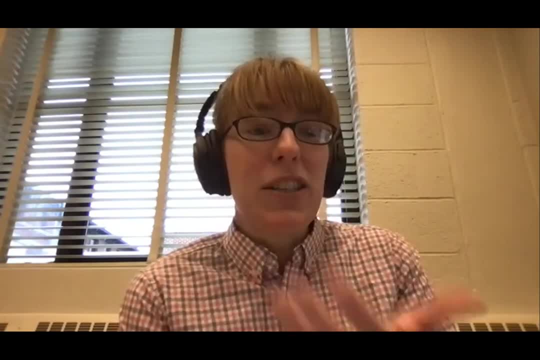 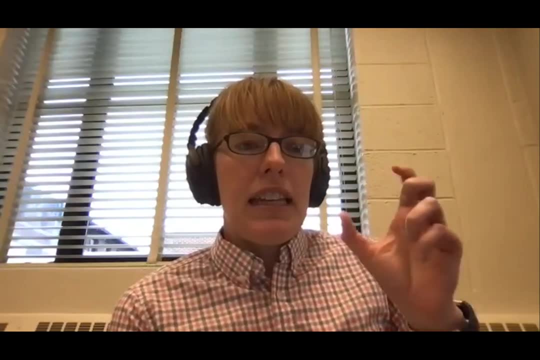 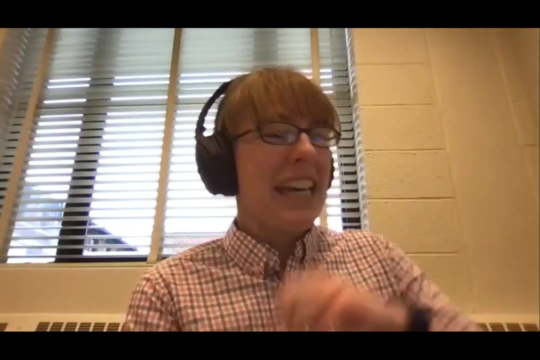 for maybe not for senior design projects, but just for teaching about robotics concepts in general. So you can give someone and you know, teach them how to build a soft muscle or a specific type of actuator and they can model how it moves and they can sort of rediscover kinematics. 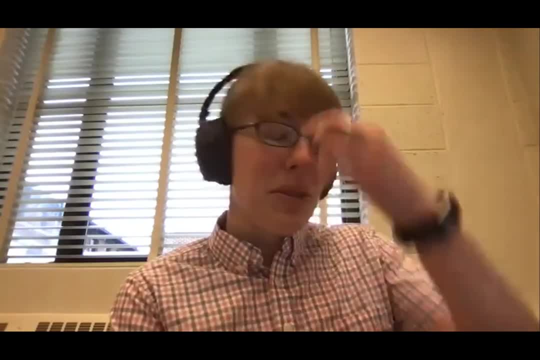 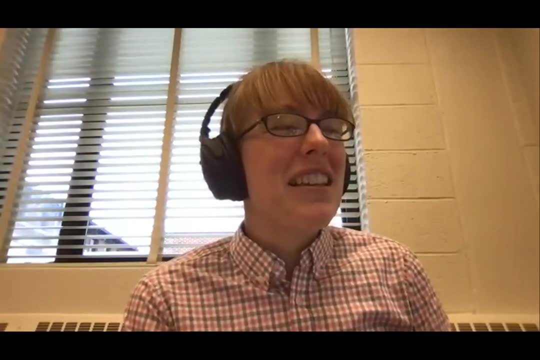 dynamics, force relationships all for themselves. for a robot that no one's built before, right Versus, I think you know. you know, when we're teaching robotics more traditionally, we kind of say: here is the one way it's done. 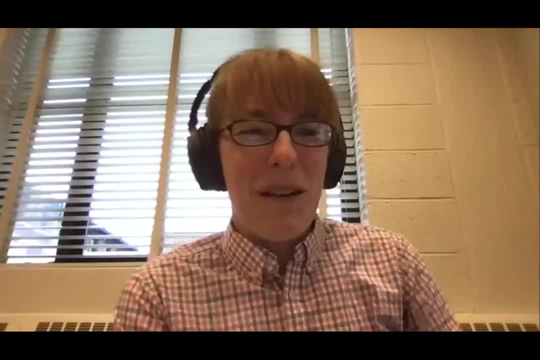 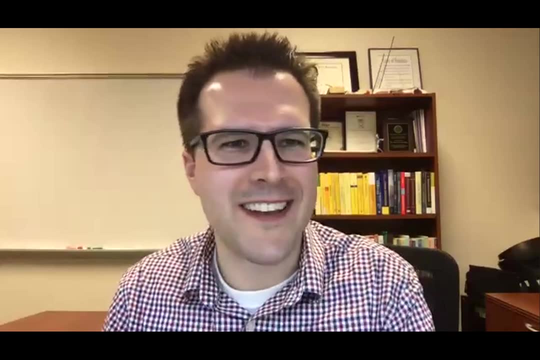 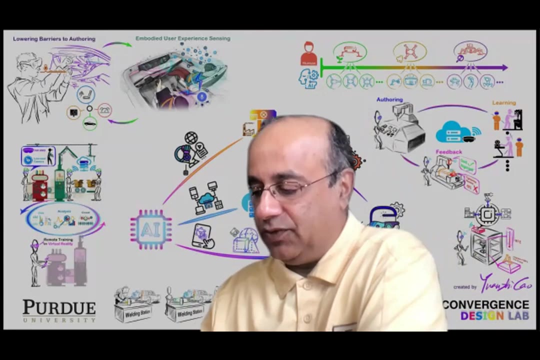 And that's maybe a little less design-focused way of thinking about robotics. at least, I love everything that Laura said. I won't add anything else. That's pretty cool, Pretty cool. So yeah, so we have seen different types of thinking that both of you have expressed in your research. So how do you think? 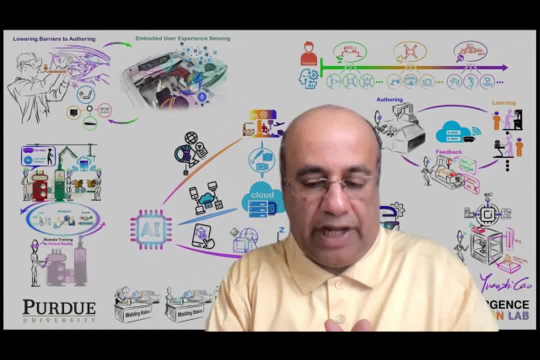 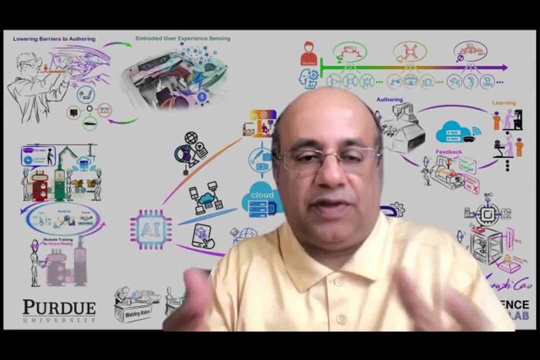 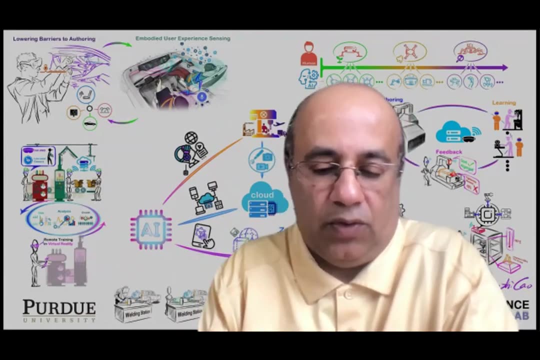 in terms of what you wanna look to see in the future. Well, I think that thinking will change as we go forward with your own research. Or are you sort of happy with your philosophy? I mean, I've seen some implicit philosophy expressed in both your talks. Where do you think your research is going to go? 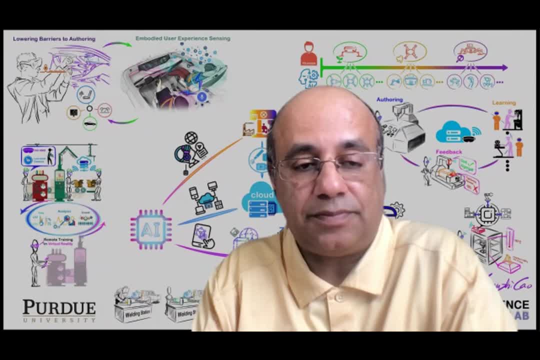 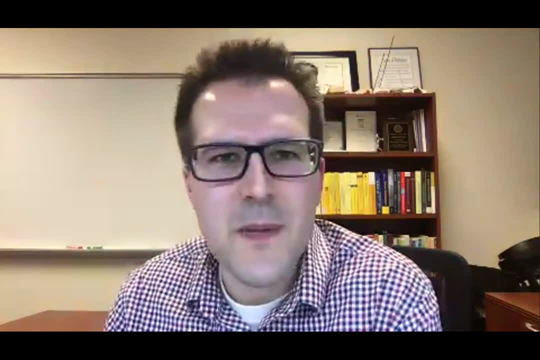 in terms of the challenges that both your areas are going to be meeting. Yeah, So I guess, in terms of, you know, as the field shifts and changes along the way changes, I think we need to be adaptable to that. And you know, we've seen with the 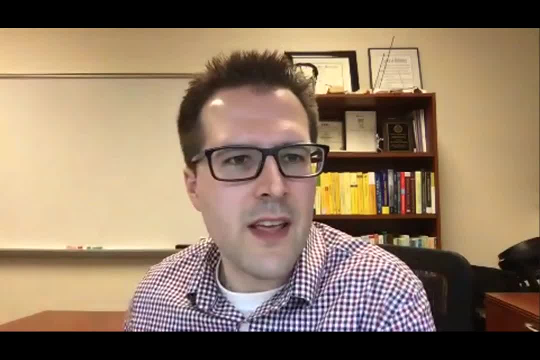 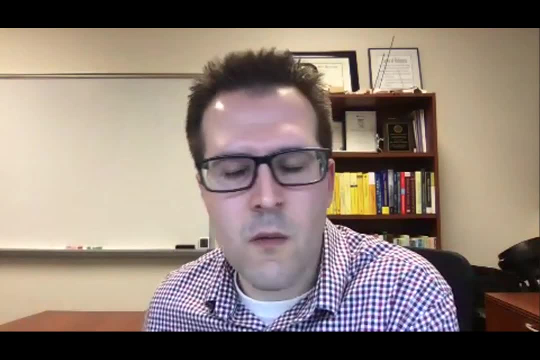 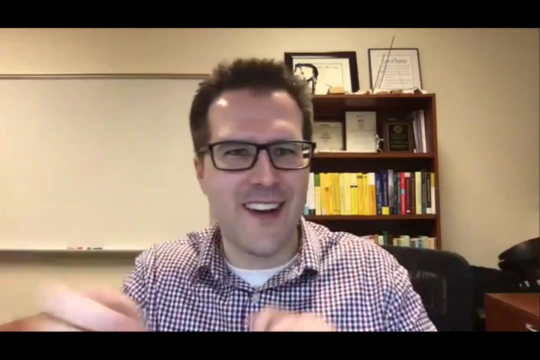 state of the art and quadruped locomotion- locomotion on level surfaces- is getting close to being a technology in the sense that you know, being able to handle very discontinuous type terrain if I'm only allowed to step here and there, as opposed to having a nice paved way. 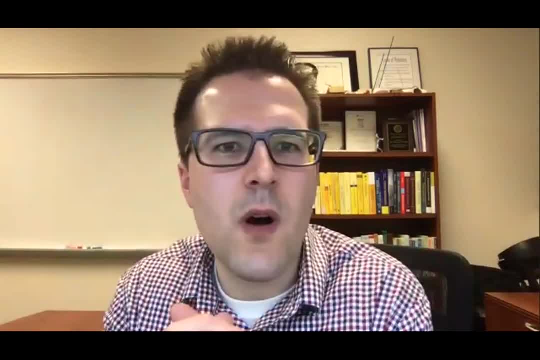 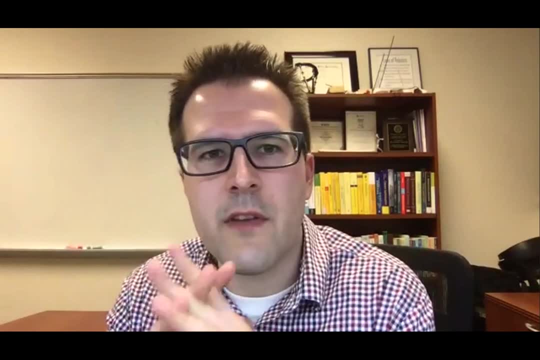 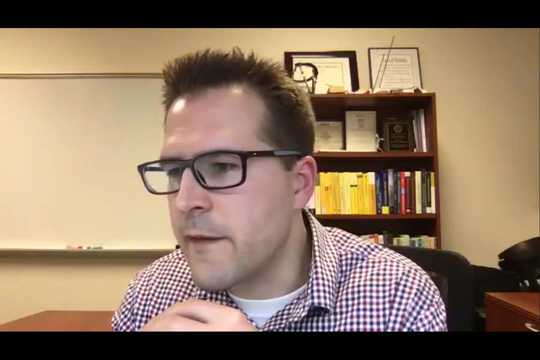 like that's the area where legged robots bring the most value over wheeled vehicles. We haven't seen as much research on that in that direction, And so that's kind of a new area that we're starting to look at. that brings in some new aspects of perception and control in different 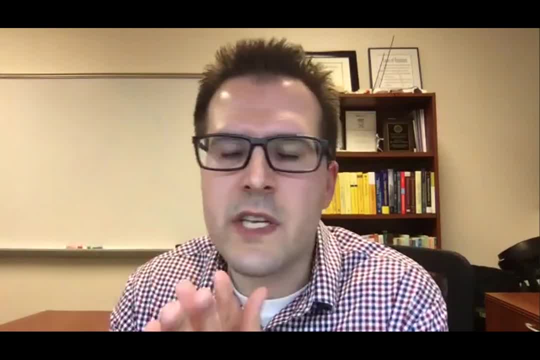 ways On the assistive device side. you know we've seen some really phenomenal open source hardware that we've been. this has really kind of changed the direction of what we've been doing in the past, And so I think it's really important to look at that. 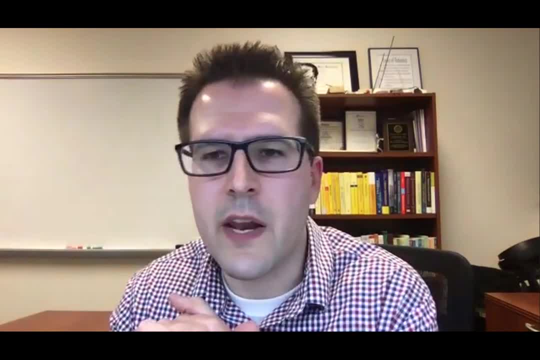 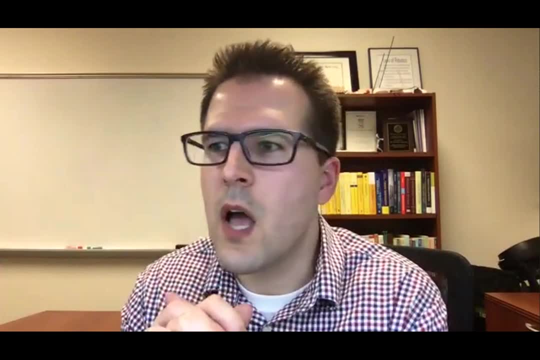 been doing in the group, shifting a little bit more to prosthetic legs as opposed to focusing as much on exoskeletons. And then I think you know we'll continue moving in that direction, just due to the access and then also the impact that we can have due to the communities that are. 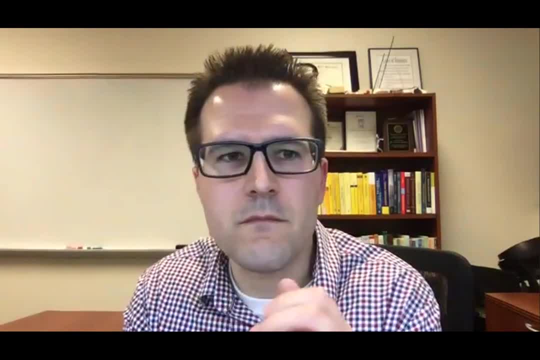 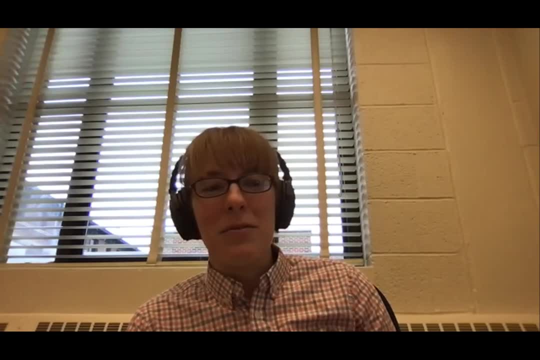 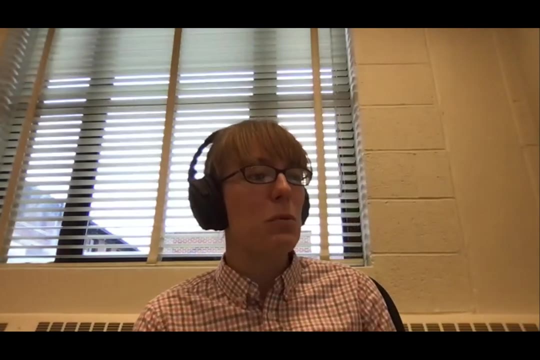 rallied around these open source platforms. Very cool To answer from, I guess, the soft robotic side. I think this is in the points that we've been talking about. you know the disconnect maybe between traditional robotics and soft robotics. That's where I think I see the 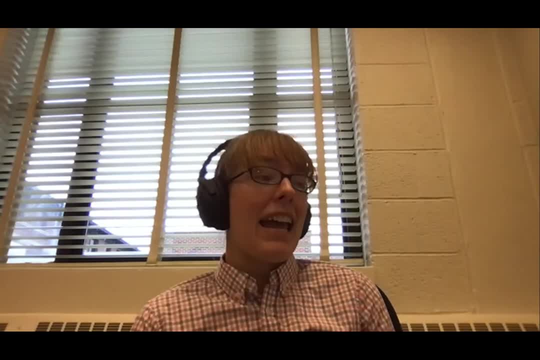 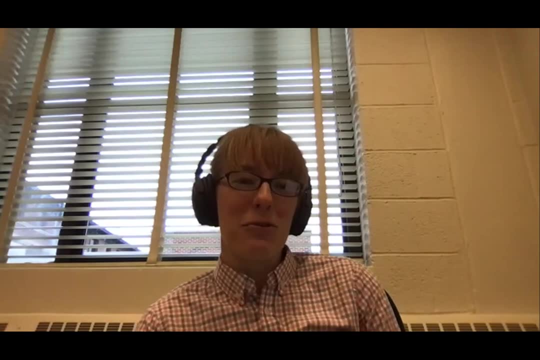 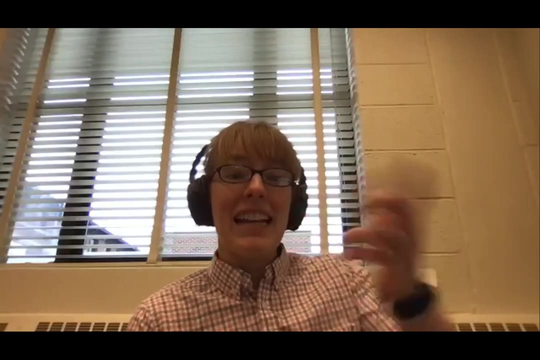 most interesting problems in the future of the field, And that's also where I see, you know, there might be a lot of hard questions in terms of what is a good soft robot coming in the future? We've made lots of cool soft robots, but now I want to make good soft robots And I think to 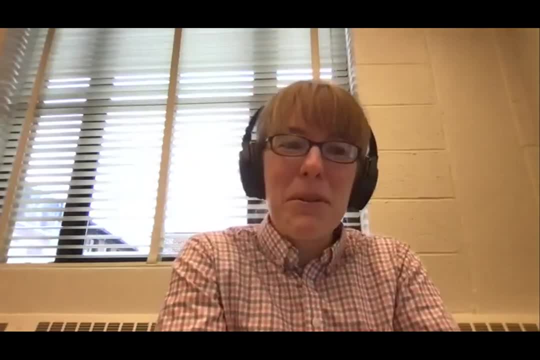 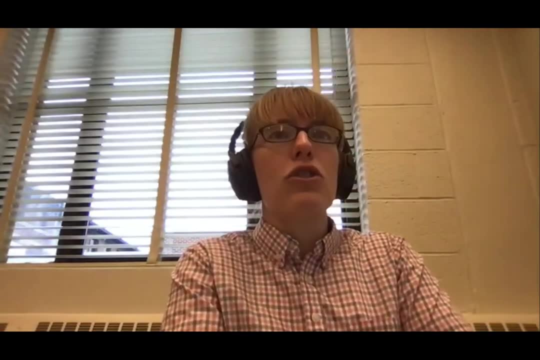 earlier questions. the example of the grippers is perhaps the most interesting. I think the example is perhaps like the most quintessential example we have right now where soft grippers are positioned, where they are solving this really difficult manipulation problem in a different way. 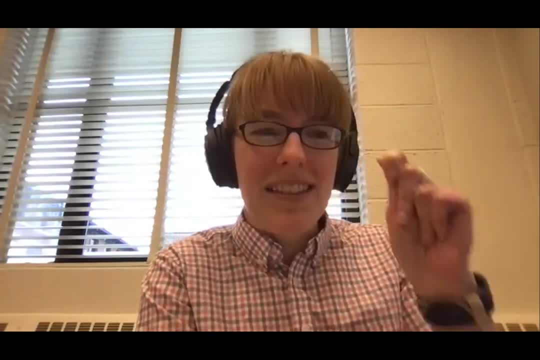 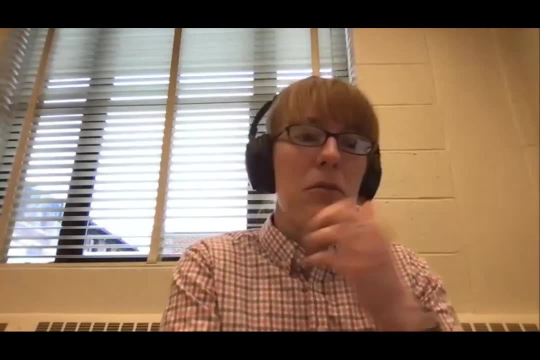 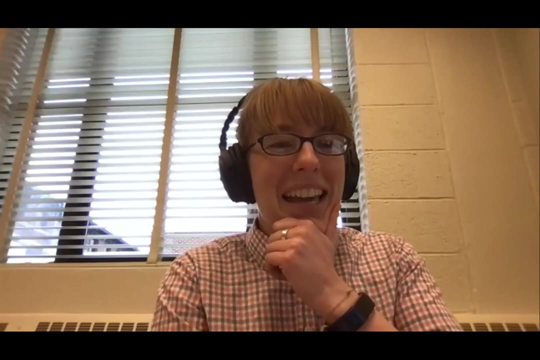 and using the exactness, the preciseness of traditional robot arms to kind of overcome their limitations maybe. But you know, they might be overtaken by better manipulation technologies on the rigid robot side at some point in time. So yeah, to put it in a sort of 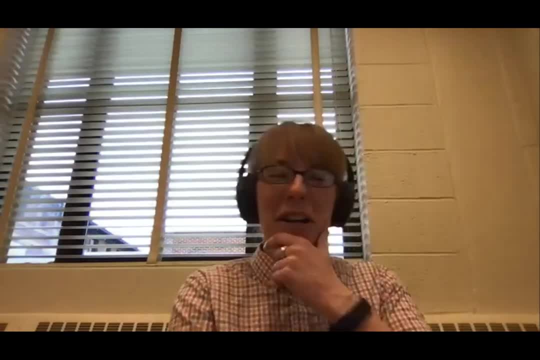 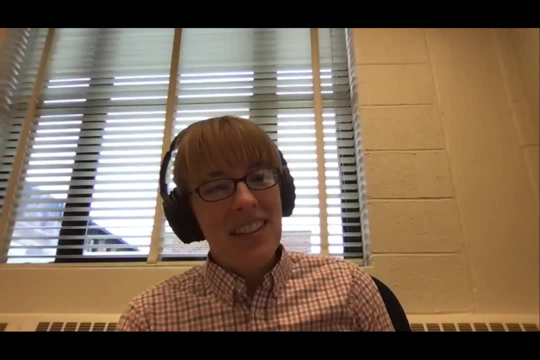 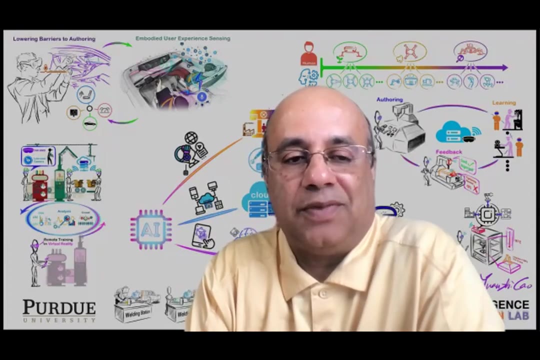 Kurt Blythe way I want to see good soft robots and soft robots that are kind of out there doing interesting things. Yeah, Very cool. So thank you so much for both your talks- Very inspiring and very cool work. You know you're the rising stars of the future, So I want to give the 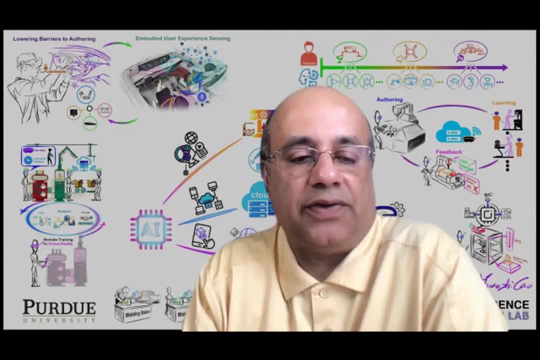 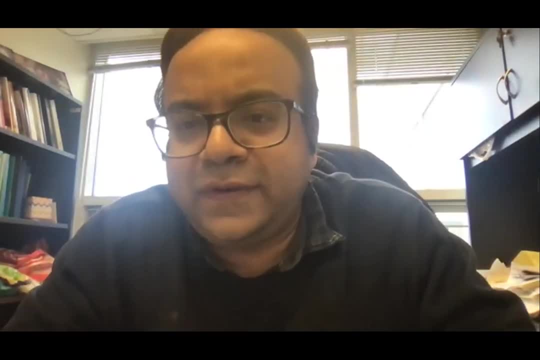 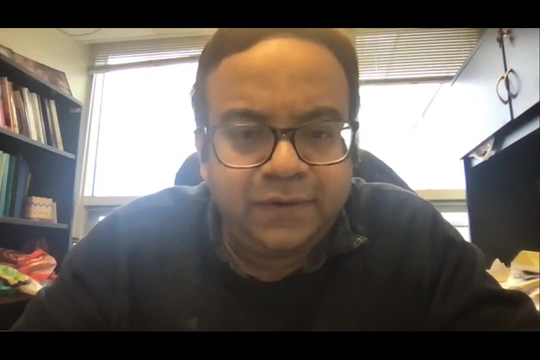 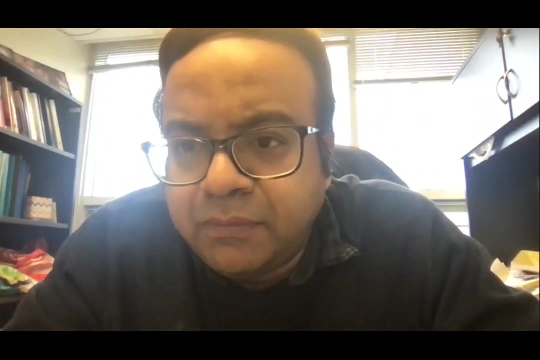 podium back to Sid and Partha to close up on this session, I mean before. I mean there are like significant number of questions from the audience. I can see them in the chat box So I can maybe pose a few questions to the speakers here. So one question I see from Margaret. I don't see. 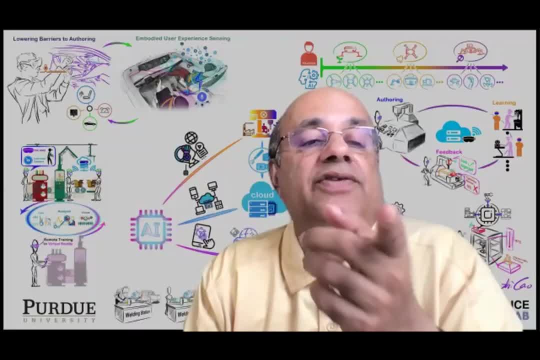 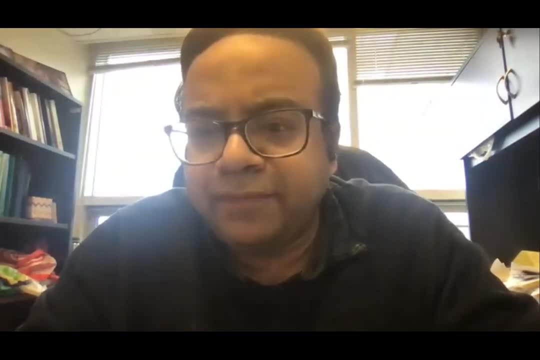 if Margaret is around. Yeah, I think both were asked already. Okay, So any more questions. I don't see any other question. Patrick, did you have a question? I don't see any other question. I don't see any other question. I don't see any. 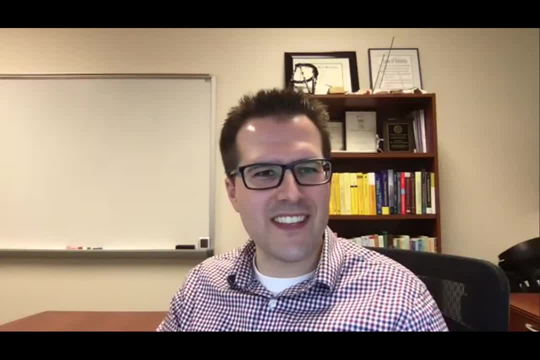 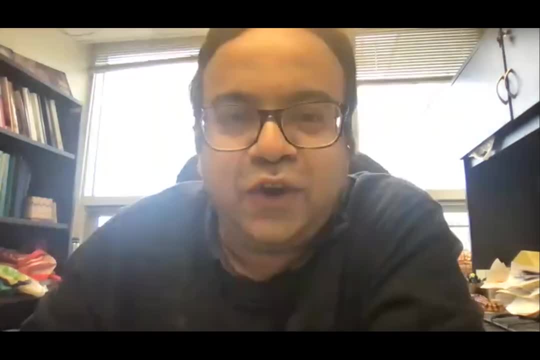 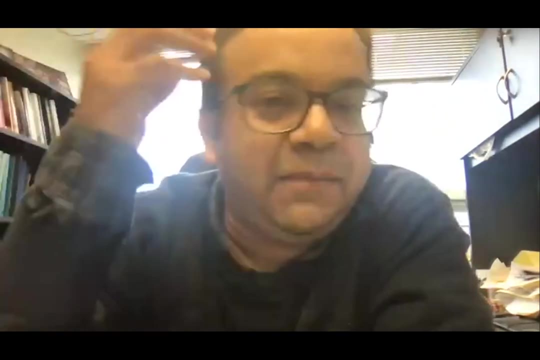 probing question. Yeah, I did. So I have an interesting, I mean, I have a kind of a take that comes from somebody working on more at the interface of the chemistry and biology and things like that. So one example that, Laura, you showed, where you showed that one soft robotic: 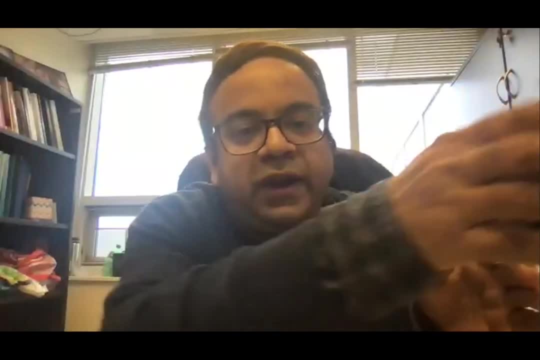 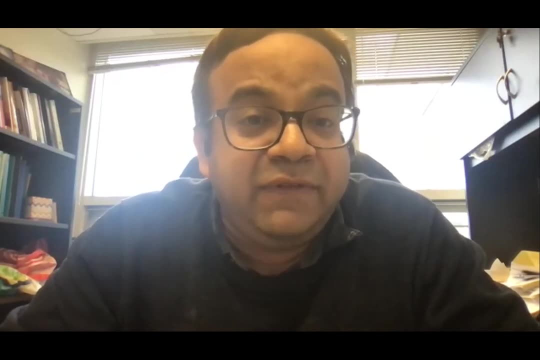 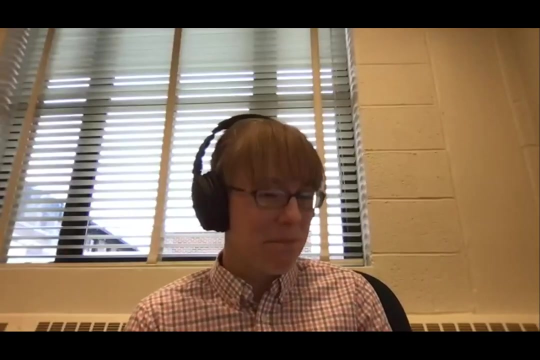 arm, if I may call, or an appendix around right Now. imagine if I am using that to model an actual biological problem in vivo. In vivo, Yeah, There is a lot of chemical signals going on. Yes, Yeah, The entire thing that you captured is basically a mechanophysical issue. 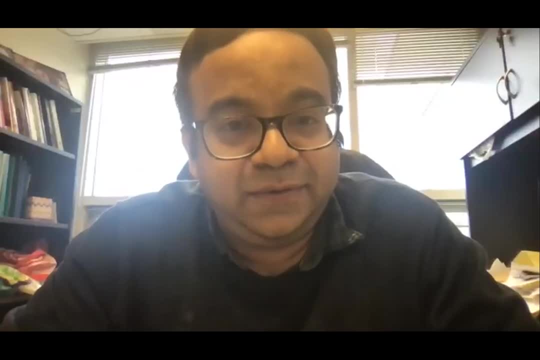 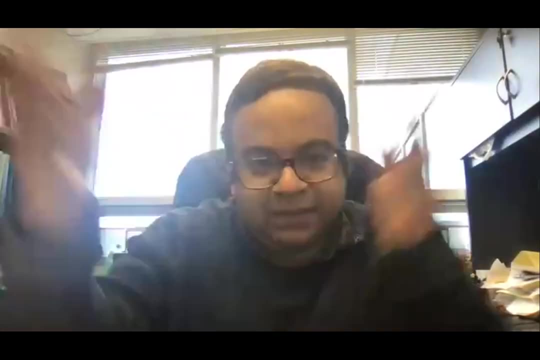 What? how do you account for the chemical issues? Yes, This is between the- let's say, let's say that- appendage. is there maybe? Yeah, Something like a yeah, How do you talk about it? Yeah, So so this is an incredibly interesting question when we talk about software. 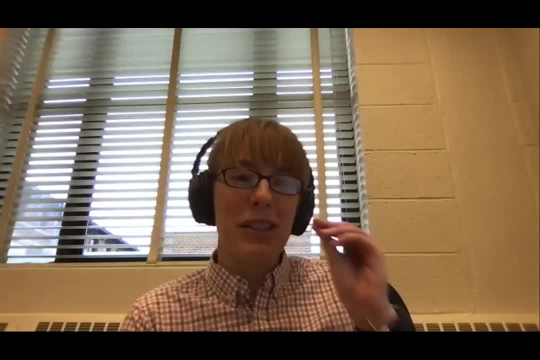 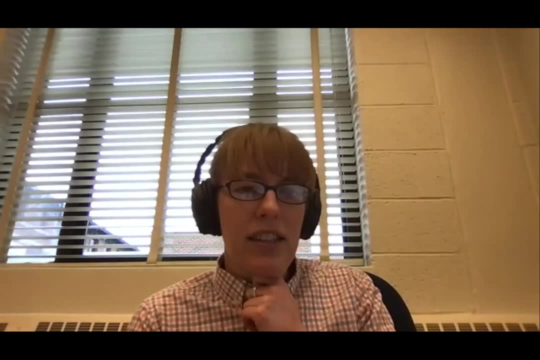 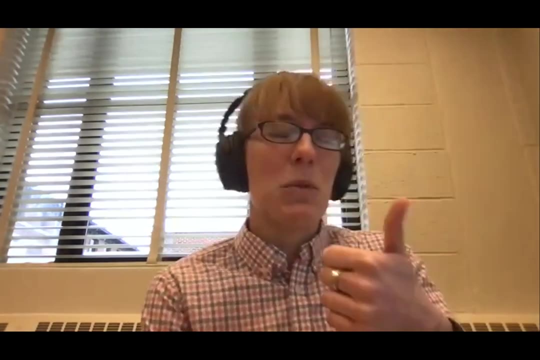 robots as like analogs for biological systems, which I think is a very, very interesting application of both robots, but but soft robots specifically, And- and this is where I think some of that language of like imitation breaks down a little bit, because we're, you know, maybe taking 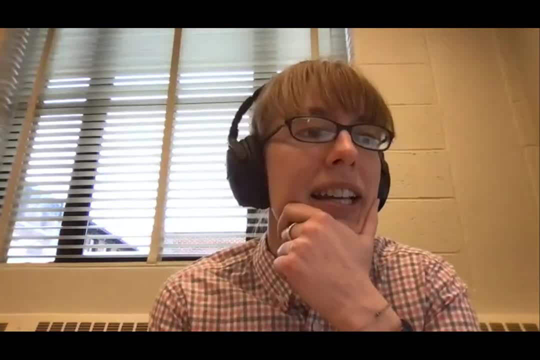 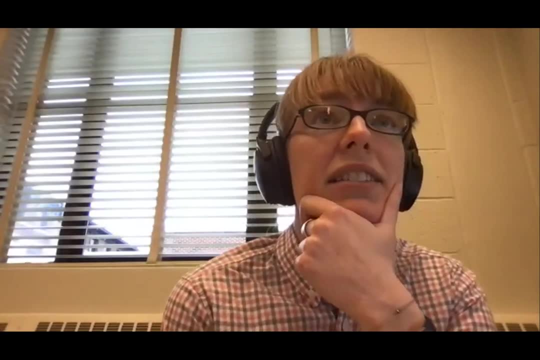 more inspiration than imitation in some ways. when we do that. Now I do think there's ways to to kind of get at that, but it's sort of a question of what? what scale do you want your imitation, your inspiration to be at? If we want to imitate, 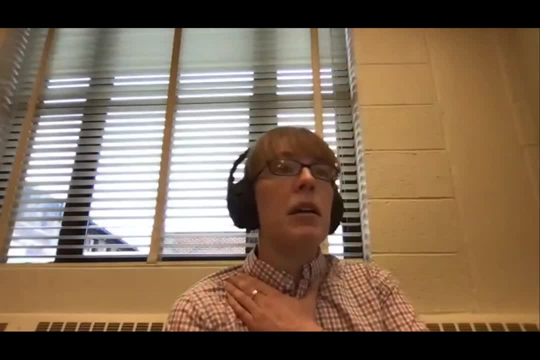 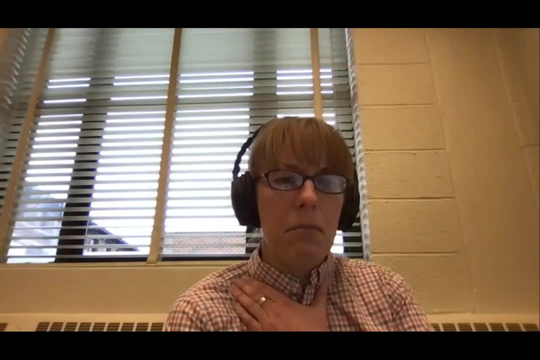 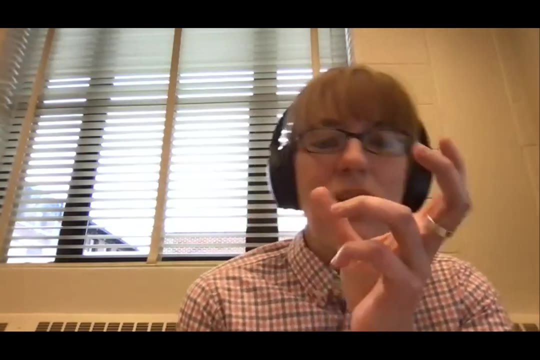 these chemical signals not work that I've been working on, but some researchers at, I believe, IIT in Italy, Barbara Mazzoli, has been doing some plant inspired robots that actually do things like tropisms, like they follow the sun or you know other things like that. 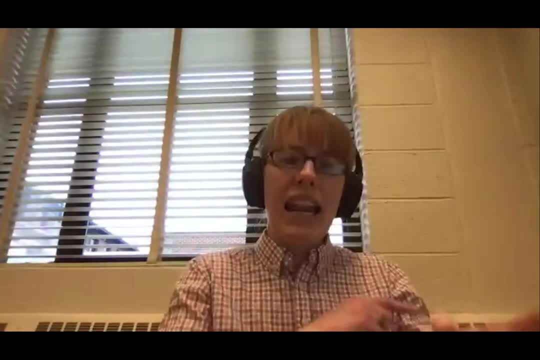 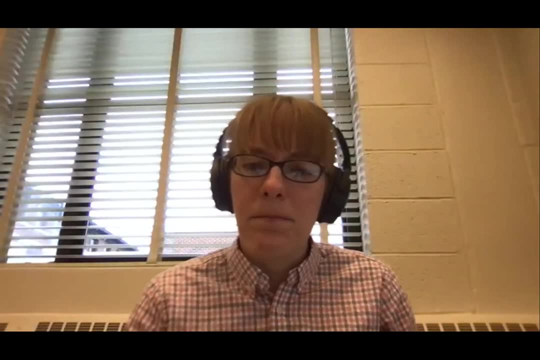 So they're not getting at these chemical reactions, but they are getting at the behavior, The behaviors that come from the chemical reactions, which you know is is an interesting thing in of itself. Yeah, Like like one example, I mean I I think, I think Karthik has posed a very interesting. 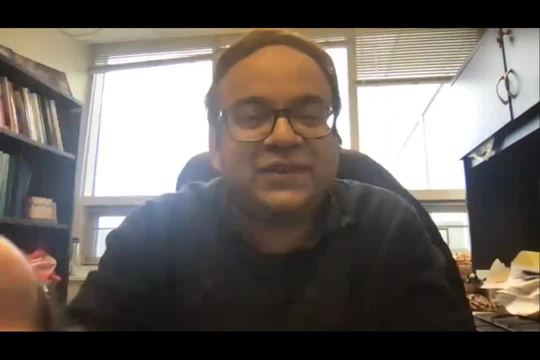 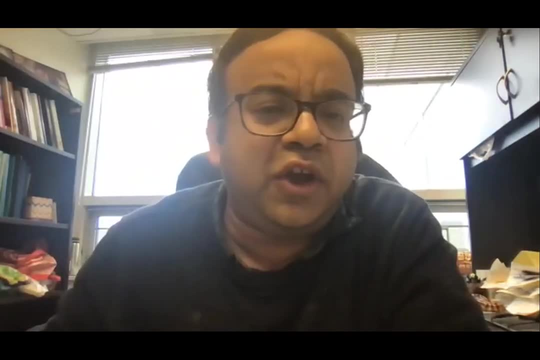 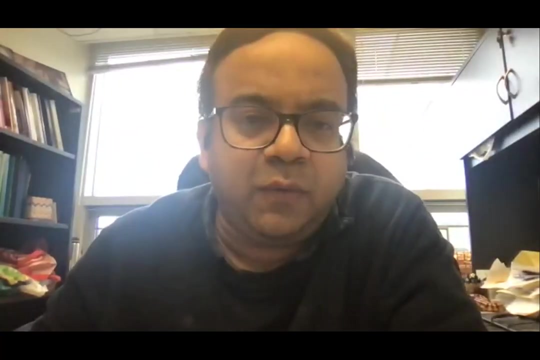 question where you would. you are requested to ask one question to each other, but before just just one comment. So I had some prior experience of working on biofilms like bacterial biofilms, So bacterial biofilms. people have been doing quite a bit of work. They 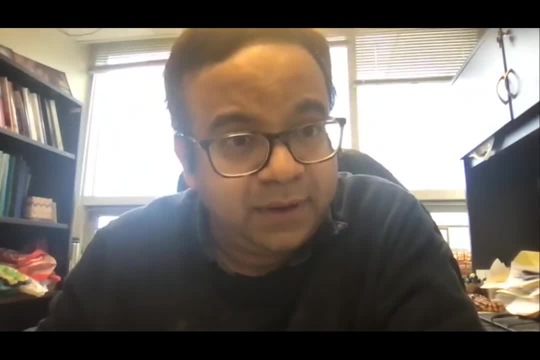 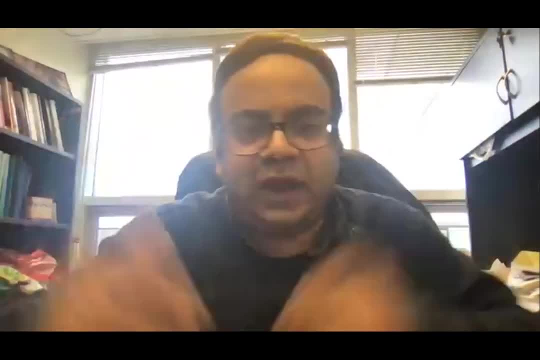 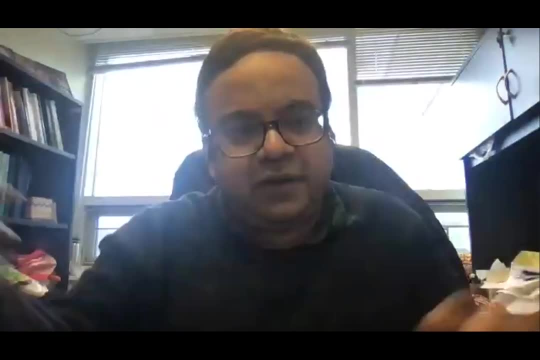 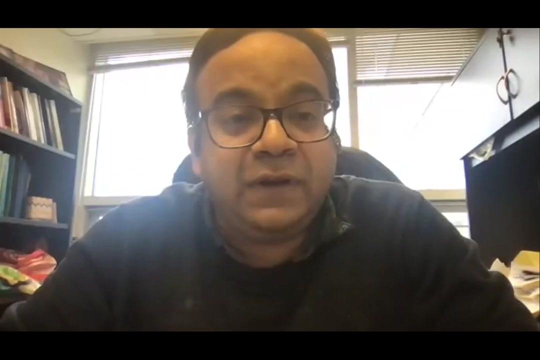 kinds of biofilm streamers they form. I I developed some equation on bacterial biofilm streamers. What hasn't been there, for example, this biofilm? I mean your picture, Laura reminded of me of the bacterial biofilm streamers. that what happens if you have this bacterial biofilm? 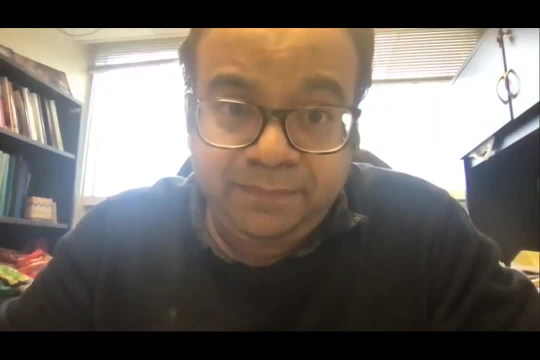 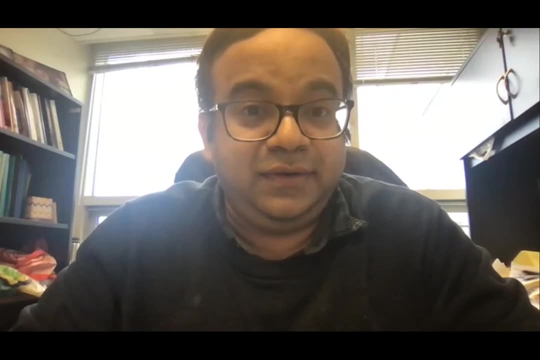 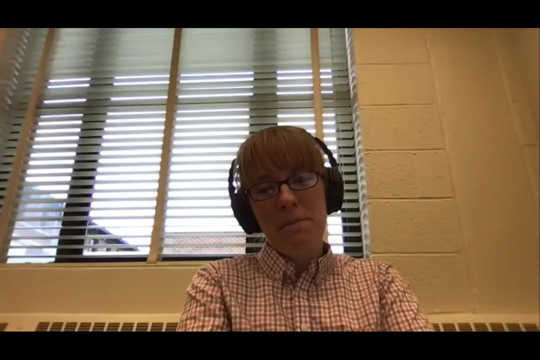 streamers growing in a bacterial colony, in an active bacterial colony, Yeah, Where there are living bacteria moving around, And then you have this kind of appendage like structure going on- Interesting, But there the bacteria themselves keep on secreting this kind of they call it extracellular polysaccharide. 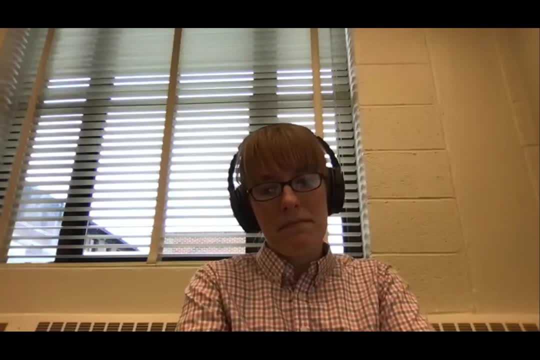 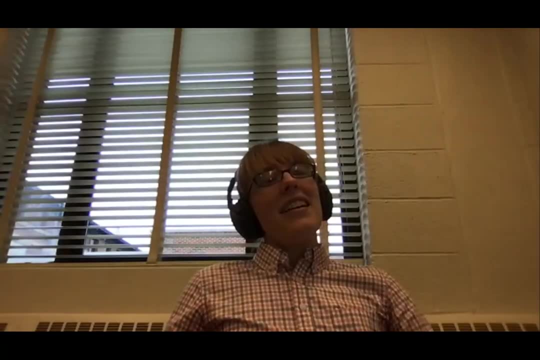 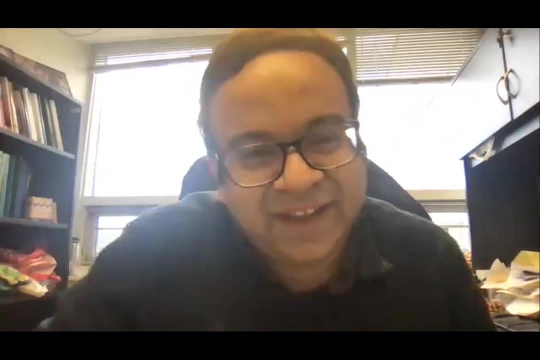 EPS And in the process they exchange this chemical interactions between them- A very difficult problem, Yeah, Yeah, But maybe something you can think about. Yeah, Yeah, I think this comes down to- yeah, a lot of multi-robot systems as well. It's very interesting. I'll have to think about that. 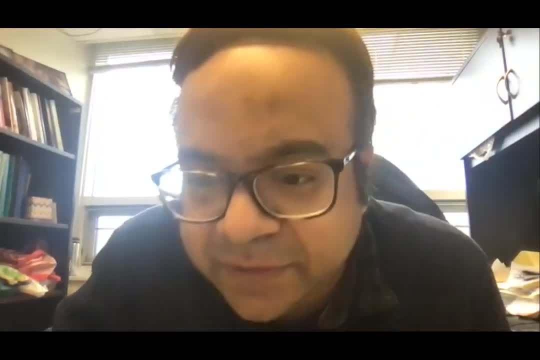 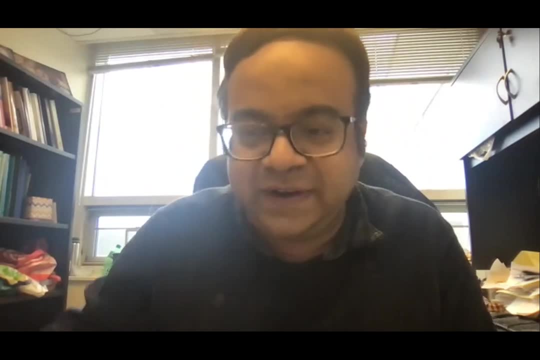 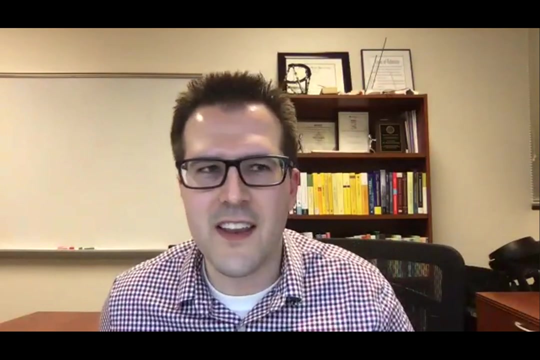 more. Yeah, Yeah, I will stop here. So I think there is one very interesting question that Karthik has posed. Yeah, So, like Patrick and Laura, you can each ask. you can each ask a question to the other. Yeah, I guess, with whatever time we have left. So, Laura, you know, I mentioned 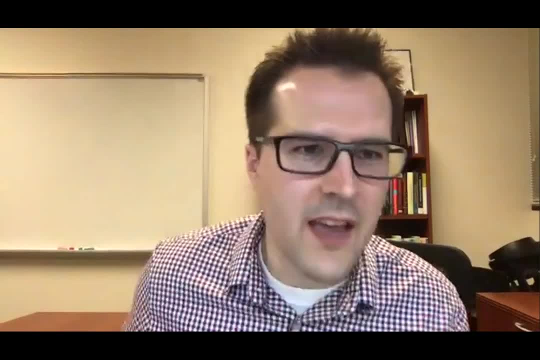 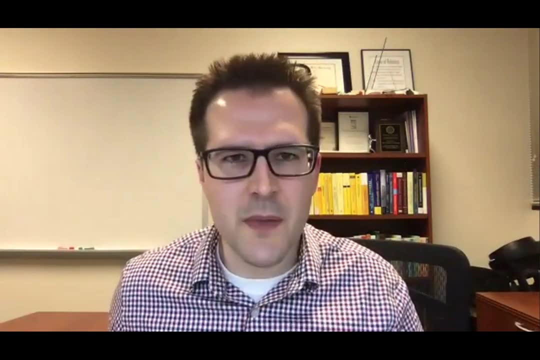 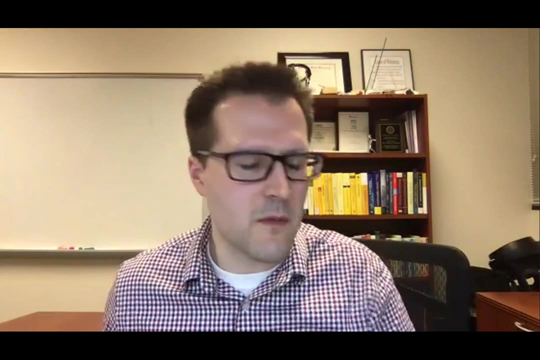 this co-design work that we'd been doing and essentially what we're we'd been trying to do was is to come up with a way to design to maximize morphological computation, Like that's kind of the the goal. But then if you're going to formulate some design automation or design- 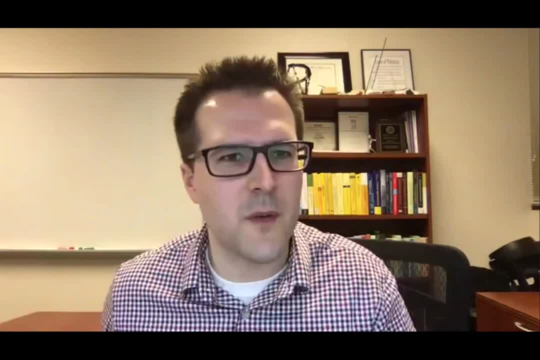 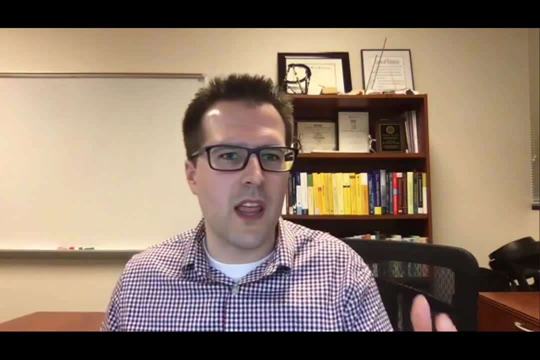 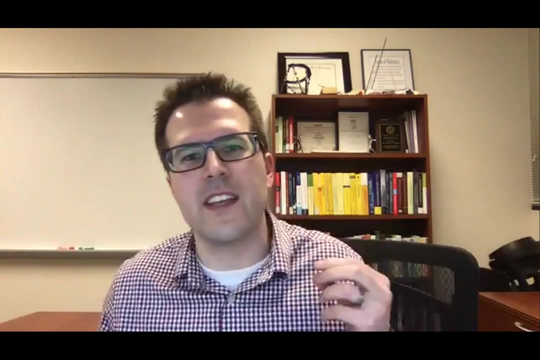 optimization problem. you now have to come up with some metric for morphological computation. Yeah, morphological computation is this thing that like we know it when we see it, but like I don't, it's. it's very nebulous in terms of actually saying what it is and, in particular then, how to quantify it, And so I'm 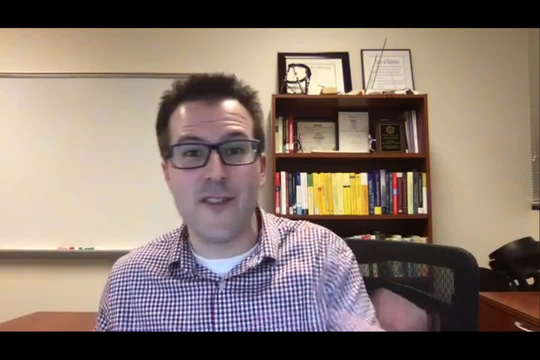 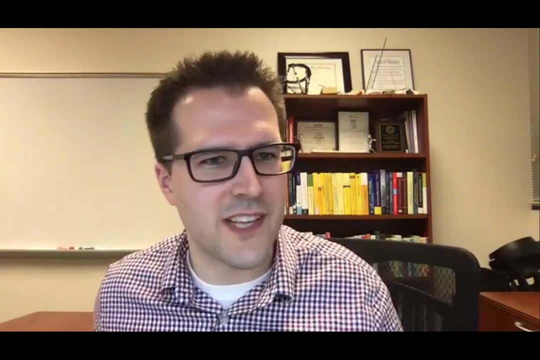 curious. I'm asking you this, this question, under the condition that I have no idea how to answer it. Do you think you know, are there good metrics of it, Or do you think it's foolish to try to metricize it? Oh, that is a. that is a wonderful question. Um, I don't think there's good metrics. 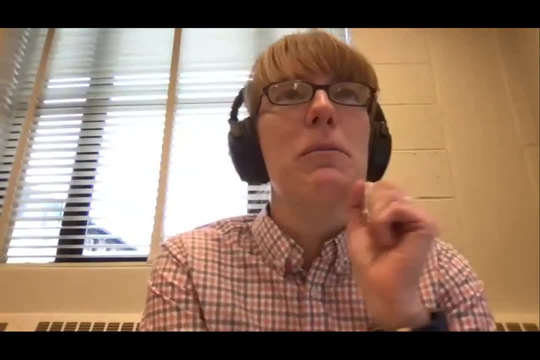 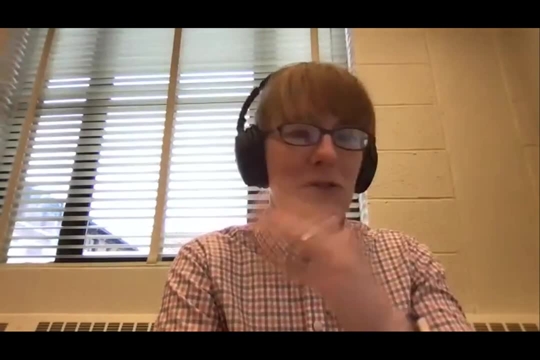 for it. yet I definitely you're right, And it's that this you'll know it when you see it sort of thing right now, like I use that word for that second thing I talked about, that's like morphological computation, but very much in that, like you know when you see it, what I think. 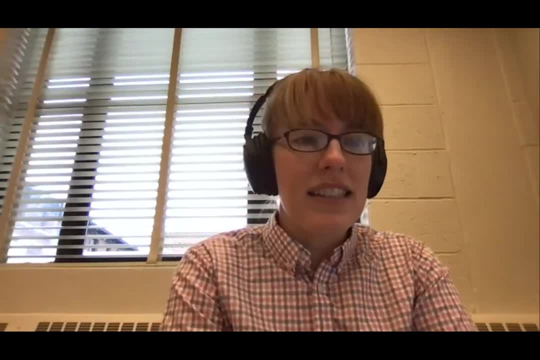 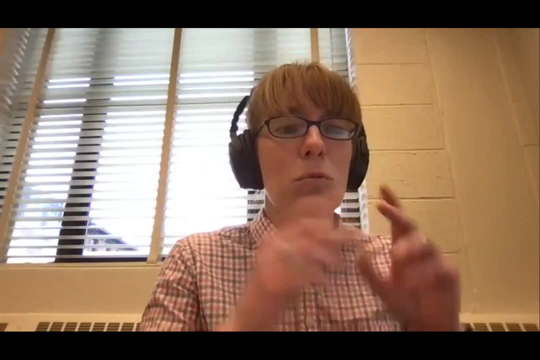 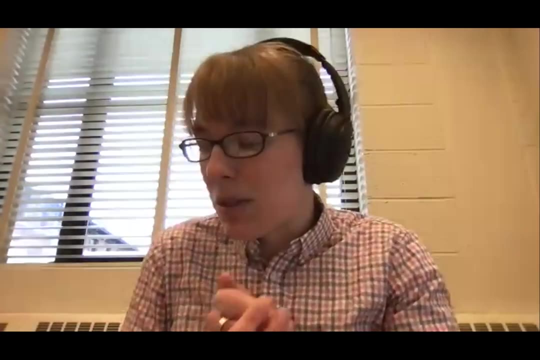 is is sort of needed is: yes, this idea of how do we know what counts is like an unknown environment, because that's like the big thing for morphological computation is: what inputs are you going to put in for how your environment can vary And then what behaviors do you want it to do as a result? 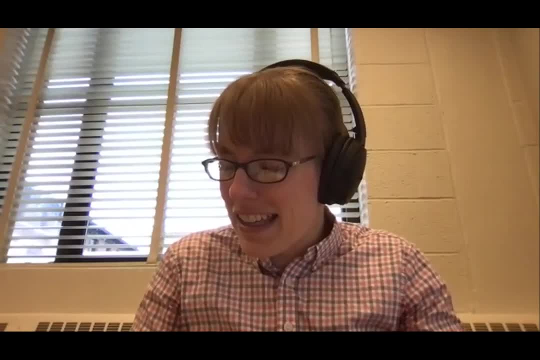 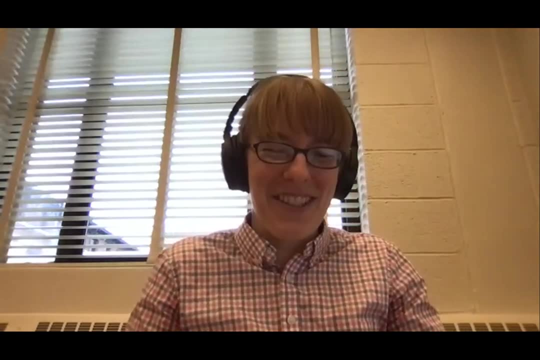 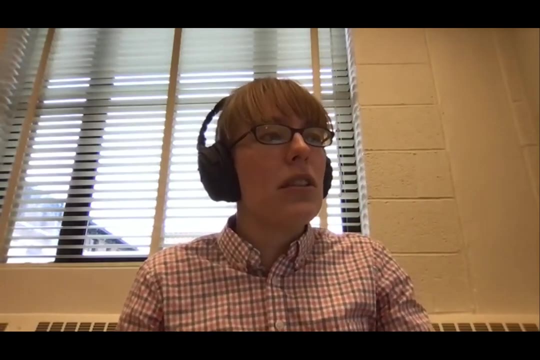 Um, and so I? I don't. I would be optimistic, And I don't think we should give up on the ideas of morphological computation, as you know, as as probably an achievable design goal just yet. But that's certainly you know. the. what you're talking about of, like, defining your outputs, is sort of the the. 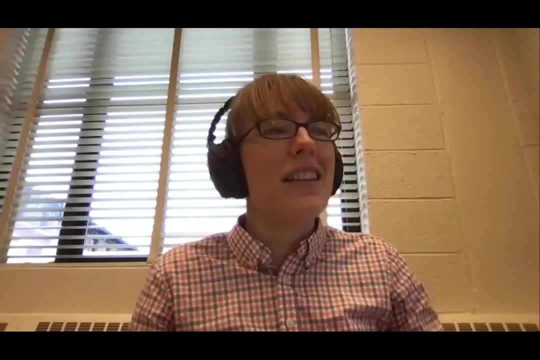 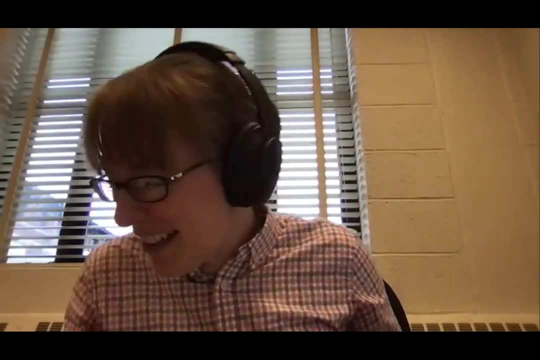 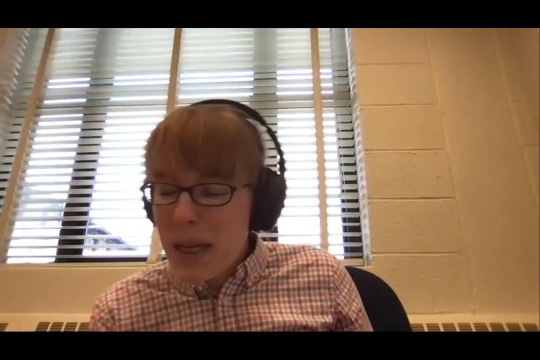 best we've got right now And I'm interested, Yeah. So I think it's an interesting question to think about, like, how do we get past that Which does actually go in? I had a question written down That I thought of when, when you were talking, which is maybe in the same sort of lines: But what? 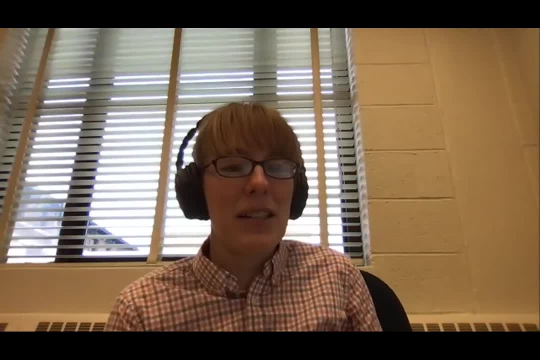 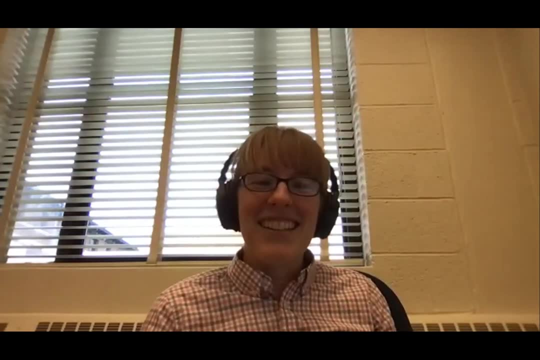 like what counts as a disturbance when we're acting, interacting with an unknown environment, Like how? how do we define like a disturbance versus like just what we're expecting to see? Yeah, I mean, I guess the somewhat of a cop out answer would be anything that's not in our model. 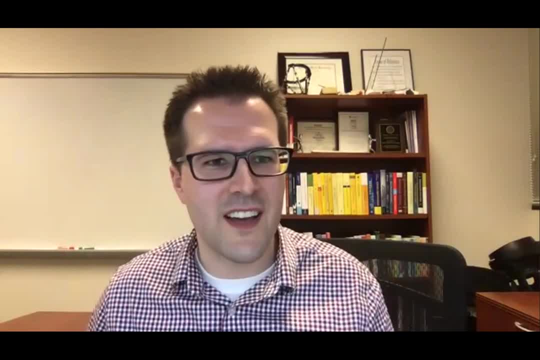 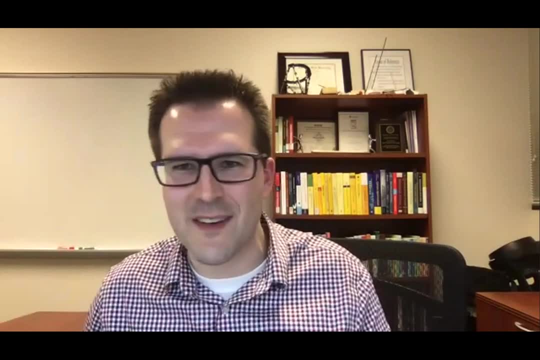 But there are so many things that are not in our model And I'm you know, my friction at my joints is going to be a disturbance because it changes with temperature, And I haven't modeled that And I don't think we should model that. And there's. 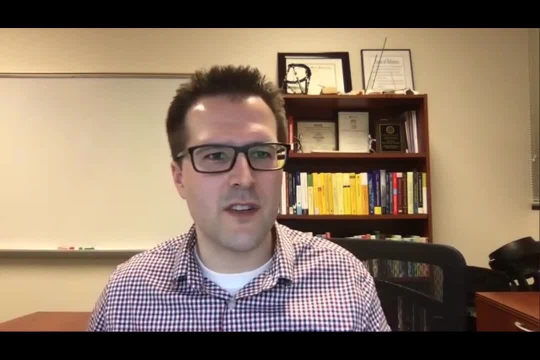 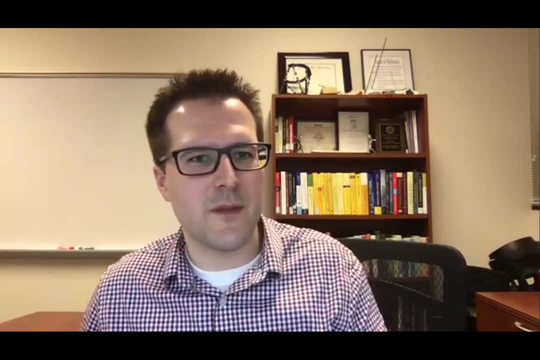 yeah, so there's like self disturbances and external disturbances from the, from the environment. And you know, even we're modeling the environment is rigid, but our environment is not perfectly rigid, And that's that's a disturbance, And so I'm very liberal with 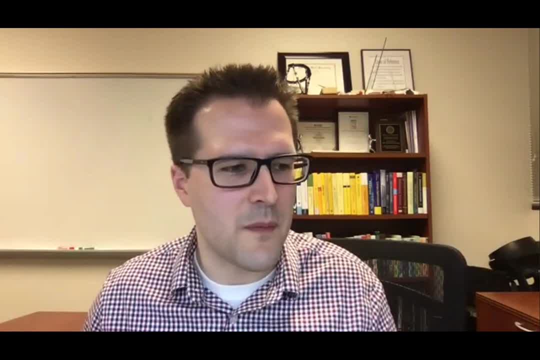 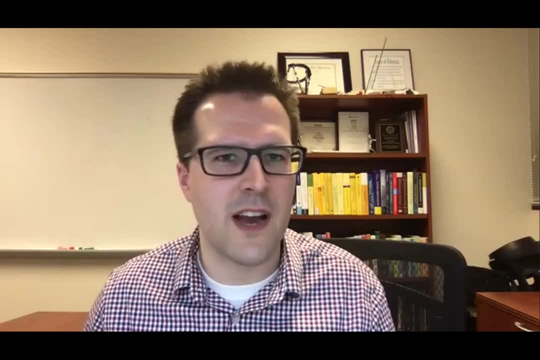 what I consider to be disturbances. It's, but again it's very hard to predict And I think it's very hard to kind of capture the the full envelope of those when you're you're thinking about designing these controllers off board, which I think you know kind of ties into your 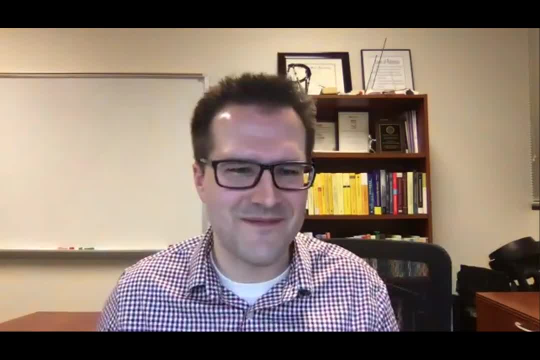 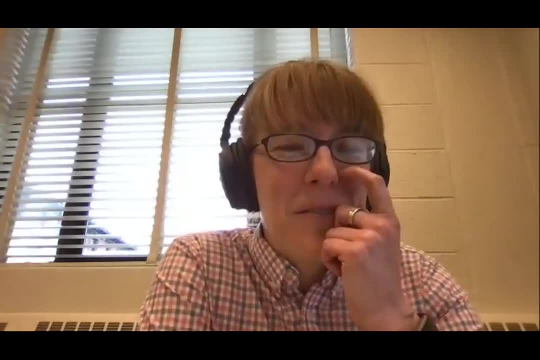 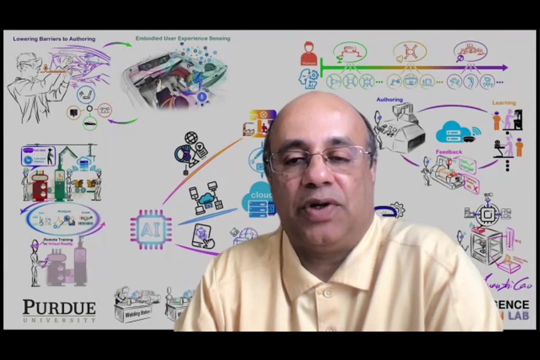 response of what's hard for quantifying morphological computation. So, yeah, yeah, well, yeah, it's a good question to think about, regardless from both sides of both sides of this, this sort of discussion. Yeah, perfect, Perfect. Thank you so much, All of your time And Partha. 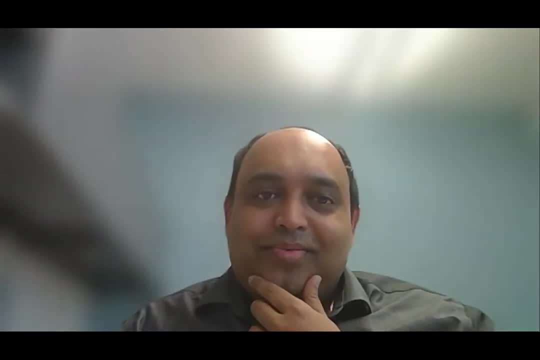 are we good to close now? I think so. First of all, thank you all very much. Wonderful talks as always, and also, Karthik, thanks for touring this beautiful conversation. The conversations after that, typically it just, you know, takes over, So I'm so glad to see that happening again and again, And now both.